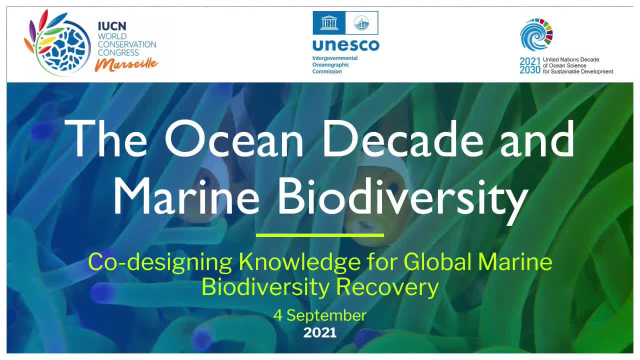 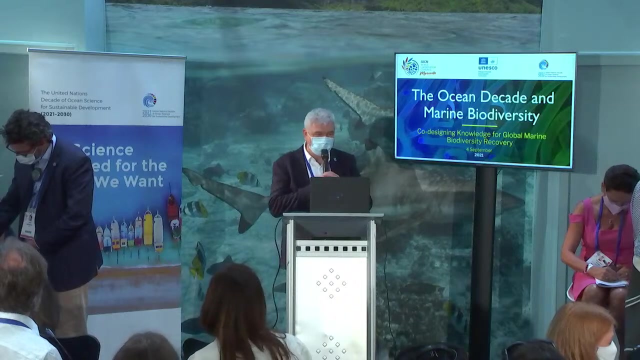 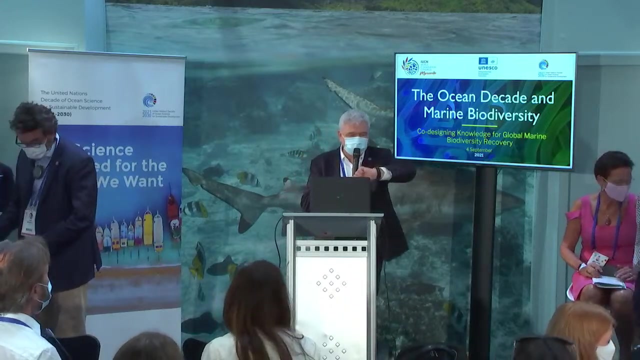 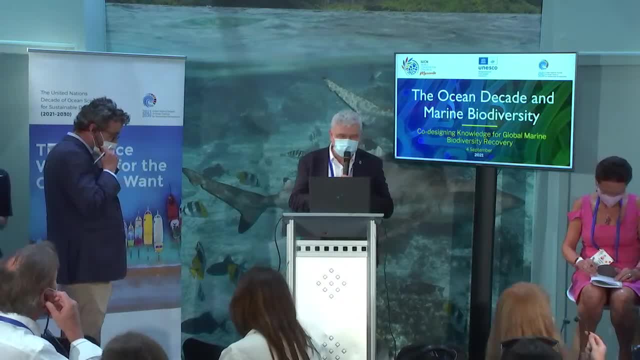 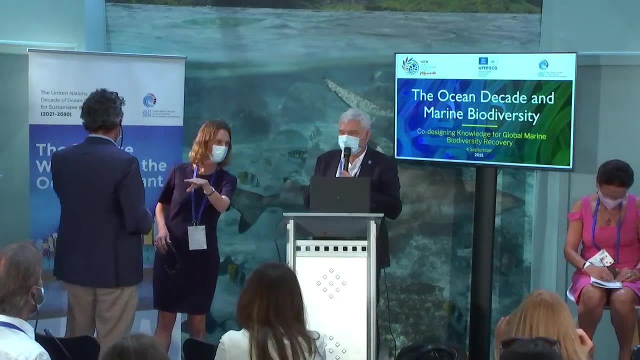 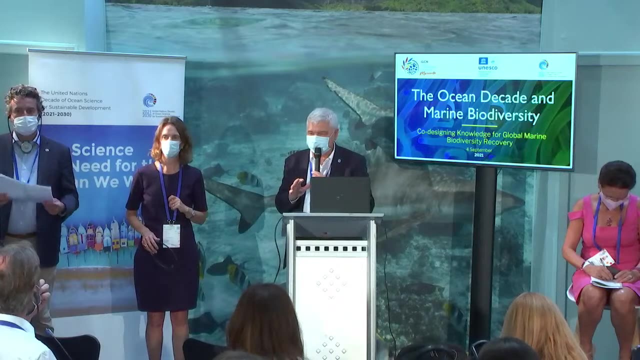 i call it marathon because we have several excellent speakers with us and i would like to take you to what we're going to do. uh, so do you hear me please? you know, please, uh, show, show your reaction. you know, do i have to restart? oh my god. 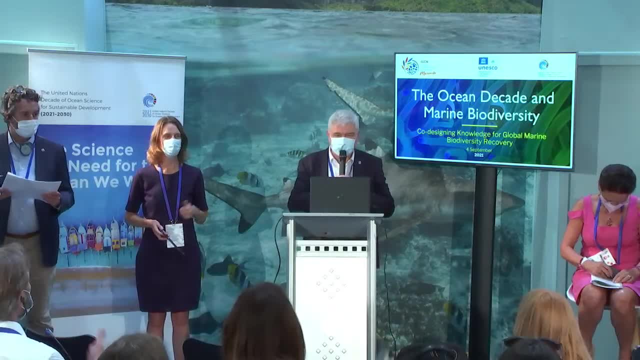 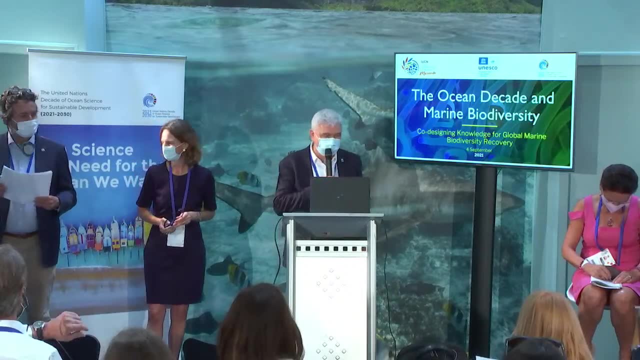 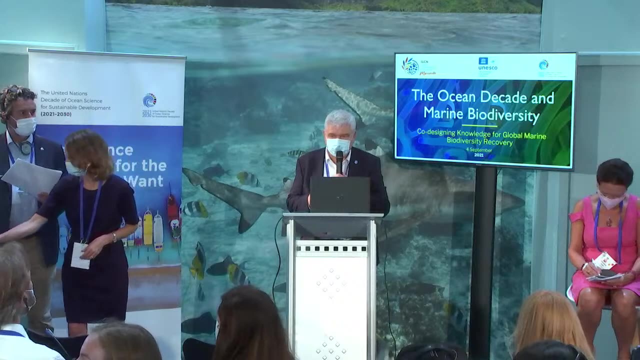 this shows once again the importance of technology for achieving our goals. okay, summed up, all right. so now it is, uh, two hours and one minute. so, uh, we are going to start a session that will focusing on the decade of fortune: science for sustainable development and how it's going to address. 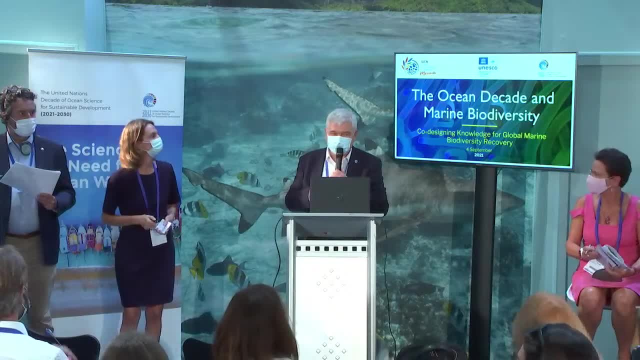 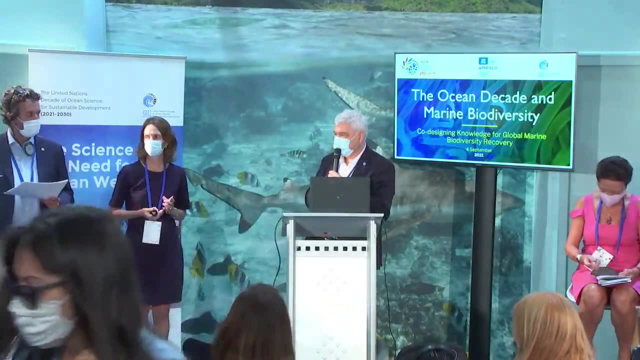 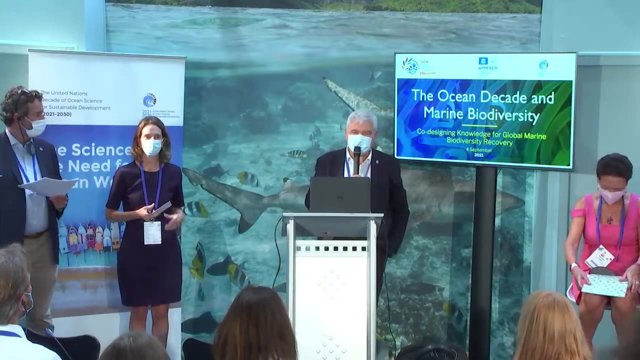 ocean biodiversity. oh la, la, la, la la. so thank you for your reaction and your understanding. so you know, i need to keep speaking, i think, because otherwise you won't be able to to understand the difference. so, uh, when, as soon as i see your reaction, i will start the whole thing. 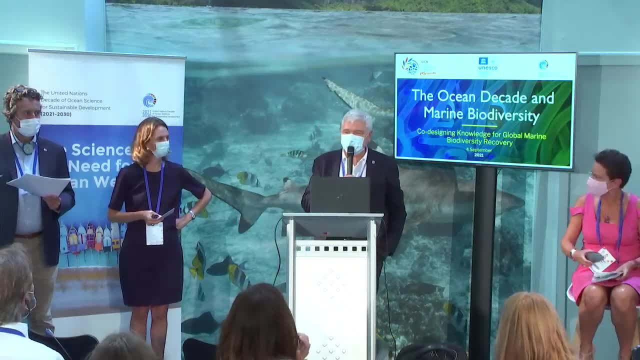 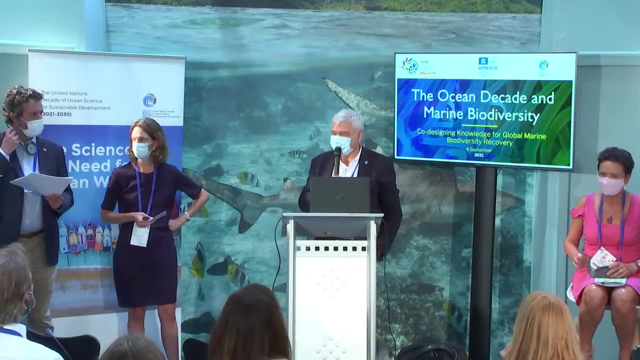 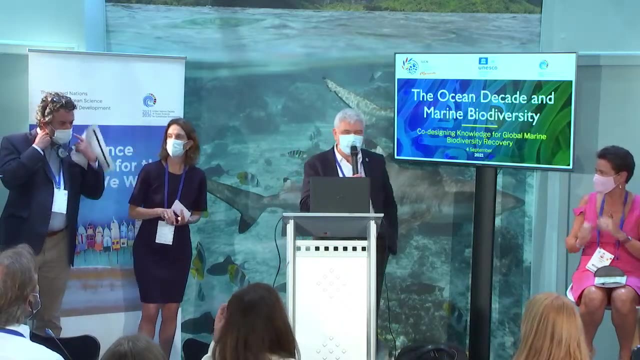 again. so you know, and because i'm russian, i have infinite patience and you know, and persistence, so there will be uh, more and more tries. so, and you know, uh, i think everyone deserves an anecdote. now i don't have one, but i'm uh, i have to then introduce myself. vladimir rebellion executive. 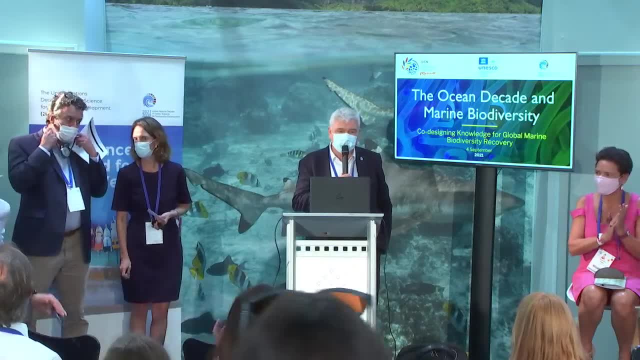 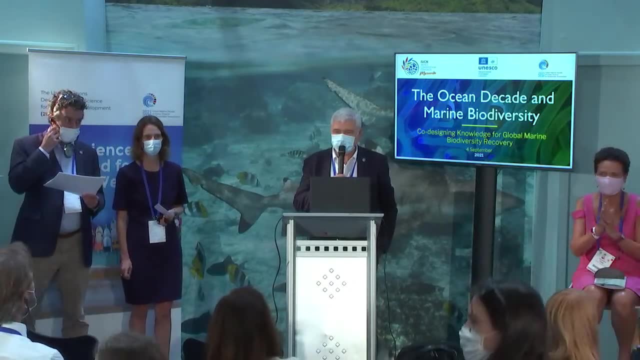 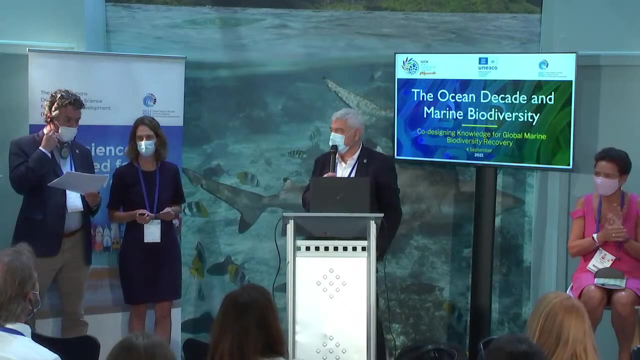 secretary of the in the governmental geographic commission of unesco, which, uh, the variation is ioc, not to be mixed with the international olympic committee. but i think we are really trying to do something that is of the same scale for the ocean and really deserves that. so do we have any any sound? 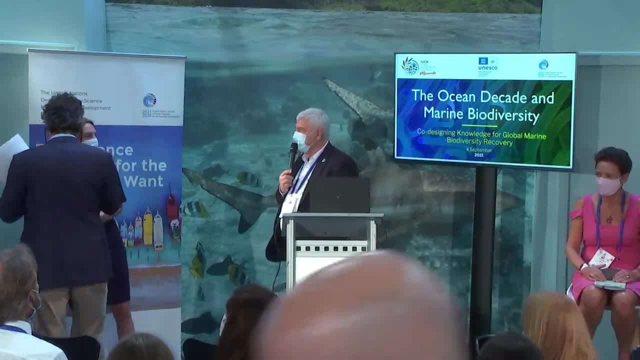 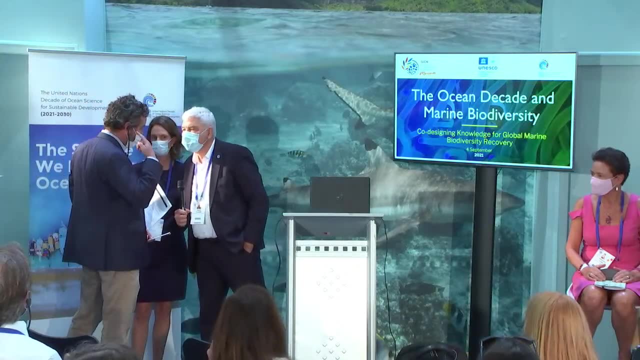 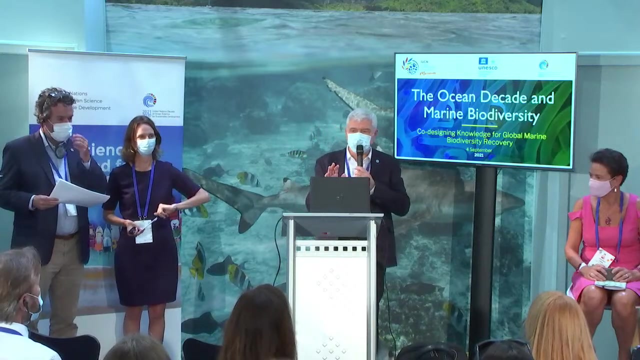 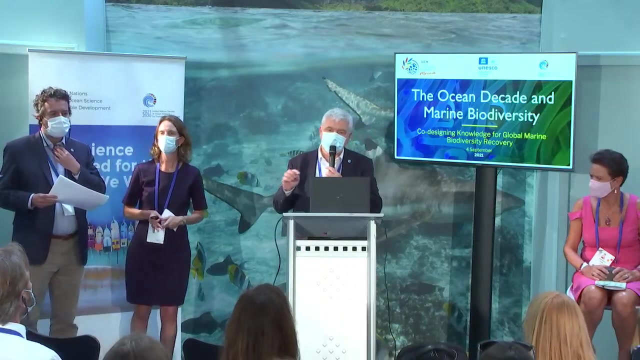 okay, now i keep speaking. i mean, let me, let me be counting. so what is going, what's happening? all right, so now let me have an explanation for you. there is some delay when i speak, and and and when you hear what i say, so we have to bear with that. 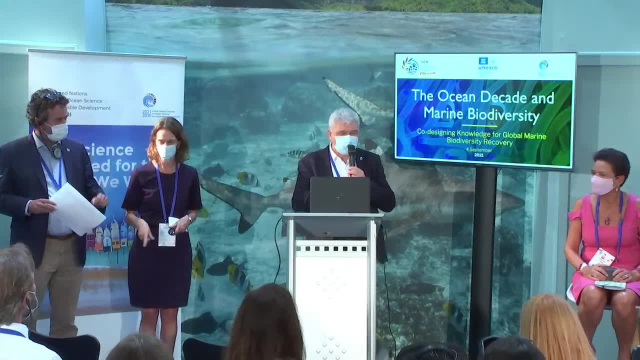 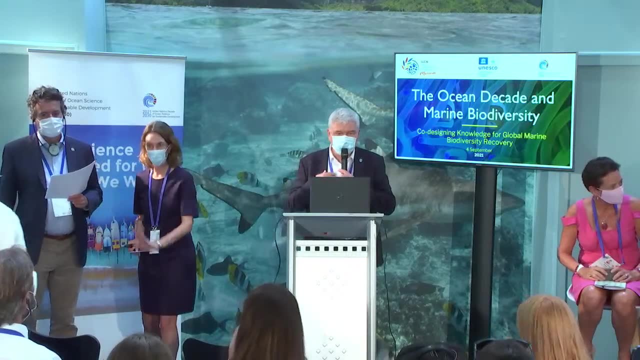 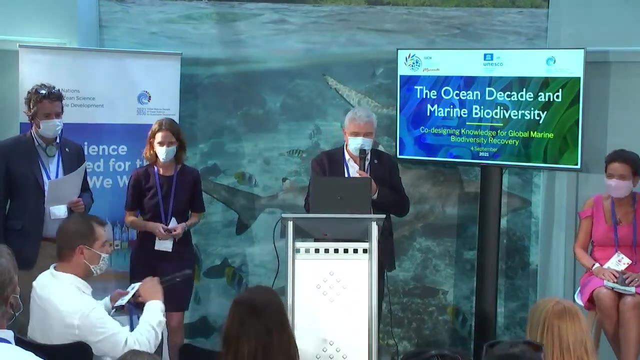 there is no other choice. so, uh, the you know, probably most of you attended the plenary, the opening plenary. what is my take home message from the plenary? there are a lot of heroes, there are a lot of attempts, there are a lot of initiatives, but everything depends on science and 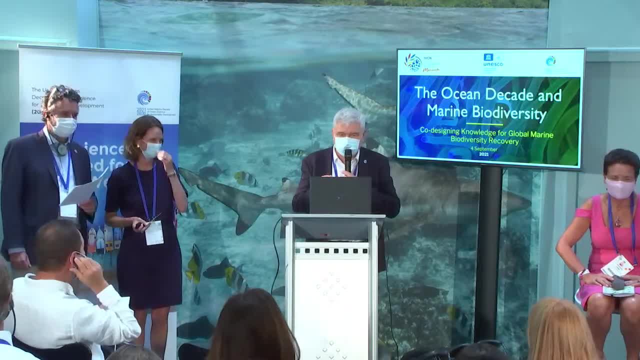 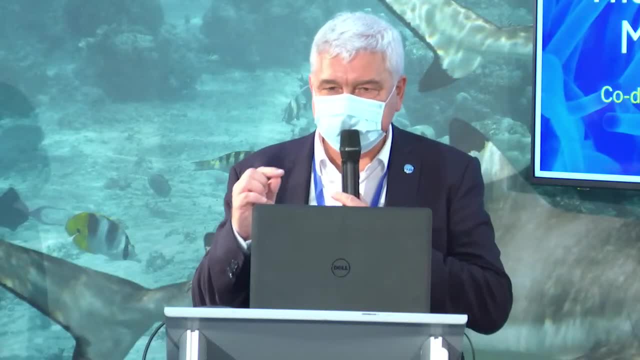 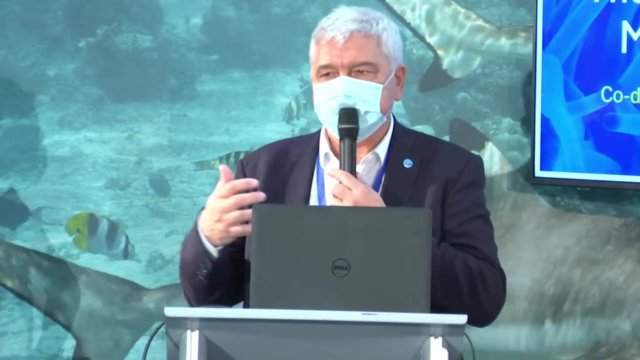 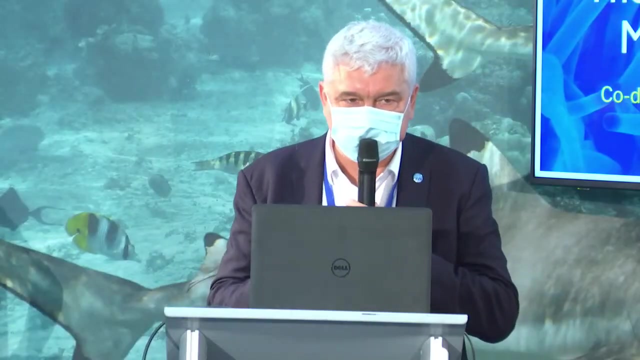 uh. everything depends on having common solutions and the platform for these common solutions. so the decade of ocean science is going to offer a systematic platform for seeking solutions, bringing together people, money, resources, ideas towards systematic processing of information and spitting out solutions in the many domains, including climate, including biodiversity, including economy. 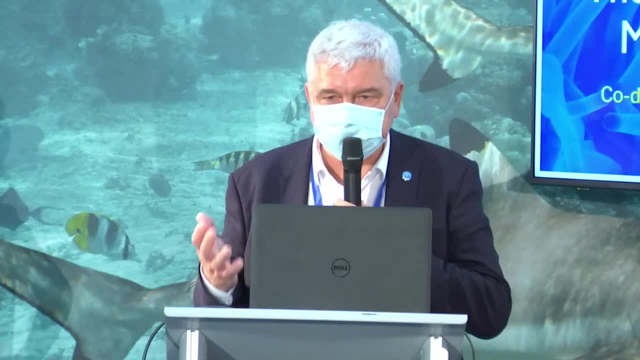 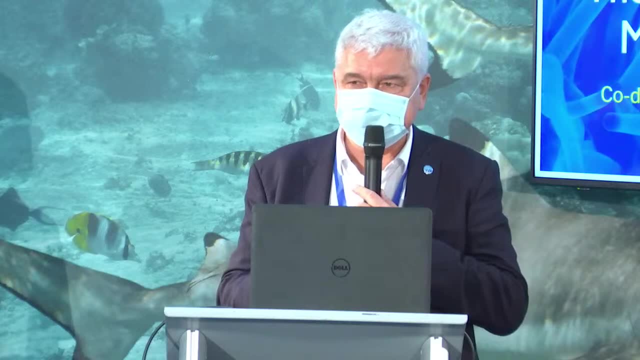 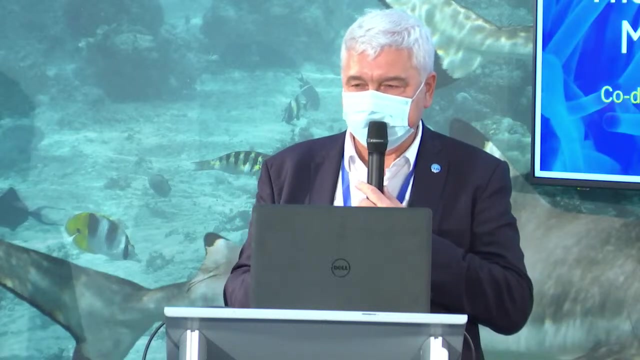 uh, affecting in the positive sense, avoiding poverty, and- and because of that it is very important that everyone engages in this process- becomes a part of this, because solutions are coming for everyone and this is a revolution in ocean science. so i would like to introduce now the moderator of this. 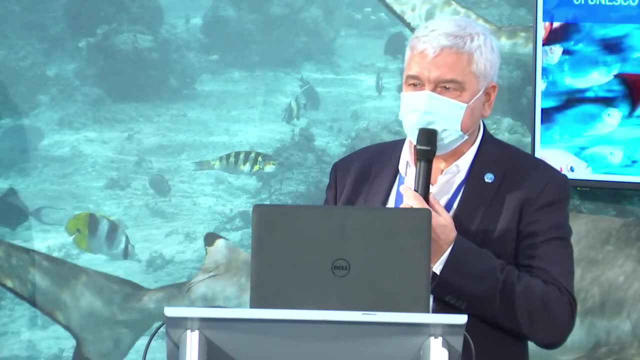 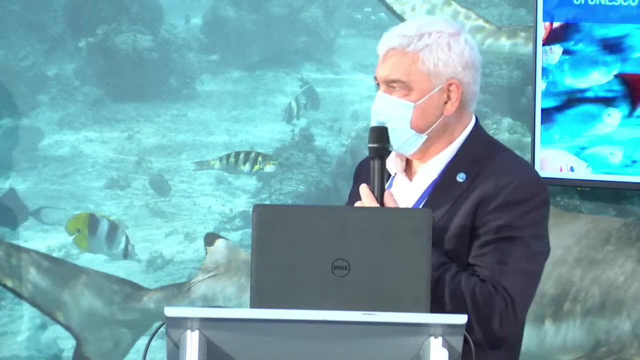 session, julian barbier, who is a head of section in ic, but his important role now is that he is the coordinator of the ocean science decade for sustainable development. julian, the floor is yours. thank you very much, vladimir. good to see you all. bonjour a tous. it's a real pleasure to see real 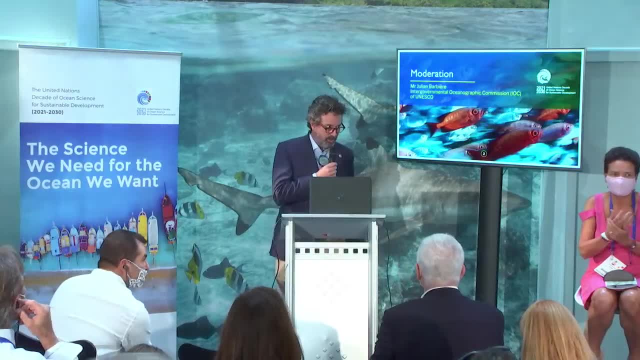 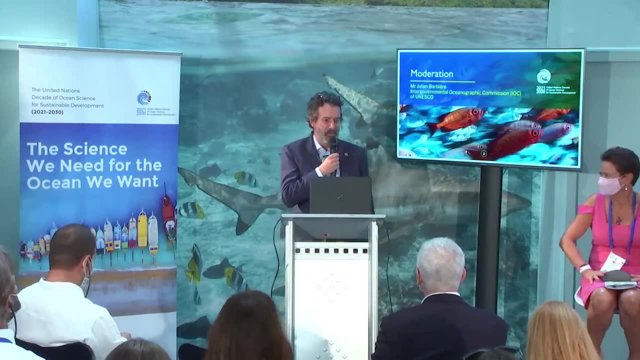 people in front of us today. we spent 18 months in front of a computer and- and sometimes this interaction we've been missing very much and i hope that this will really help us to achieve our goals both in the decade and the biodiversity agenda. so our event today is really to first. 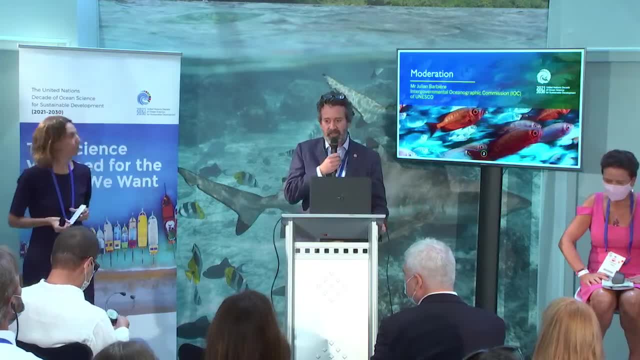 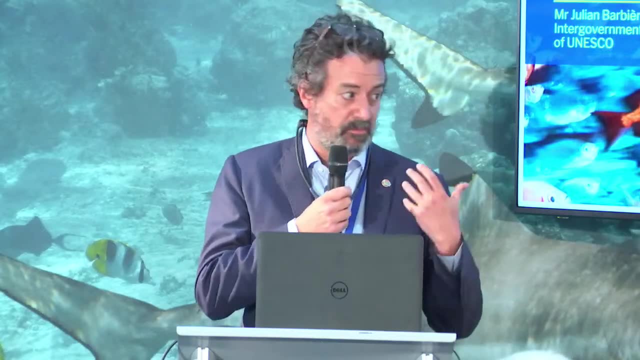 familiarize you with the goals of a decade. so all of us are going to be here today to age, we're going to be here tomorrow. but i want to first give you a little bit of background as to our the ocean decade, which just started a few months ago. but really see how we can articulate this and 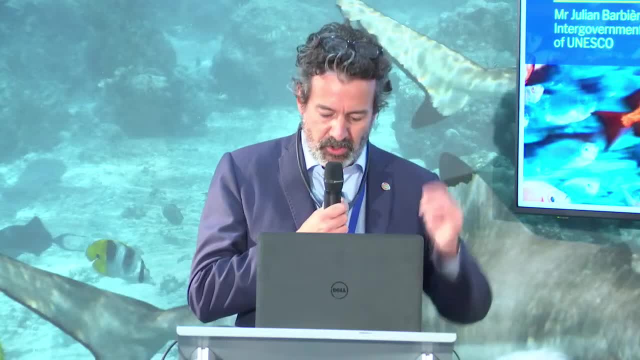 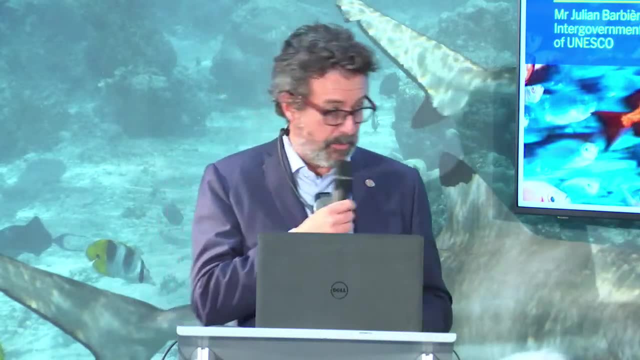 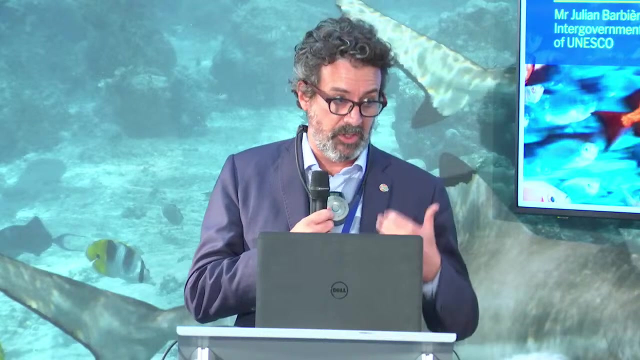 support the whole global biodiversity and conservation agenda. so today we have a great speakers with us who will give you some of the different dimensions of this, of this dialogue. we'll address the issue of the post 2020 global biodiversity agenda, which is still going to be. 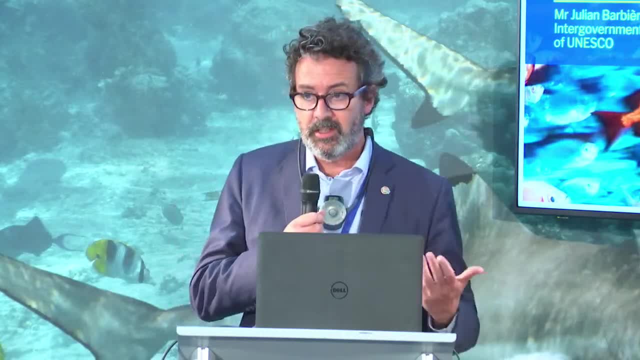 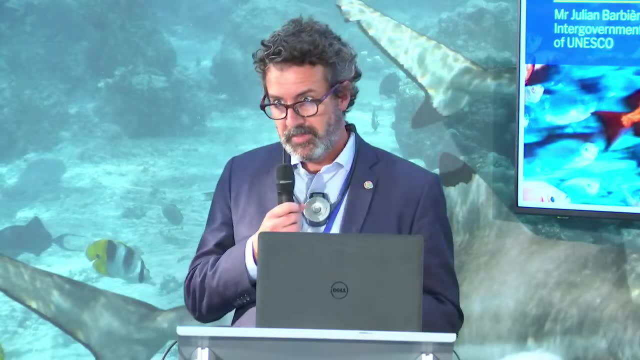 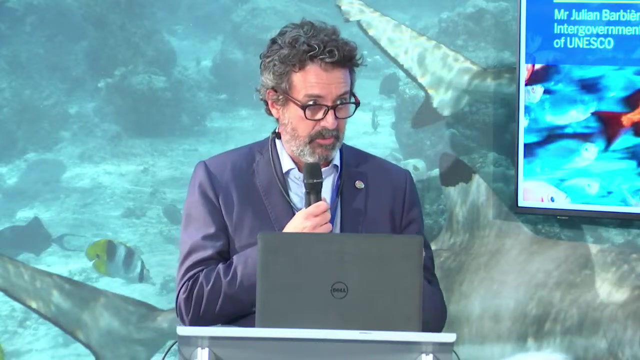 negotiated next year. again, what is the science need? how can science support the effective design and implementation of fbas? for example, we have a global initiative 30 by 30, which really aims to get 30 of the ocean under some level of conservation. again, what other tools? what? 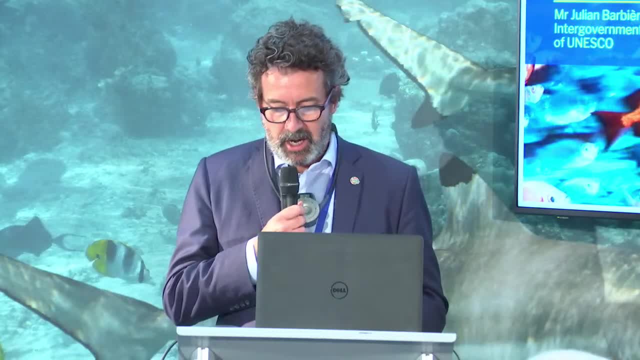 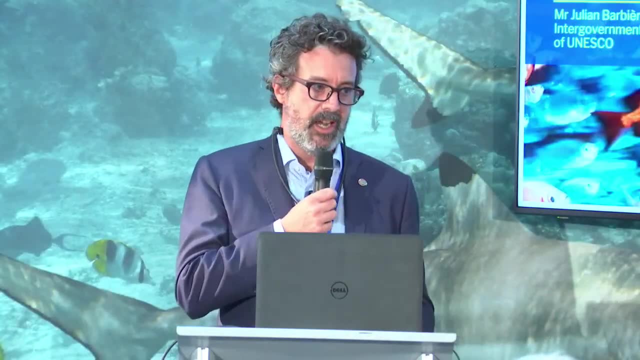 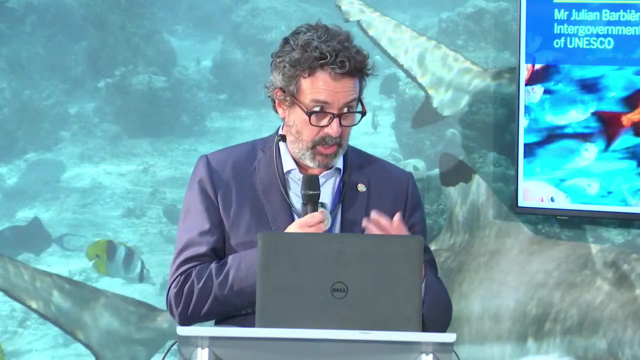 other data that we need to to achieve these goals. and, of course, we have the high seas: 43 percent of the surface of the earth is the ics. we have a unga negotiation next year also on this new legally binding agreement, so we will hear about this. 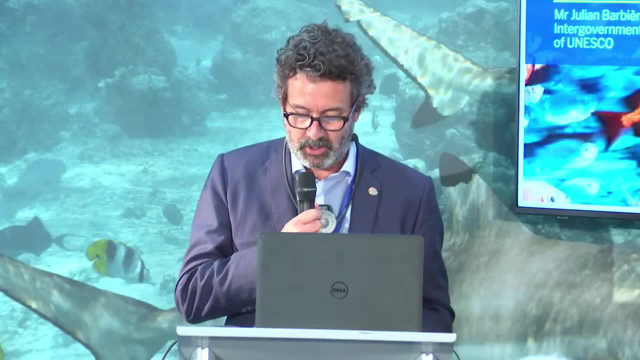 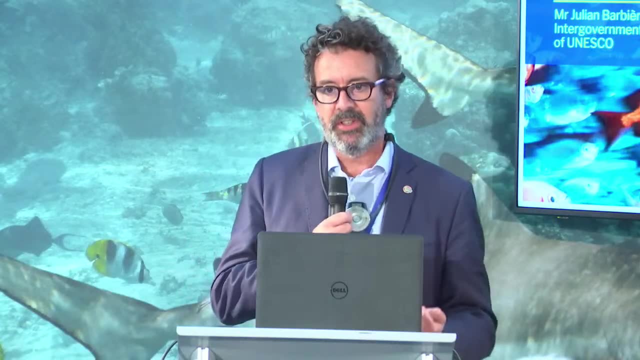 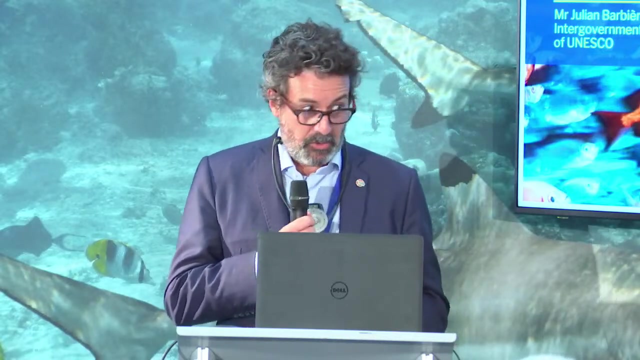 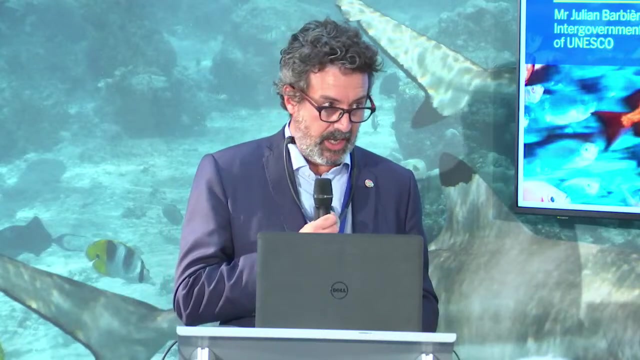 and try to understand where we are in terms of our existing knowledge. we'll try to sum up and also really understand how we can develop this new way of implementing science in the co-design and working with end users towards the delivery of knowledge and actions. so today we are you joining us physically. we also have a live internet webcast audience. 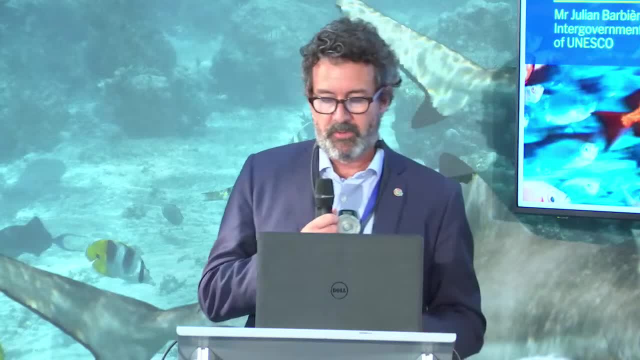 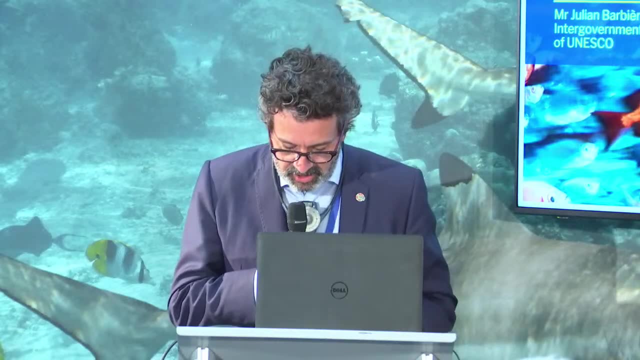 and we hope to have a little bit of time at the end of the of the interventions for for some we will use the slido mechanism, so we have a hashtag: ocean decayed. if you are familiar with slido, you can ask your questions there and we will moderate them. but we will also try 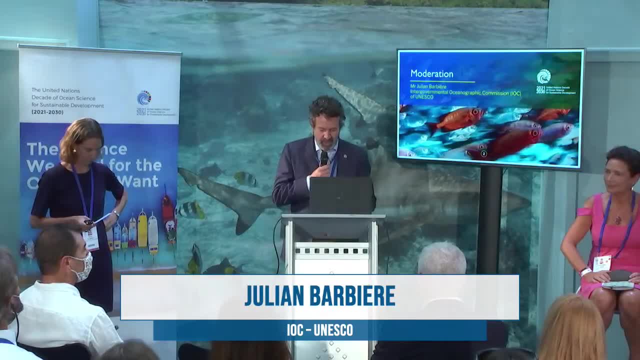 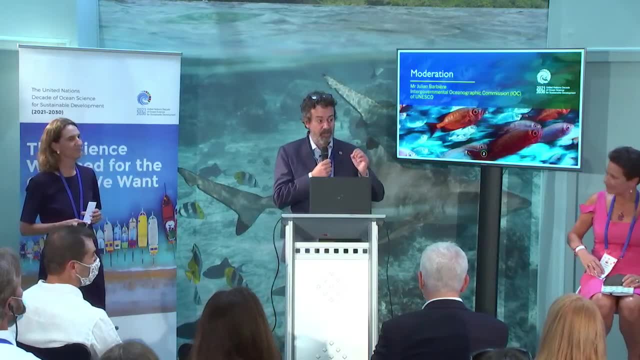 to get maybe a few live questions from from the audience without further ado. before we we go into the panel, you need to have your inoculation for the decay, so we're going to give you a five minute shot so that you get a vision of what the decay is about, how you can engage and how does it link with your inoculation afterwards? so I'm really excited to have you guys in our session. let's just have a quick segment and finish with all this time. well, everyone is on the panel. I think that that's about it for this webinar. thank you very much. I will see you in the classes. and next we have a few more questions. so for all who want to take minute half second diferenciation with each opportunity will find people on the web83 and what sort of way you want to address them and how does it link with the biodiversity agenda. 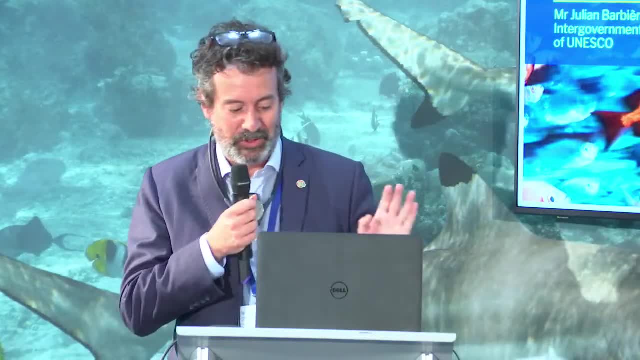 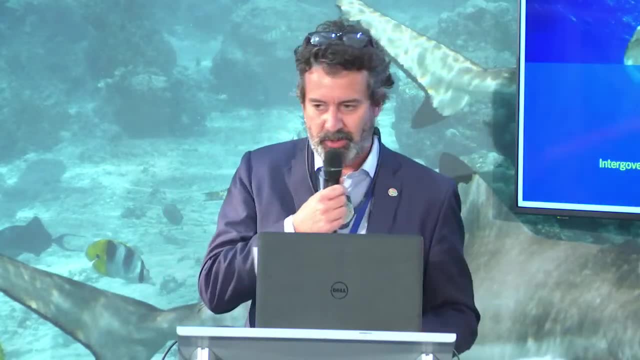 And I can assure you there's no side effects to this. So over to my colleague Alison, who will give you a bit of an overview of EDUCATE, and then we go into the panel. Thank you very much. Thank you very much. 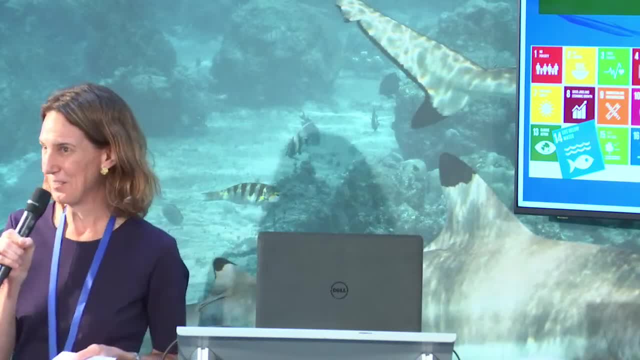 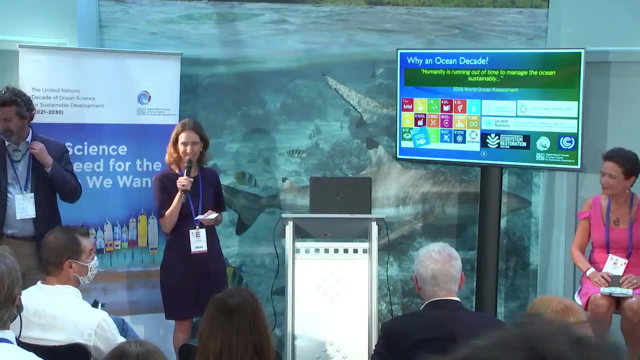 Okay, so I am. Thank you. It's lovely to be here this afternoon- The first live speech I've given in a while, so it's a real pleasure And welcome also to our streaming audience. This seems to be the future, these hybrid events. 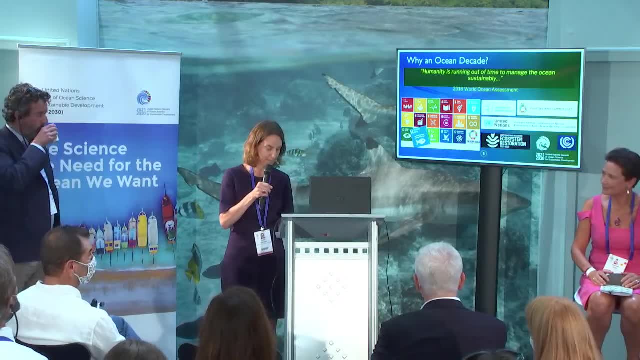 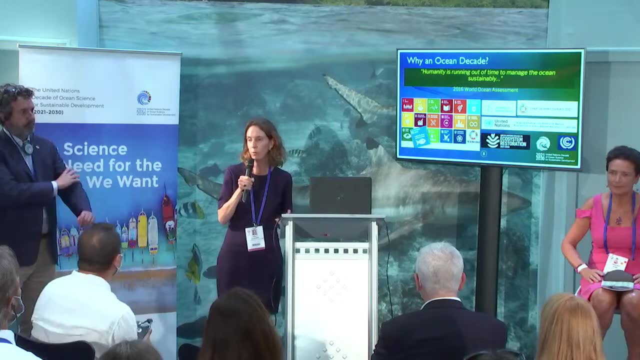 As Julian said, I don't want to take too much time. We've got some amazing speakers lined up- but I think it's important that there is some basic knowledge about the decade. So, first of all, why an ocean decade? Now we all know the ocean is in trouble, right? 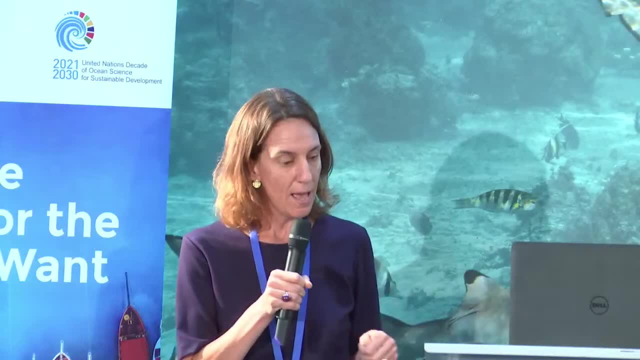 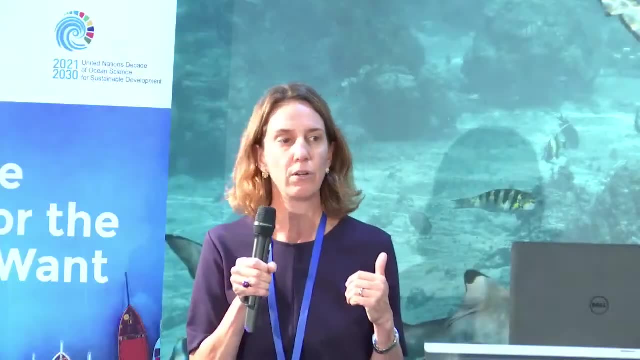 I think everybody is here at this Congress has that awareness. But you know, this quote really sums it up: We're actually running out of time to manage the ocean sustainably. We're also running out of time for the Sustainable Development Goals. 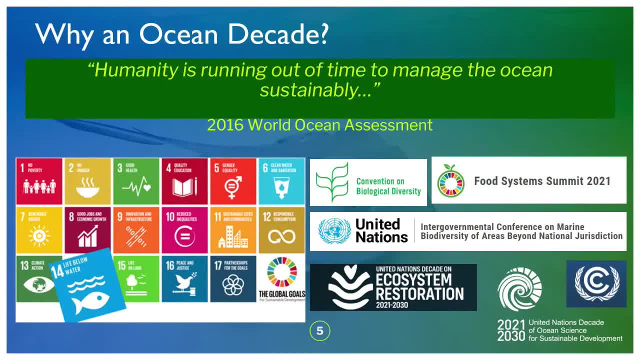 We're running out of time for all these other global aspirations- about climate, about food security, and yet the ocean is central to all of these. Now, one thing that is true, and that is a barrier to meeting any of these aspirations, is that there is a lack of knowledge. 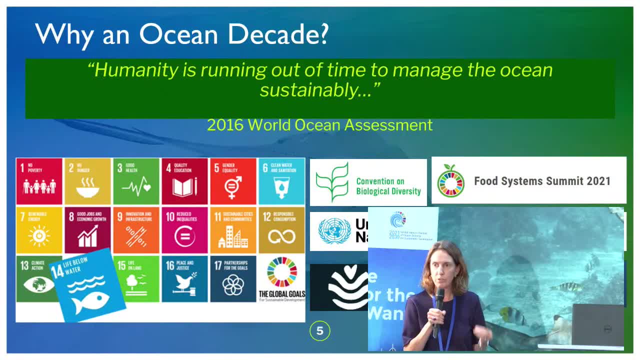 There's a lack of science, There's a lack of co-designed, inclusive, solutions-orientated knowledge, And that is what the decade is all about. Sorry, I'm doing microphones and turning slides. So the ocean. So the ocean decade basically grew out of discussions within the IOC in 2016. 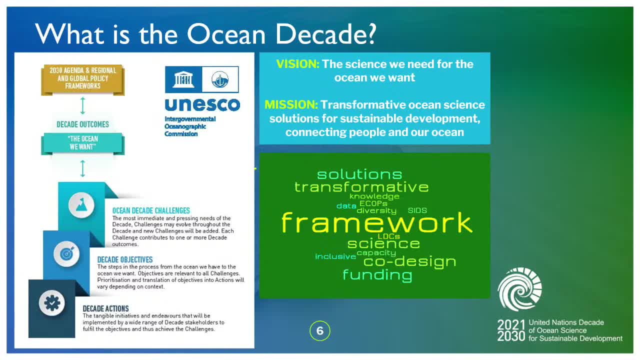 that really wanted to address this lack of knowledge. In 2017, more and more partners came on board, The UN General Assembly proclaimed the start of the decade and we launched into a three-year participatory preparation phase. Now, this was in the days- 2018 to 2020, where people could still get together. 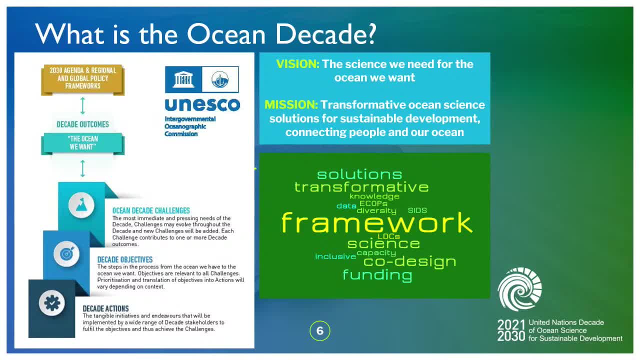 We had thousands of people in regional, national, international meetings around the world. We had thousands of people in regional, national, international meetings around the world. We had thousands of people in regional, national, international meetings around the world to design this decade. 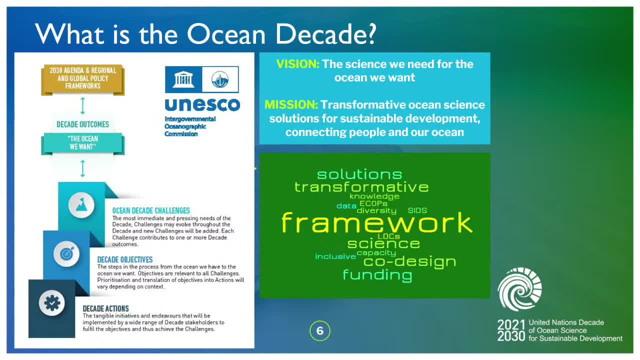 And what did that lead to? Well, you can see here the vision of 10 years, starting in 2021, where we are going to work together to generate the science we need for the ocean we want. The mission statement sums it up: It's all about transformative ocean science. 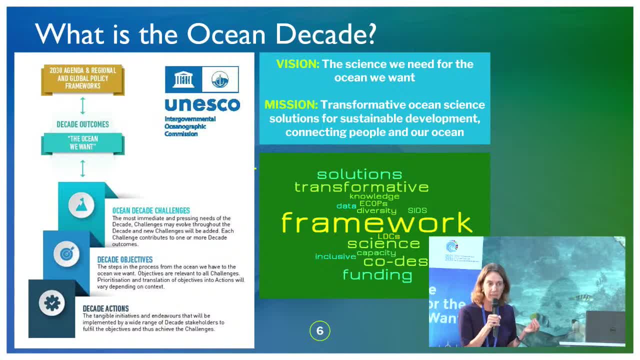 solutions for sustainable development that connect people and our ocean. We need to change behaviour. We need to change individual behaviour. We need to change institutional behaviour. The decade is going to do this through the Decade Action Framework, which some of you who know the decade will be familiar with. 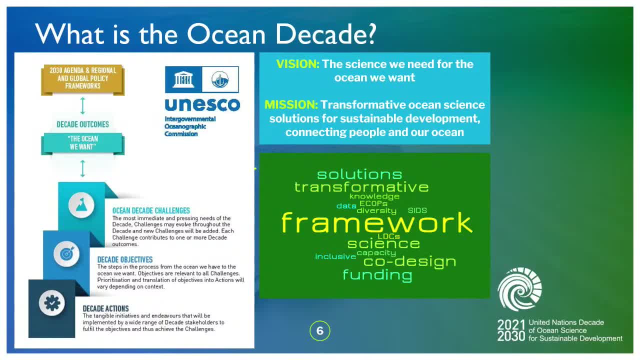 We've been touting this on Zoom calls for the last two years now, where groups- if you start at the bottom, where groups of people all around the world will come together to co-design and to implement decade actions in the form of national, regional, international actions. 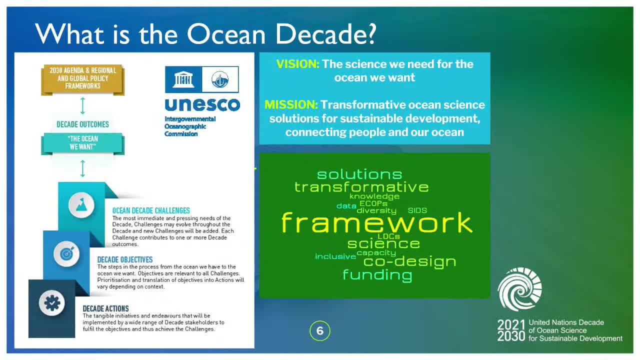 These will work at all different steps of the ocean science value chain, from the identification of knowledge, to the generation, to the creation of knowledge, to the use of knowledge, to the building of the capacity to be able to use and apply ocean science. 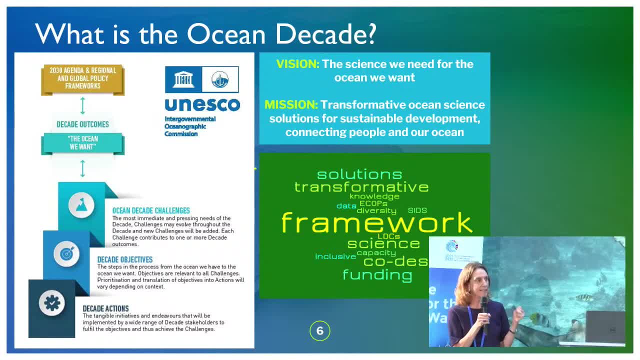 And this will respond to 10 major ocean decade challenges. These are the challenges that, collectively, we have set ourselves for ocean science for the next 10 years, And they range from pollution to ecosystems, to biodiversity, to climate, to the infrastructure we need for science. 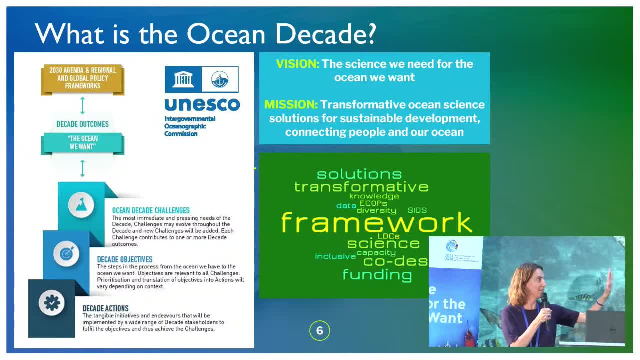 to capacity development, to behaviour change, And you can see here this word cloud, some sort of change. It sums it up: It's about solutions, It's about transformative, It's about providing a framework for collective action over the next 10 years. 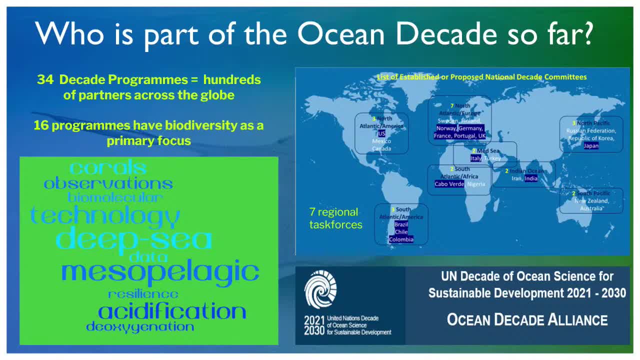 So who is part of the decade? so far? We have numerous partners. We've had a three-year preparation phase, nine months of implementation. We have planted the seeds of the ocean science revolution that Vladimir just mentioned. There are 24 national decade committees that are up and running. 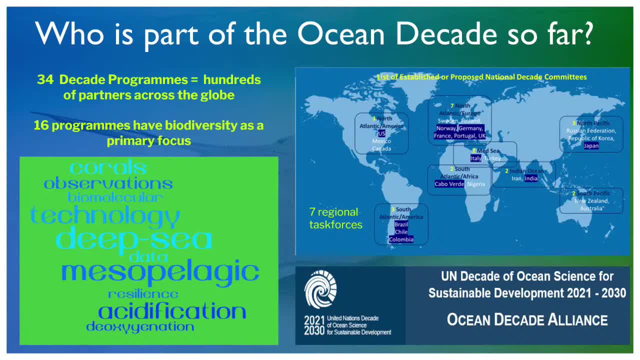 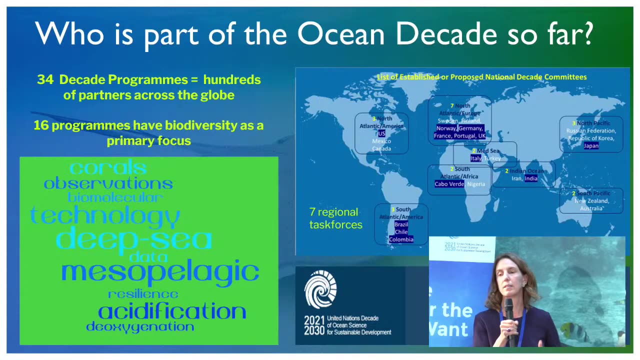 many more that are getting underway. We have seven major regional task forces, From the Arctic to the Southern Ocean, that are identifying the regional, the national priorities in ocean science needs for the next 10 years. We have the Ocean Decade Alliance, which is philanthropy- UN agencies. 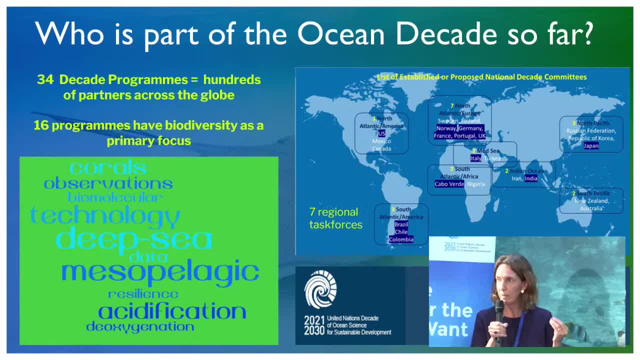 private sector governments coming together to help us mobilise the resources And at a very concrete level, we have 34, our first 34 global decade programs, of which we have representatives here today on the panel in the audience, who represent hundreds of partners across the globe. 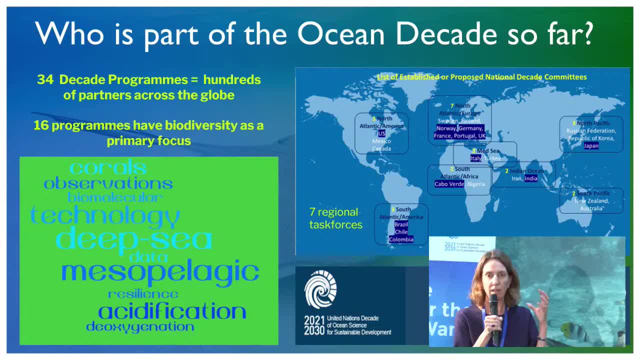 who have committed time, energy and resources to carrying out the first building blocks of transformative ocean science. Sixteen of these programs have a strong biodiversity and ecosystem focus. They have mobilised and leveraged already US$800 million for ocean science and they have an ambition over the next three years alone to leverage $2 billion more. 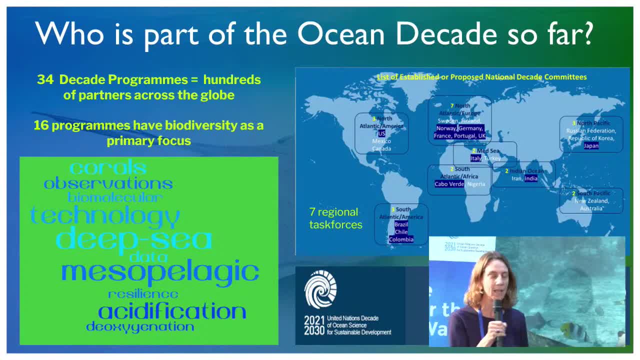 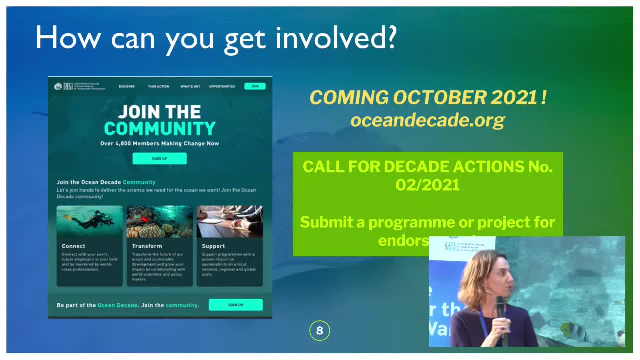 So you can see, we're not talking about something small, We're talking about global. We're talking about a global ambition, but a very necessary global ambition. My last slide then: if you're convinced, how can you get involved in the ocean decade? 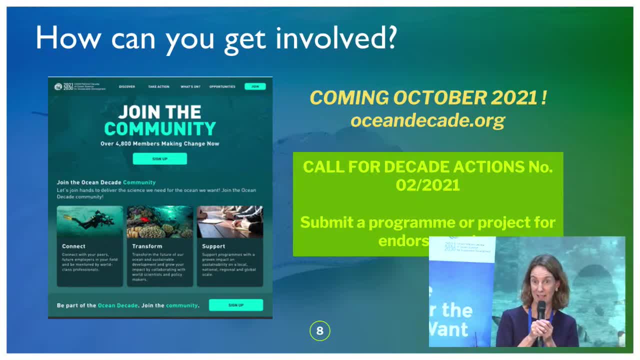 Well, it's a great time to be hearing this, because October this year is a big month for the ocean decade. We have two big new ways of getting involved that are really going to make it easier for the decade really to become everyone's decade, as we say. 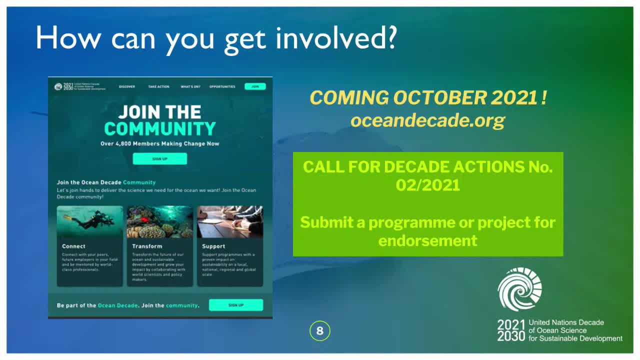 We have a global stakeholder forum, which will be launched in mid-October, which is the place that everybody can come together, collaborate, exchange, work in communities of practice, join decade programs, incubate ideas for the decade. So keep an eye on our website and you'll see information soon on how. 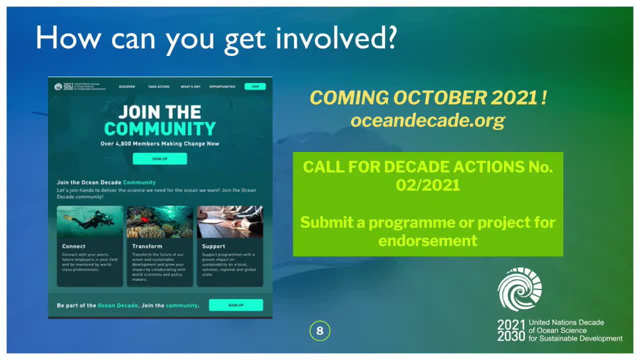 to join this global stakeholder forum. We're calling it the LinkedIn for the ocean decade and we've seen some test runs. It's fabulous. I think you'll really, really appreciate the collaborative nature of the forum. And then we have our next call for decade actions. the 34 programs that I mentioned to you came. 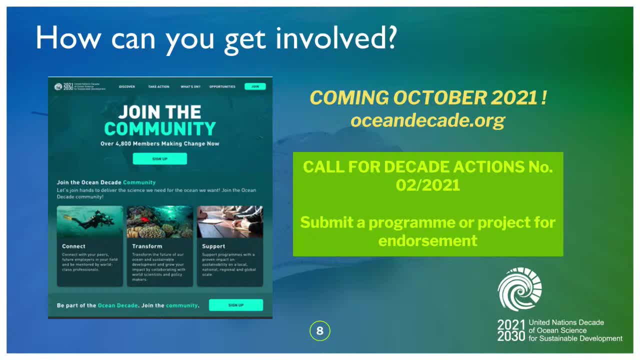 through a first call for decade actions. We have a second call for decade actions, which will be launched in October, where we will be asking partners around the world to submit projects and programs, ideas to become part of the ocean decade. So we hope you will join us in the global ocean science revolution and create the science. 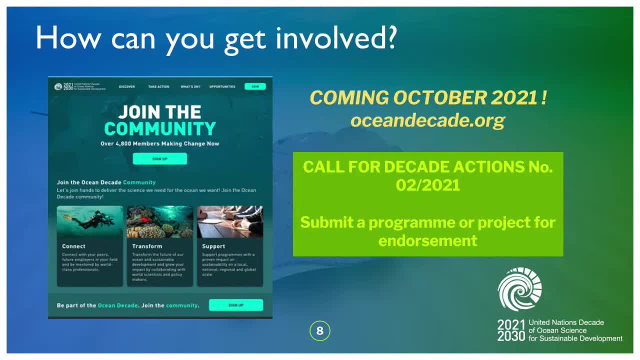 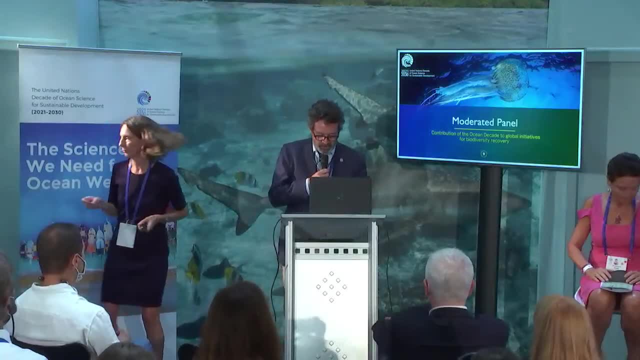 we need for the ocean we want by 2030.. Thank you very much. Thank you very much, Alison. So now I hope we'll just interrupt If you have any information. you are all up to gear with what the decade is and basically. 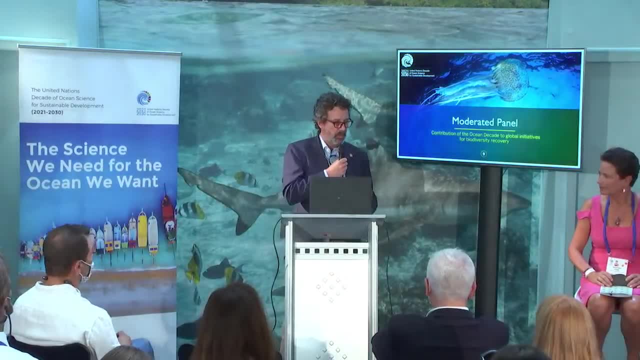 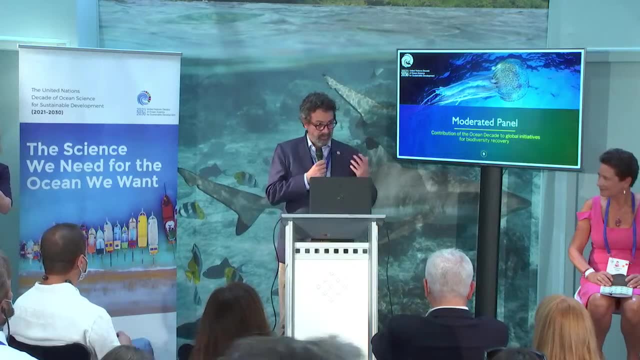 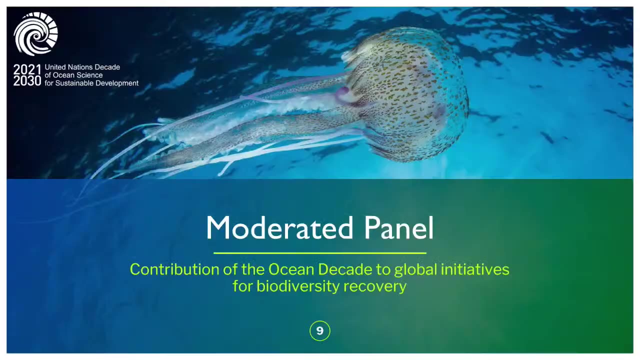 a global framework for prioritizing our needs and our investments in ocean knowledge. Right Now let's go into the substance of our panel. Our first segment is really to see how the decade really articulates with the overall global biodiversity framework and, in particular, the CBD agenda. 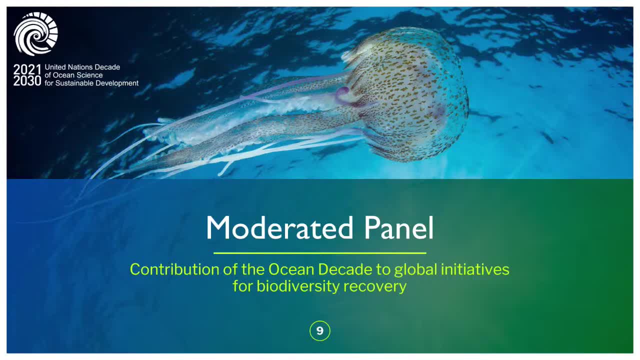 So to talk about this we have Dr David Obura, who is the founding director of Cordio East Africa. Cordio is a knowledge organization supporting sustainability of coral reef and marine systems in the region, And his primary research focus is on coral reef resilience, in particular, climate change. 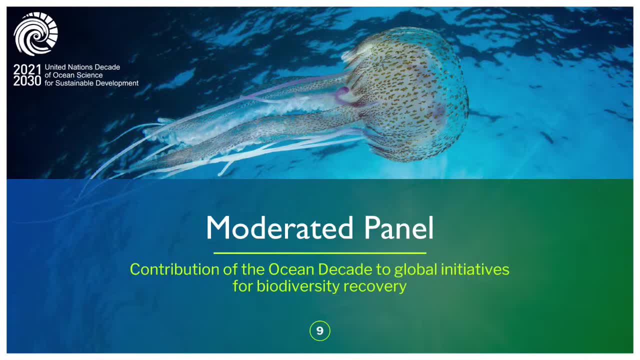 And, of course, David has been supporting many scientific processes: the global coral reef monitoring network, the global ocean observing system, biology and ecosystem panels, amongst a few. So let me start with a first question for you, David, because you are clearly well familiar. 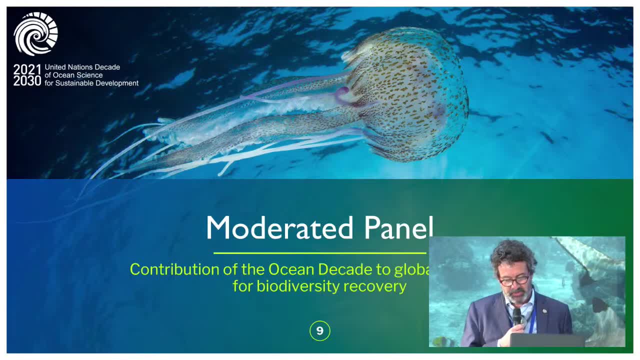 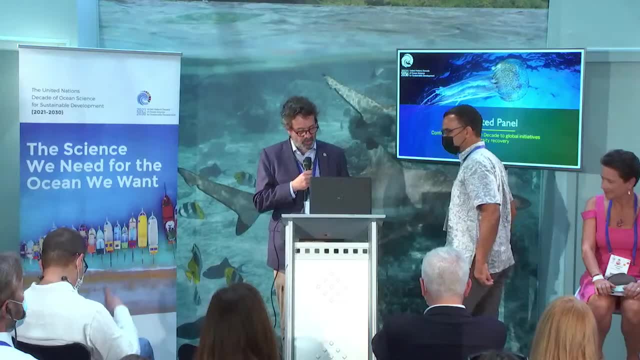 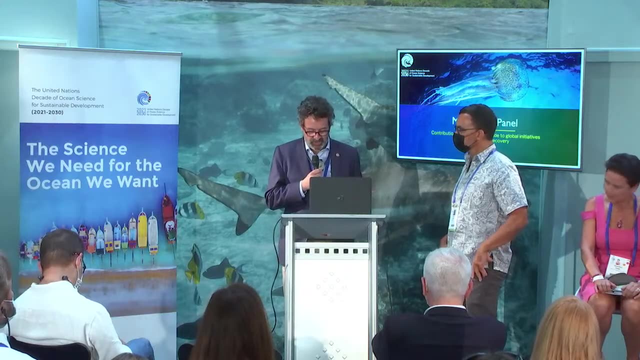 with the decade, But you've also been involved in the post-2020 framework And, as you know, the ocean decade recognizes the importance of measuring progress and evaluating impact over the next 10 years. So, from your perspective, where do you see the synergies between those two processes? 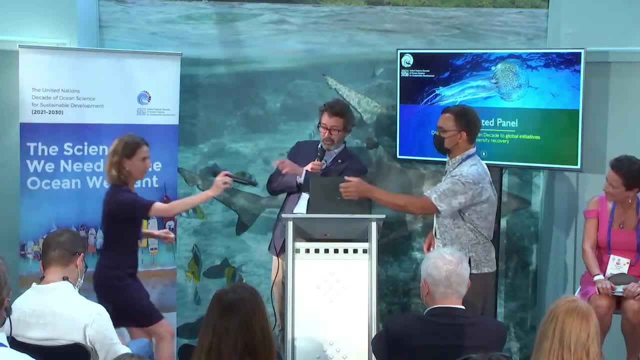 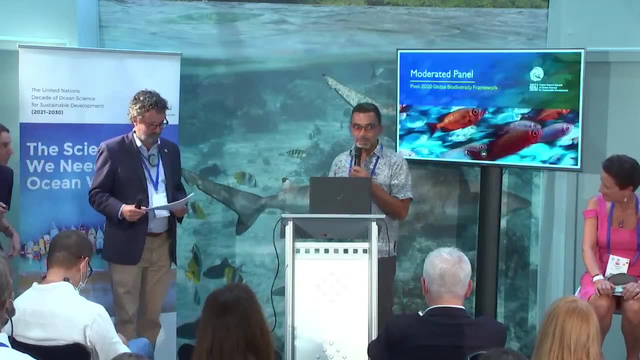 and how really the decade could facilitate that process, And you'll use the next mic, which is clean. Thank you Over to you. All right, Thank you, Julian. I hope everybody can hear me. Thank you, Yes, so thank you for inviting me on this session. 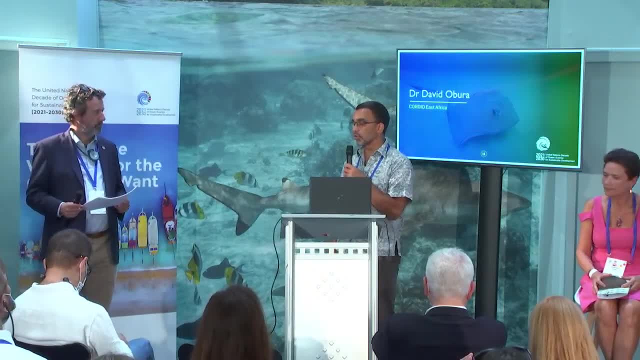 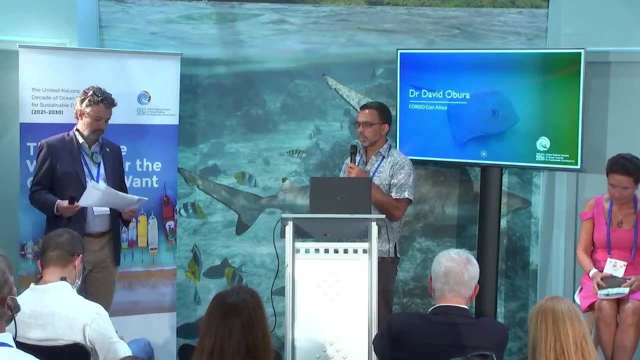 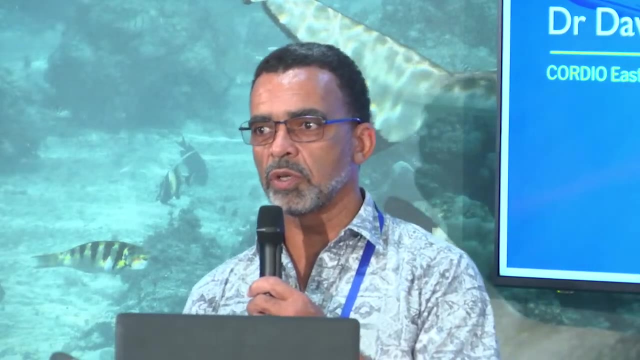 As you said, I have been very much involved in coral reef monitoring around the world- in Kenya and East Africa, in my region, but also globally- And through that I've become involved in the GOOS- the Global Ocean Observing System- process of establishing global monitoring networks and global observing systems. 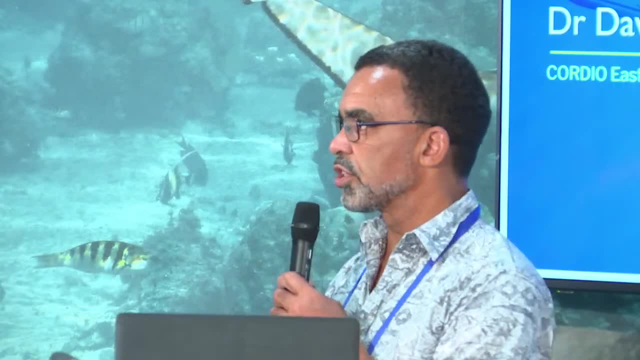 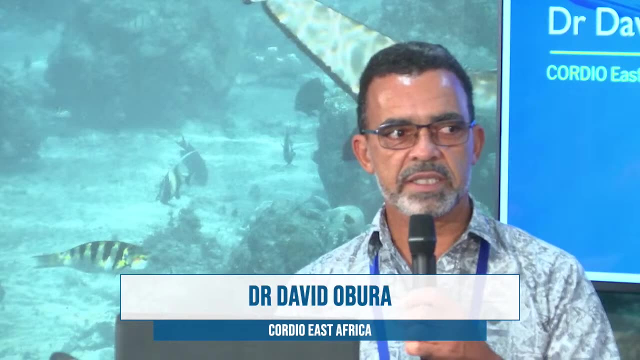 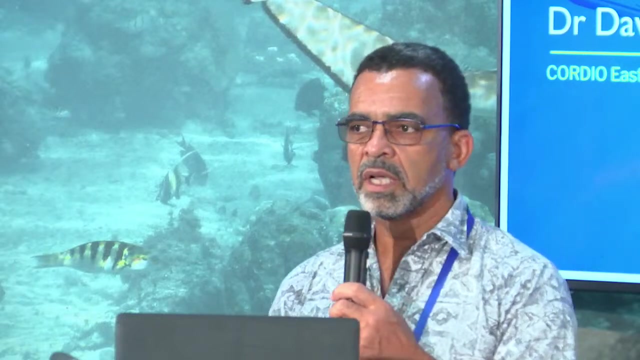 The GEOBON, the Group on Earth Observations, Biodiversity Observation Network, which is the observation network, also has a marine program. And all of this? the purpose of doing this is really to feed data into convention processes so we understand the ocean, we know its state and can report on it effectively. 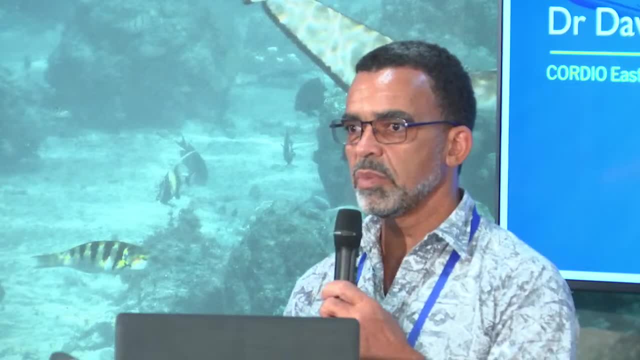 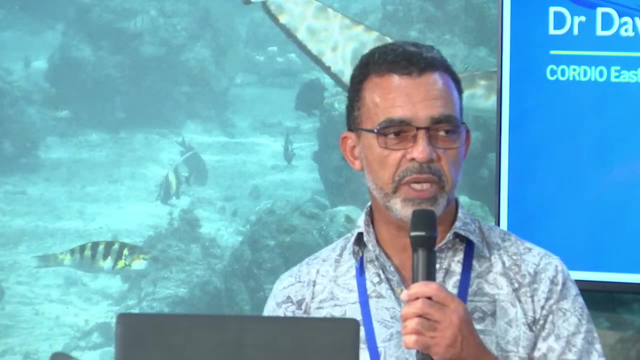 And so, with the Global Biodiversity Framework under the CBD being negotiated currently, it also has a huge process right now to identify relevant indicators to understand the state of biodiversity across the planet. Of course, a lot of the focus is on terrestrial areas. 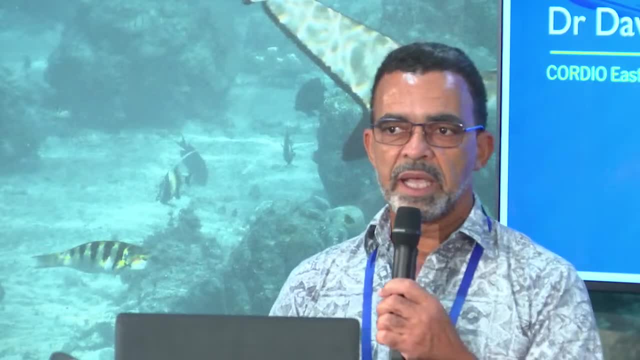 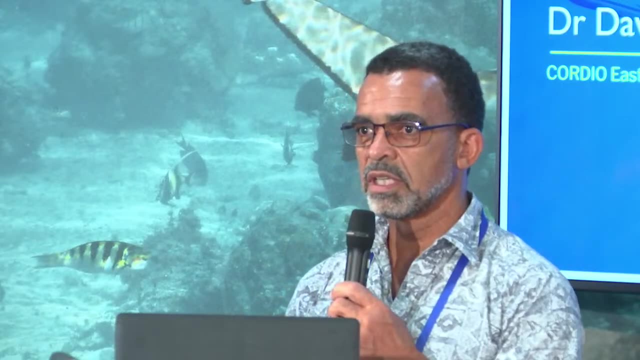 But there's also, of course, the ocean, There's also, of course, very strong oceans components, And so both processes have actually undergone very detailed and very extensive consultations over the last few years, while the COVID processes, of course, locked us all down and 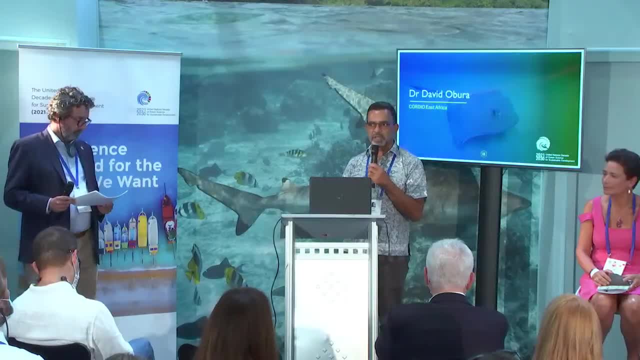 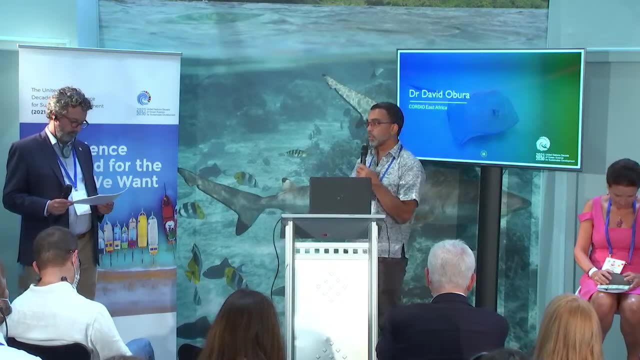 away from what we normally do. for 18 months, It's actually provided additional time for technical processes to catch up, in a way, And so I think that now we're in a better place for understanding how we can monitor and evaluate these two processes and how the decade can really support the ongoing processes. 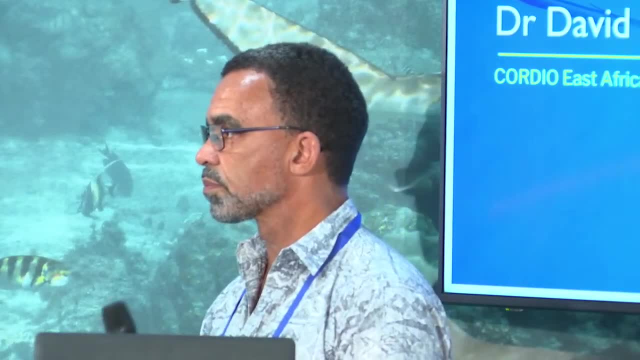 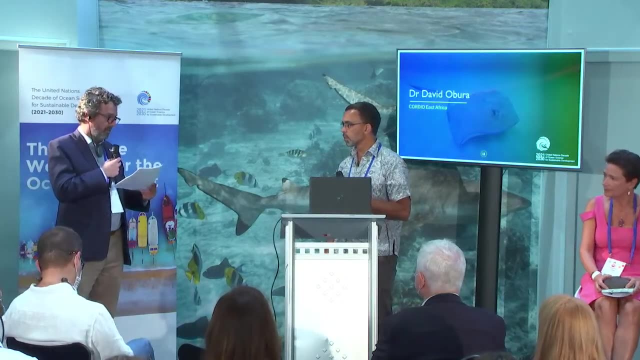 under the convention over the next 10 years. Great Thank you. So, as you know, the decade is a global initiative And, of course, it's very important that it's inclusive and all regions of the world have the means to participate and benefit from the output. 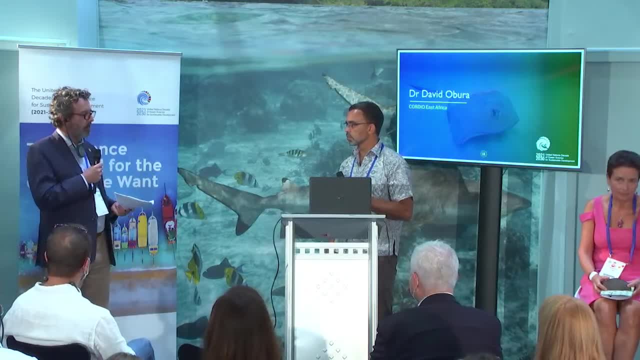 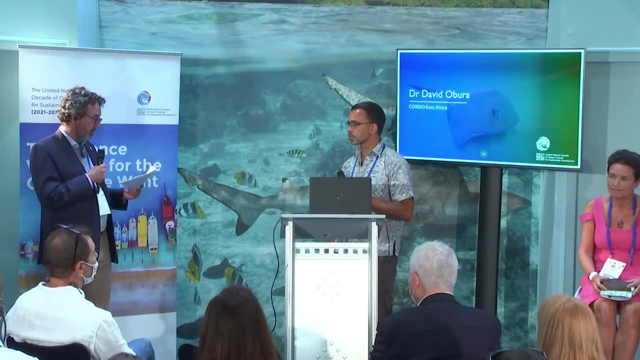 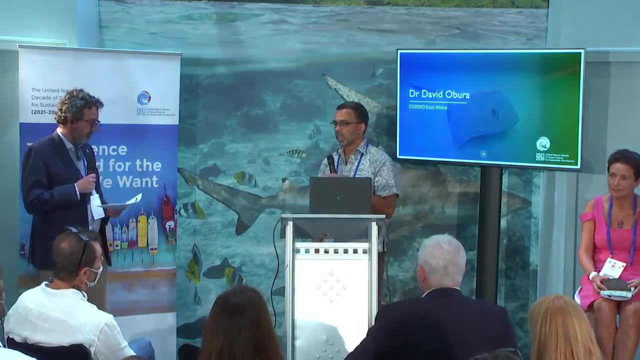 So, from your experience, particularly in Africa, what might be the barriers but also possibly the opportunities for countries to access? you know biodiversity data and you know data And use this data for informing management and conservation efforts. Yes, 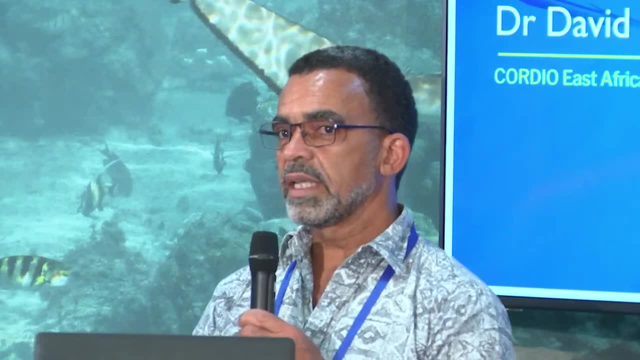 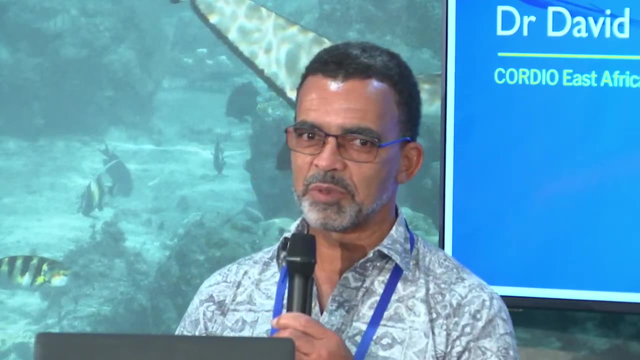 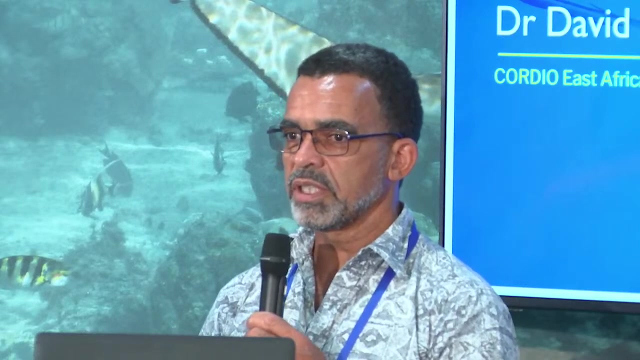 So there's certainly. so, looking at the next 10 years priorities for the decade. well, it's nine years now, of course, because we're sort of, you know, the time has been running away with us with COVID And, as COVID has shown us, the networking of people together is a huge challenge. 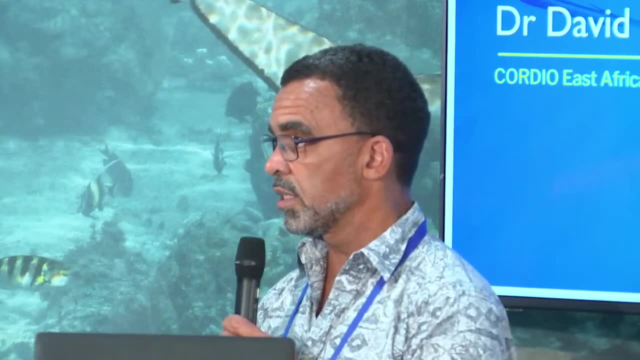 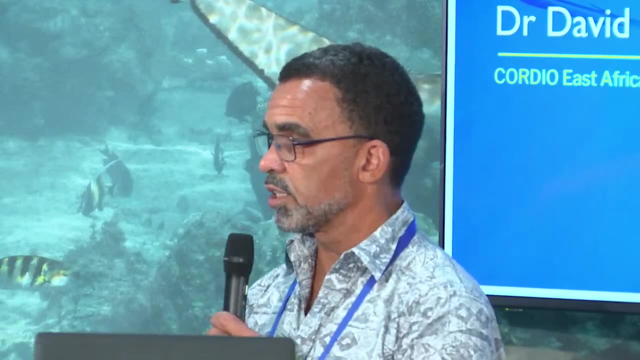 So, particularly in Africa and other parts of the world, there's a huge digital divide. There's a lot of challenges. There's a lot of challenges around being able to, you know, even just access the internet and get on to sessions like this- participate remotely. 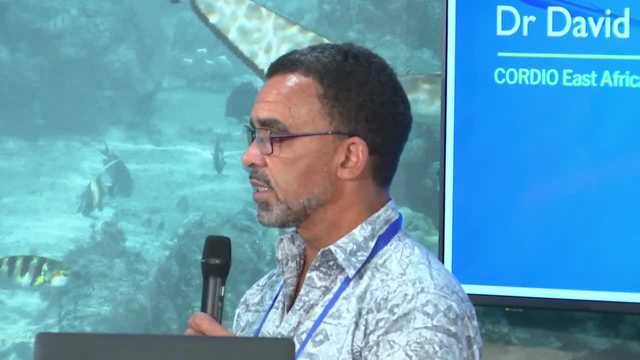 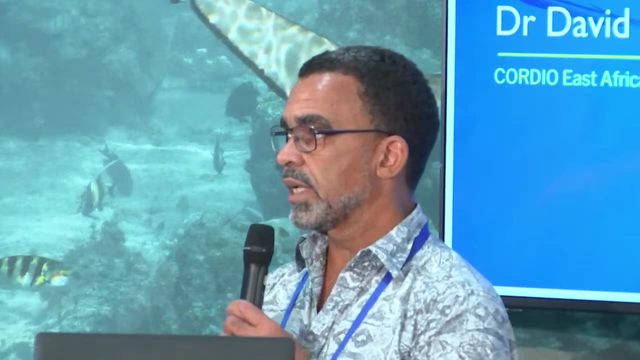 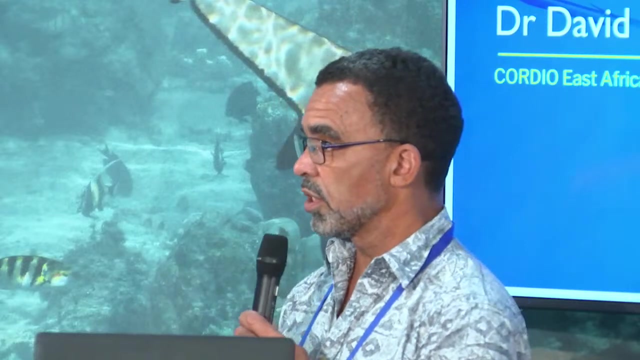 But it also counts for data as well: accessing data, where there's a lot of global data that's available, particularly on atmospheric and physical ocean variables, But actually accessing that for African countries is very hard. So I think those two things are really, I think, critically important as priorities. 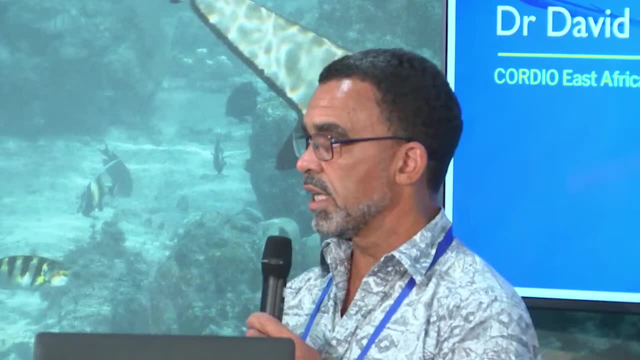 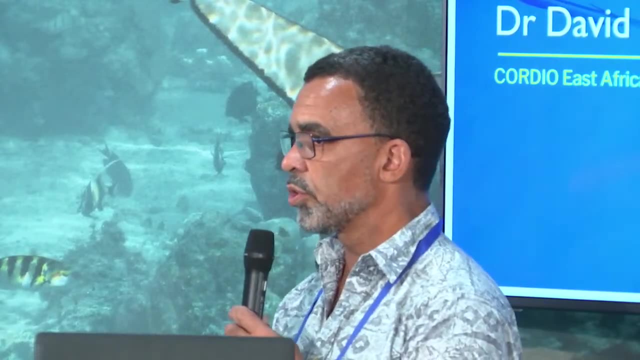 for the decade to really build up is: one is building up the data networks, The infrastructure around being able to share data, And I think that is, of course, one of the priorities of the decade, with the Ocean Info Hub being developed. And the second thing is then building the capacities for countries to participate in. 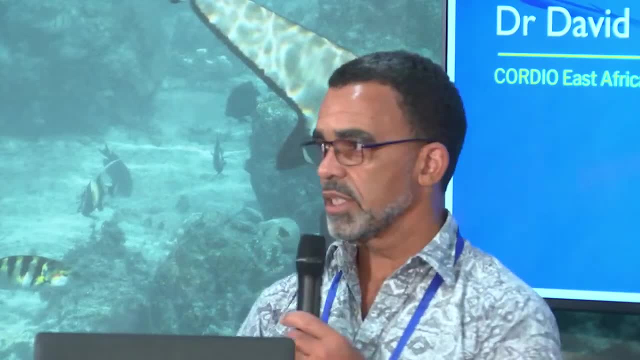 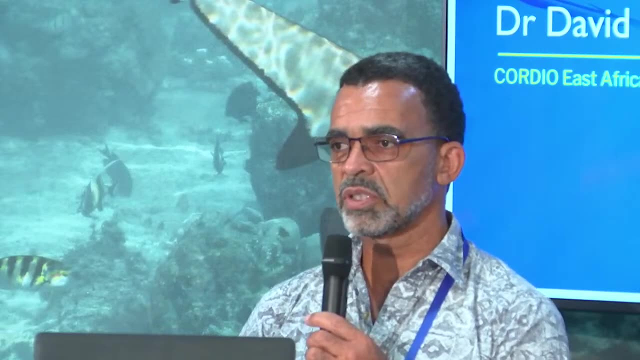 that infrastructure, because if it's no use of being there if people can't participate in it. And of course that needs trained personnel, it needs more equipment, it needs a lot more sort of sharing programs and capacity building and training. And then the other thing that's really critically important that I think we need to do is to 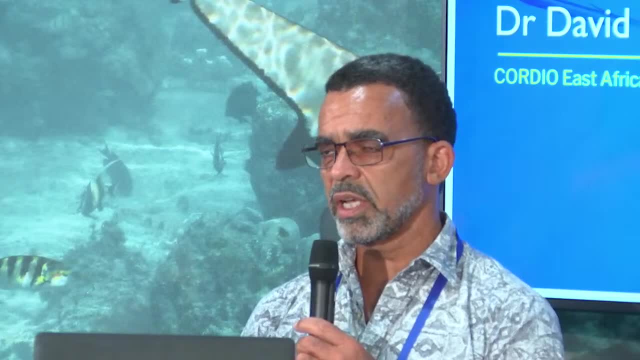 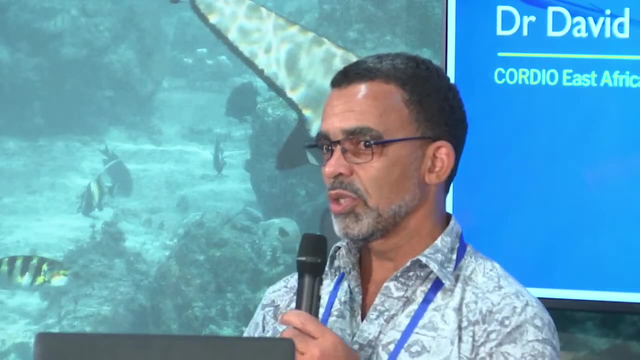 build up the infrastructure And I think that's the most important that I think the decade can help really emphasize is that when it comes to monitoring information, to understand the state of the ocean, you need regular money. It's not enough just to build up a program, have two years of training or put in an institution. 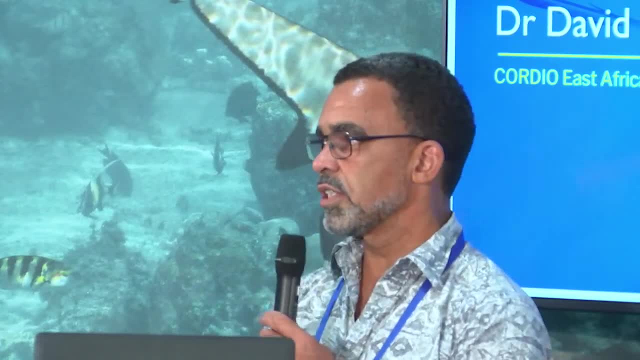 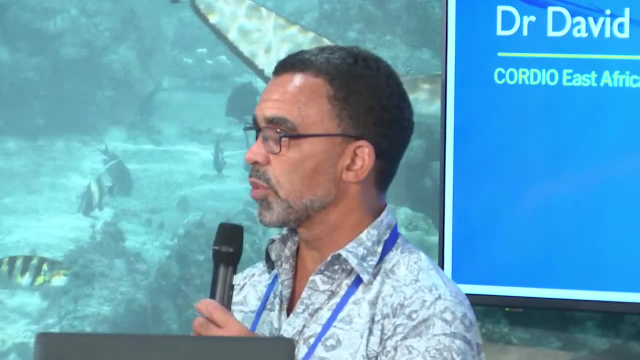 or some equipment. You also need to make sure that you have sustainable financing for salaries and for ongoing expenses and things like that. So I think that's another area that certainly from an African perspective, that's a big priority. Great, The whole issue of sustainability again. 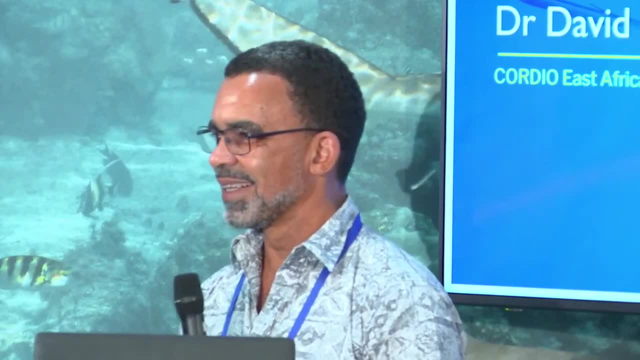 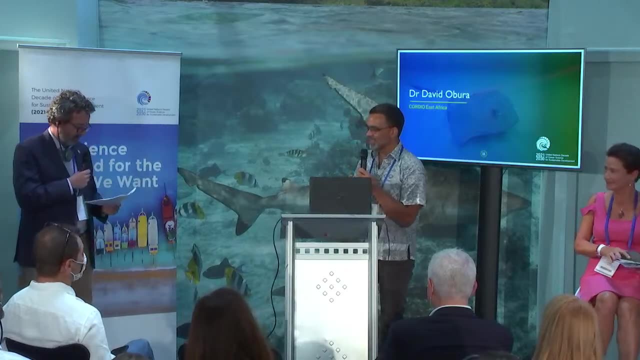 Great. Thank you very much. I will let you go because I know you need to run to the other side of the conference venue, But you will be back at the end of the session for the Q&A, so thanks again, David. 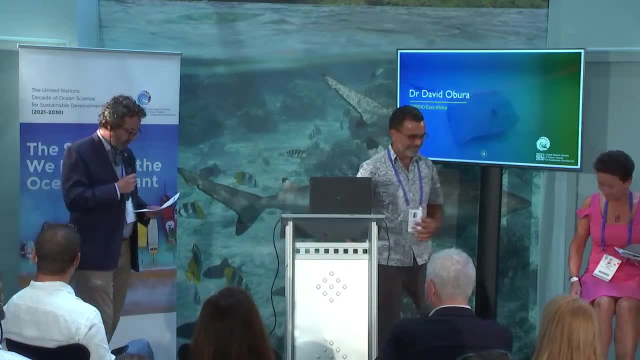 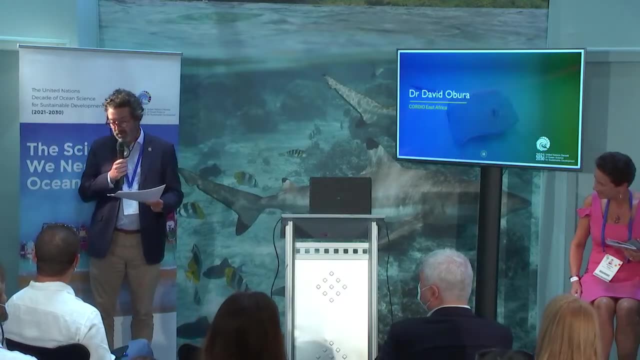 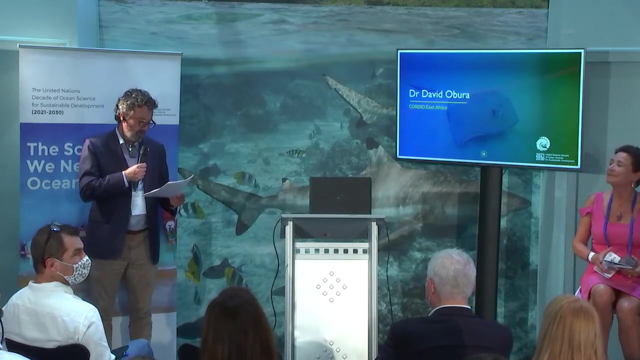 And we'll just then move on on our agenda. and we're going to hear from the Convention of Biological Diversity, in particular our colleague Joseph Appiot, who could not be with us today but sent us a pre-recorded video. He's the coordinator of the Marine and Coastal and Island Biodiversity Program of Australia. 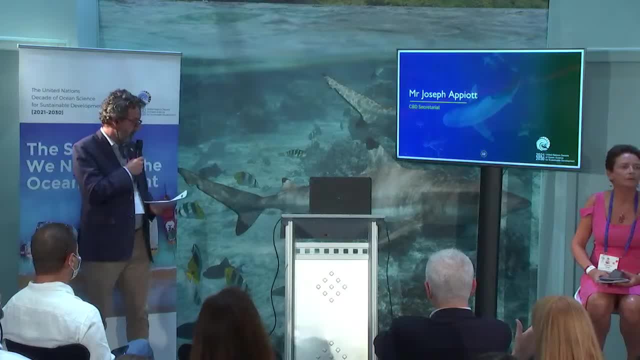 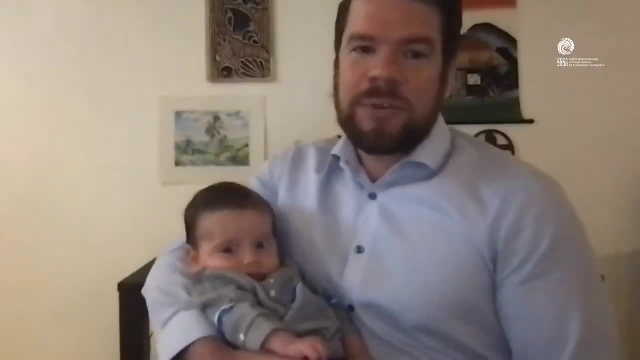 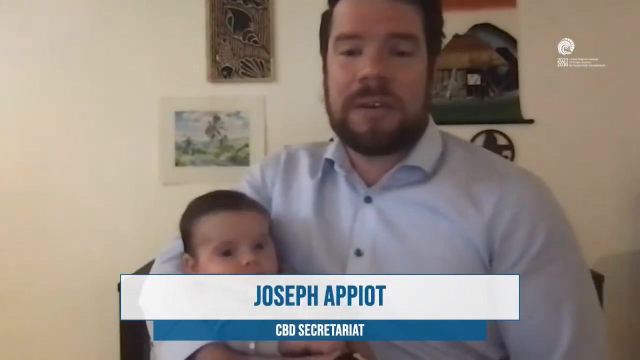 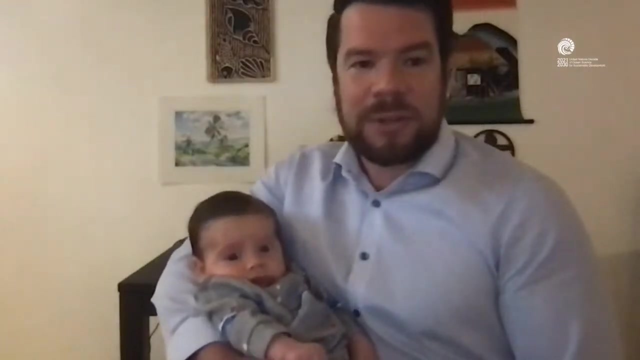 So if we could please just have the video. Thank you, Greetings from Montreal, Canada, the birthplace of professional ice hockey and Celine Dion, but, most importantly, the home of the Secretariat of the Convention on Biological Diversity. My name is Joe Appiot and I coordinate the work on marine, coastal and island biodiversity. 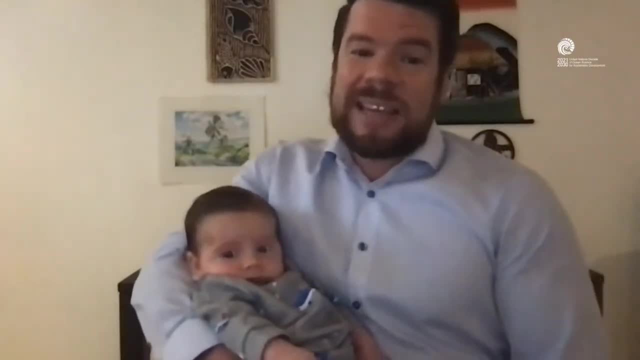 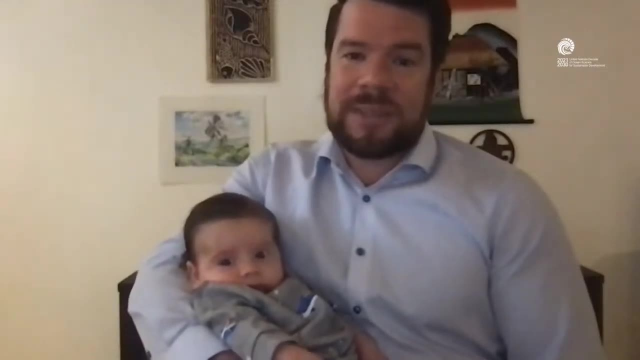 here at the CBD Secretariat. I regret sincerely that I can't be there with you in Marseille. I'm sorry, Thank you, But staying home is also a great opportunity due to the pandemic and I greatly appreciate the opportunity to address this event remotely. 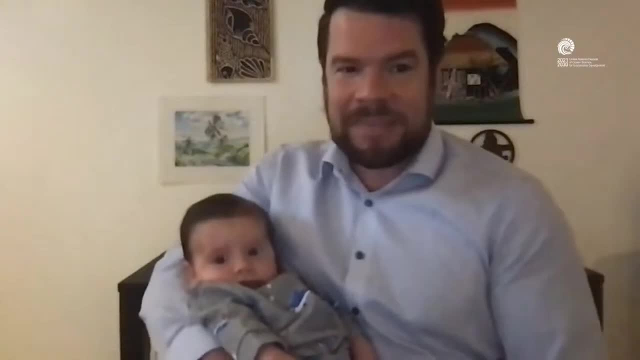 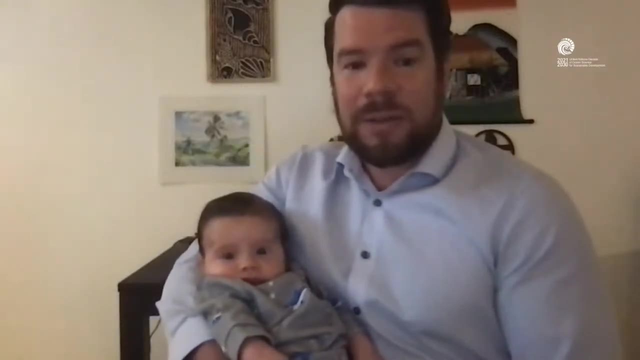 But staying at home also gives me more time with my newborn son, Lionel. In addition to a newfound appreciation for sleep, Lionel's arrival has also deepened my desire to keep the ocean healthy and well functioning for him and future generations. Under the CBD, our parties and stakeholders are working together to do just this for biodiversity. 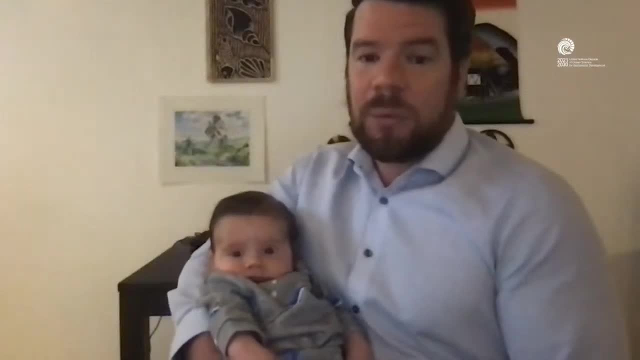 through the development of the post-2020 global biodiversity framework biodiversity framework. This framework, which will be submitted for adoption at CBD COP 15 next year, will contain a new set of global goals and targets for biodiversity. The lack of up-to-date information on the status and trends of 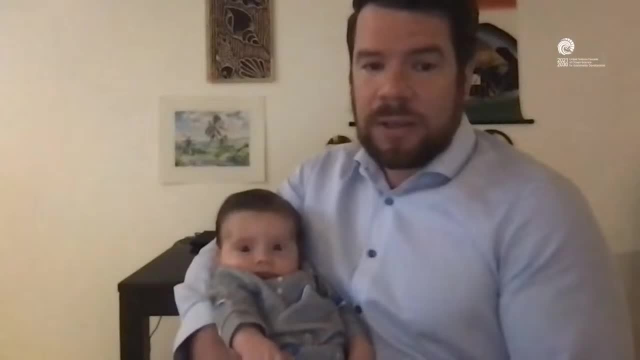 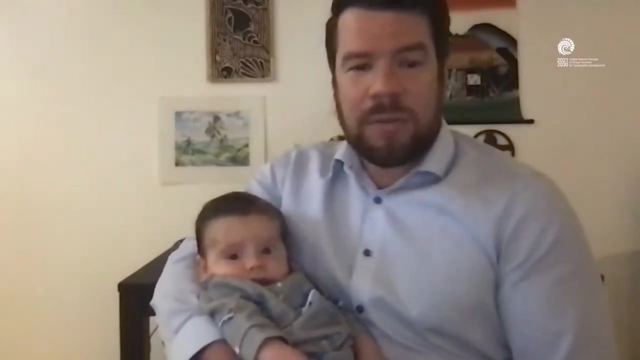 biodiversity was a primary contributor to the failure to fully achieve the Aichi biodiversity targets, and nowhere is this challenge more pronounced than in the ocean. The fact that the launching of the UN Decade on Ocean Science coincides with the development of the post-2020 framework provides us. 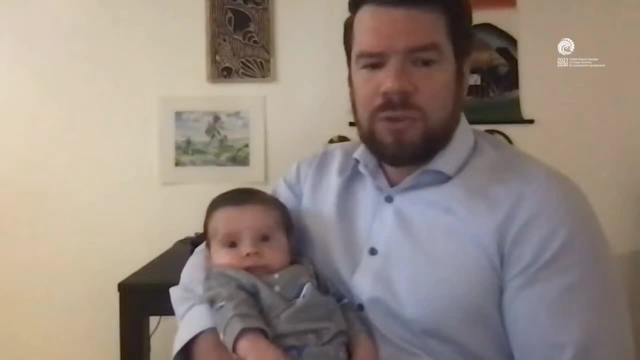 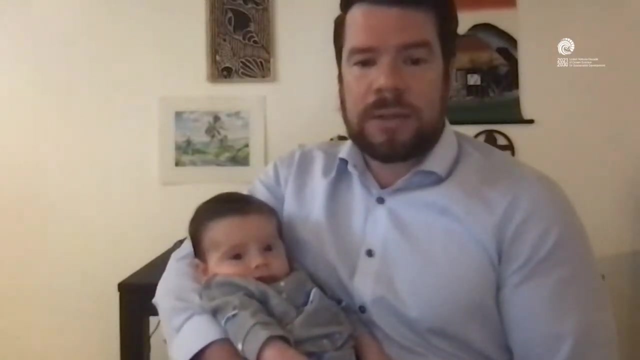 with perhaps a once-in-a-lifetime opportunity, to address this challenge, to further break down silos among our different areas of work and to catalyze synergies to get the ocean data that we all need. This is crucial not only for setting strong goals and targets, but to carrying these into reality through. 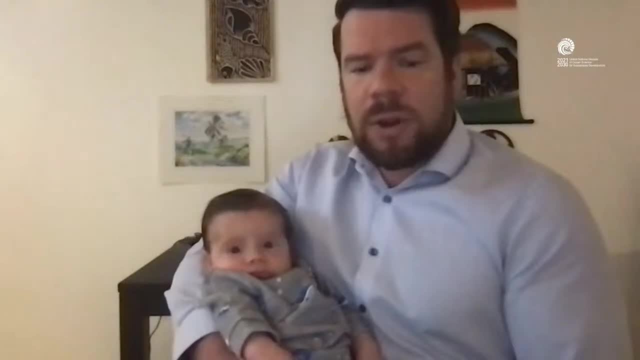 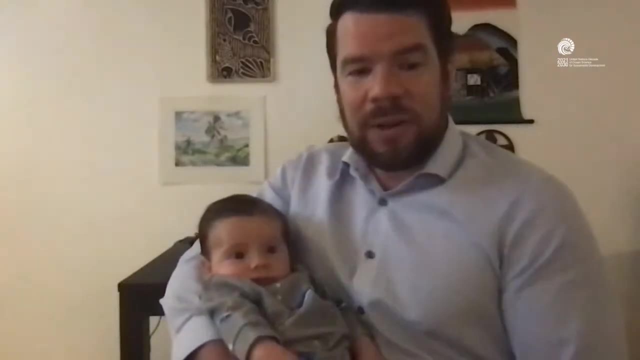 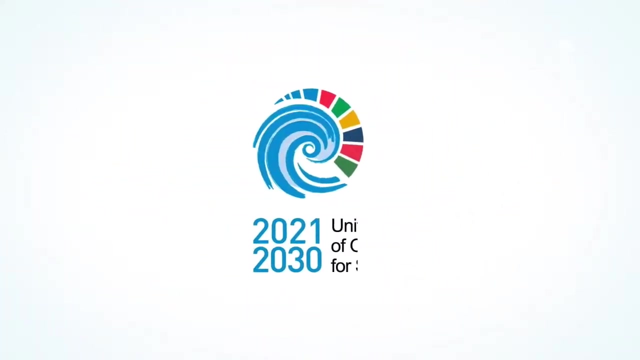 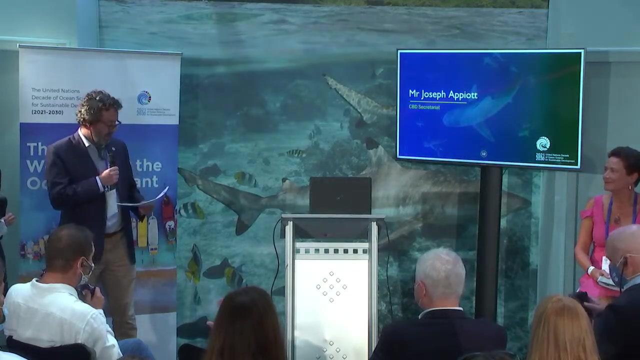 implementation And to understanding whether our efforts are moving us in the right direction or not. With that, Lionel and I will pass off to our good friend, David Obura, and wish you all a productive meeting. Say bye-bye, Okay. thank you very much, Joseph and Lionel, for this very nice message. Certainly, we 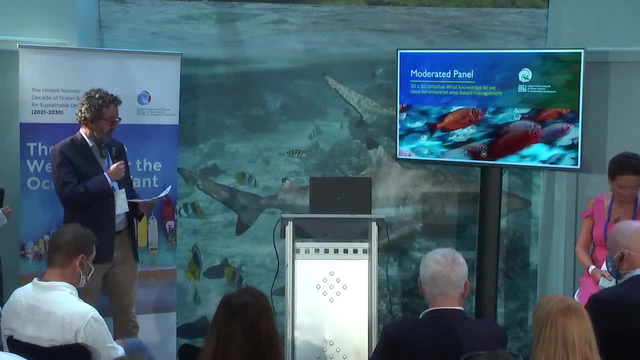 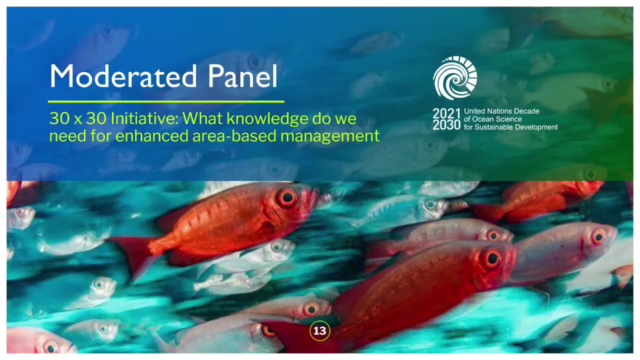 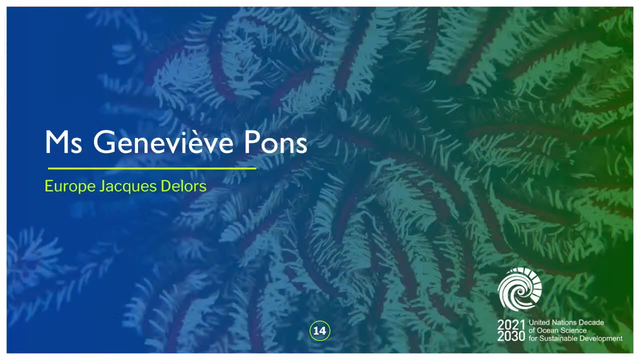 look forward to working with the CBD in the coming months in supporting the, the, the agenda and really trying to see how the science can really deliver the right tools for conservation. Now we are going to be going to our next speaker and we're going to talk about the 30 by 30 initiative, which is a global initiative. 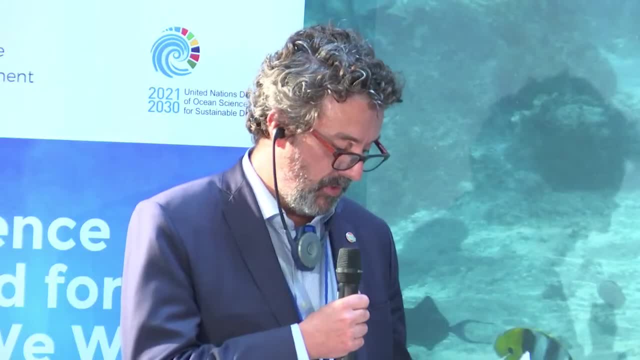 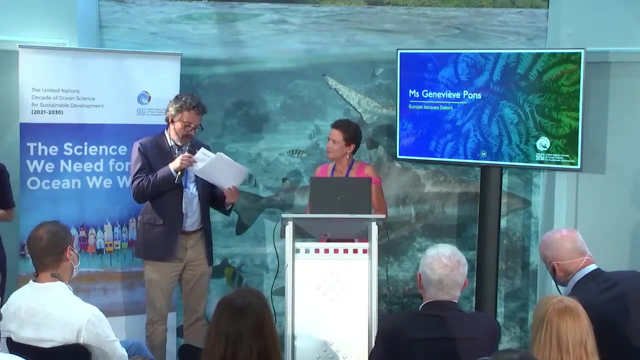 about conserving 30% of the ocean areas And, in particular, the theme of what knowledge do we need for enhanced area-based management? So it's my pleasure to invite Genevieve Ponce, who is the director general and vice president of EGD Europe, Jacques de. 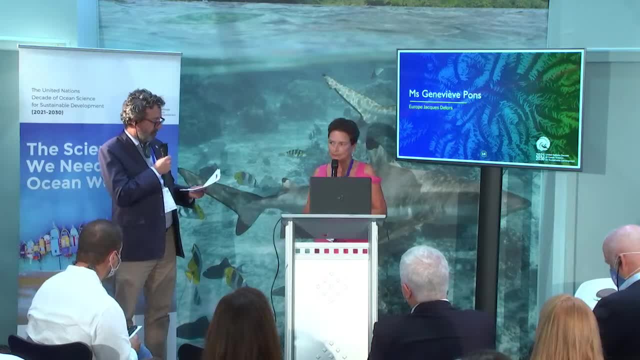 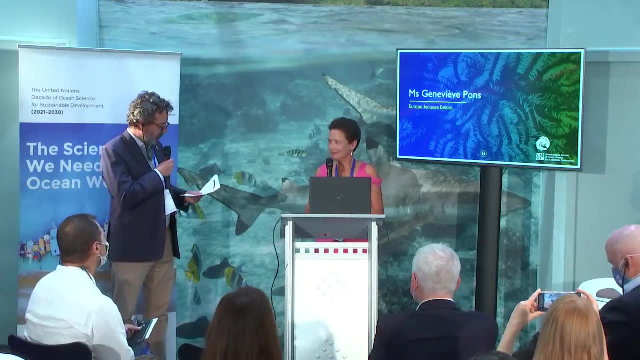 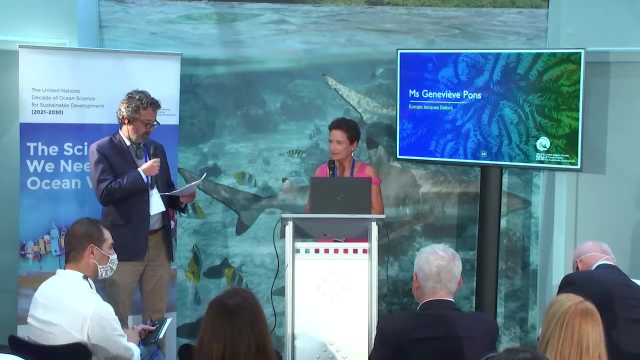 l'Or. She has been part of Jacques de l'Or's cabinet in the in the 90s, being a climate and environmental advisor, Had taken several positions with UN and NGOs, and now, as of today, she's been appointed as the head of Europe, Jacques de l'Or's and which is the latest, 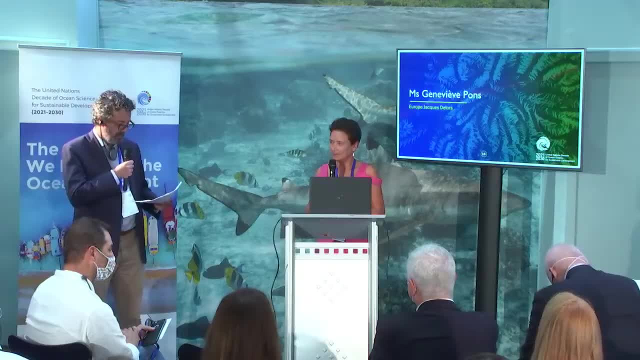 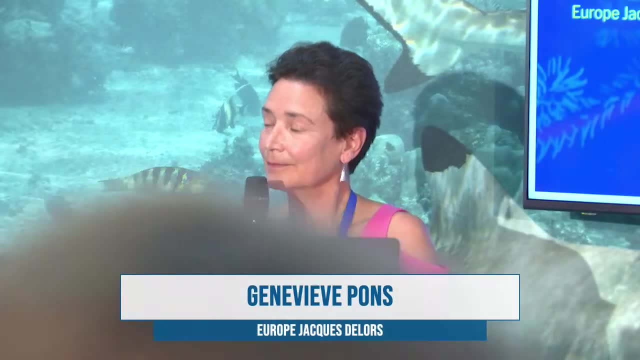 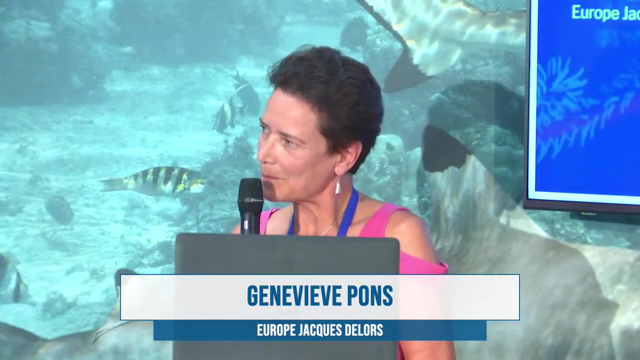 in the family of think tanks carrying on Jacques de l'Or's European vision. So welcome Genevieve. my first question is: could you please give us a bit of an overview of this 30 by 30 initiative and, in particular, how does it actually link with the real CBD agenda? 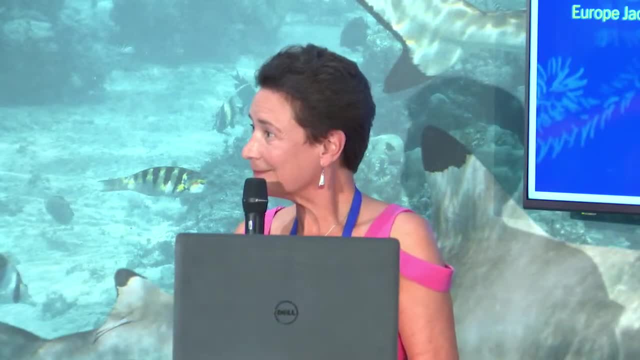 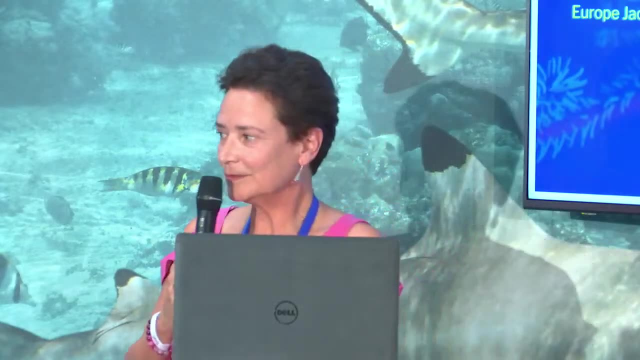 but also the BBNJ process, And maybe you can give us some example of what's happening in the Antarctic, where we already heard quite a bit about this today. Thank you very much. Thank you very much, Julian, and very happy to be with you today. 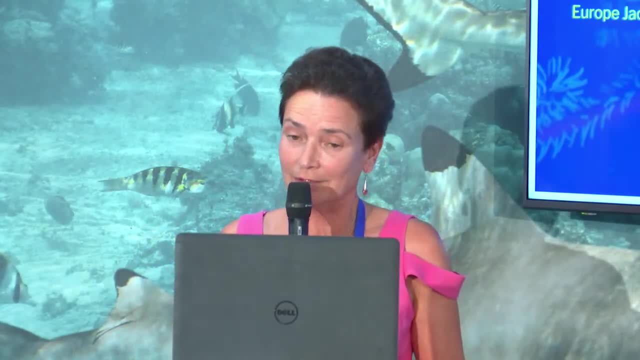 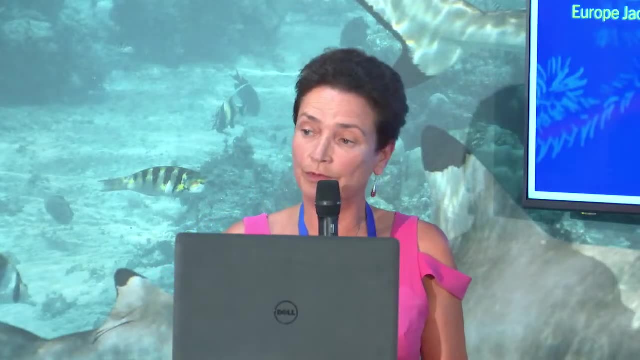 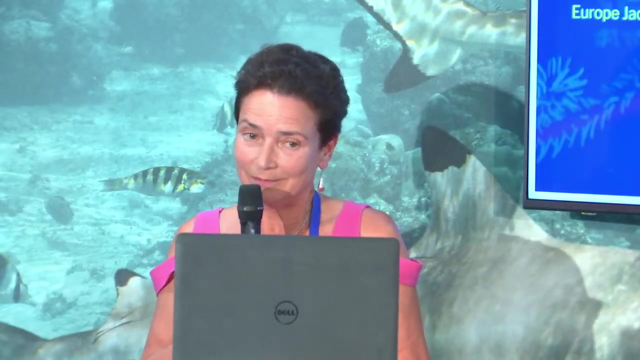 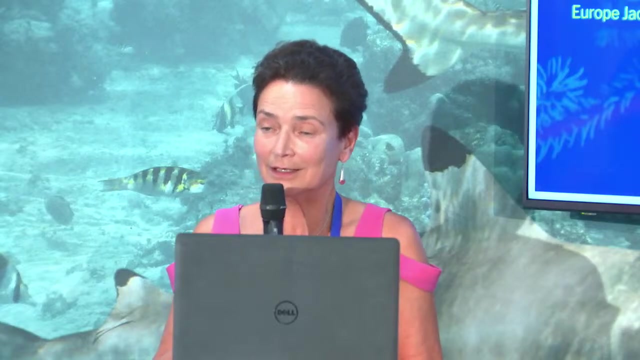 30 by 30 is a call to action to protect at least 30 percent of our ocean by 2030 through the creation of a network of marine protected areas. It is science based. Science and experience show that when you protect a marine area, life is coming back quickly. I am a diver. 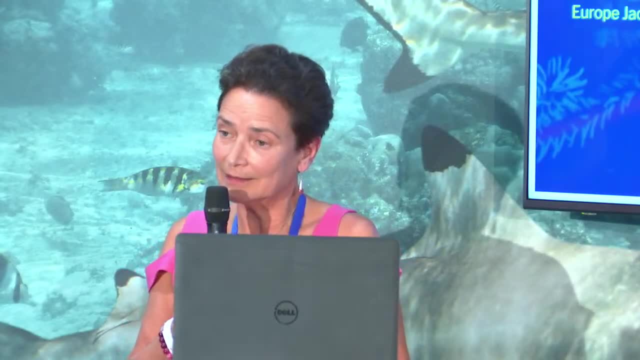 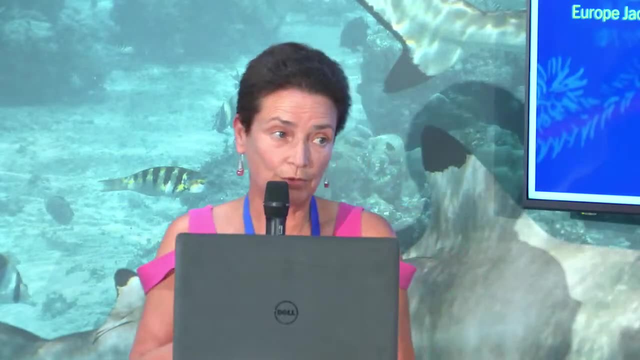 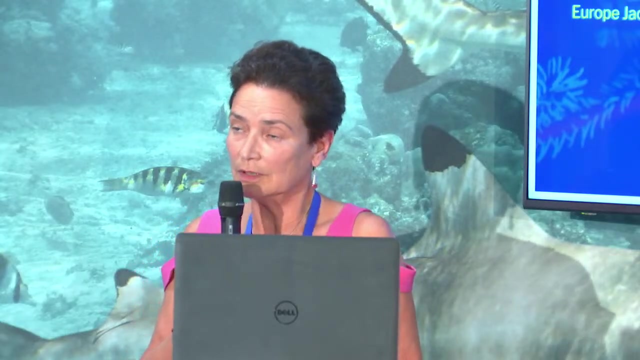 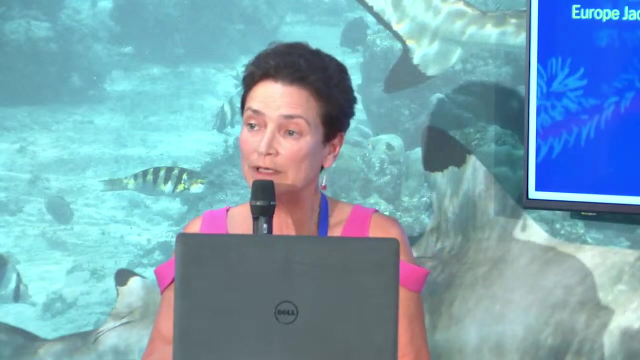 and I've seen with a lot of sadness very depleted areas And then, a few years later, thanks to good protection, they were thriving again And life was coming back, which means not only a benefit to biodiversity but also a benefit to climate, because we know more. and more, the narrow link between biodiversity and climate. Thank you very much. And the rich marine zone has the capacity to absorb carbon and emit oxygen. So this is what it is about. It was launched by a resolution of the IUCN in 2016.. It is now. 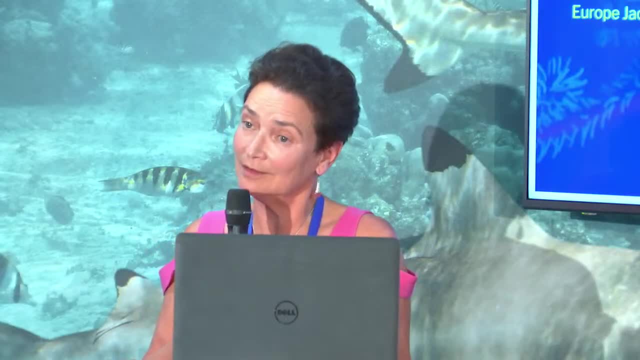 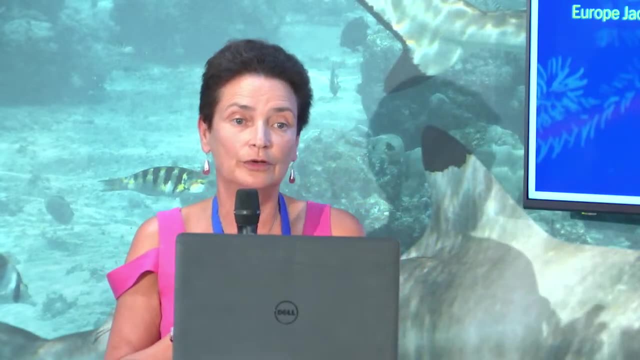 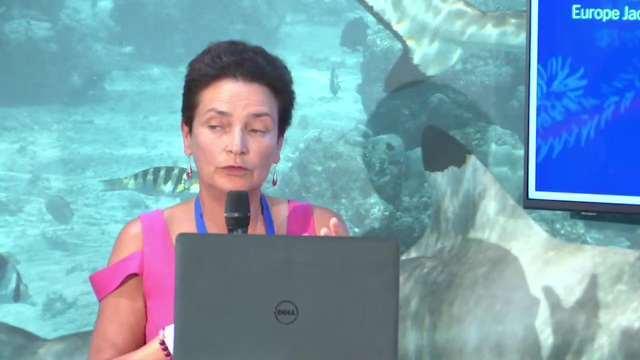 endorsed by nearly 100 states in the world. It has become one of the key targets of the CBD, the Convention on Biodiversity. It is now globally supported, Thank you. and during 135 years of cult bibinjim, it will be healthier. 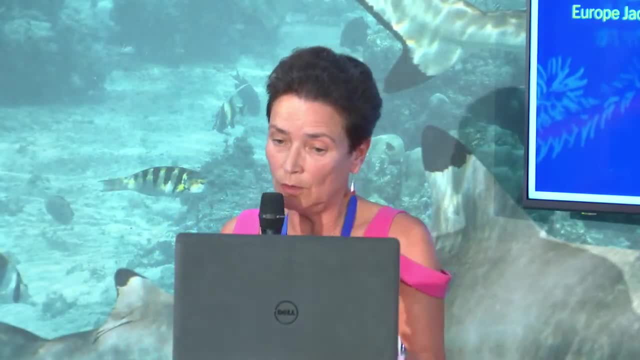 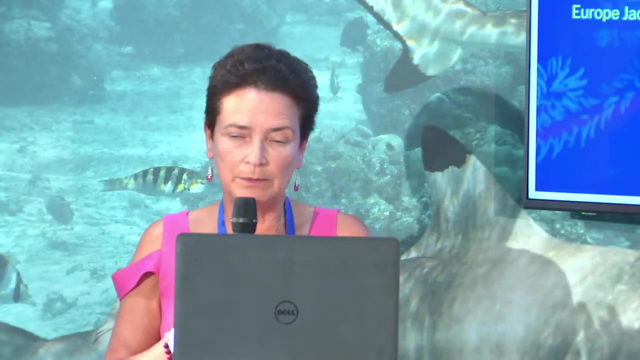 Thank you very much. According to Unreal, Whenever Jim and Misha Greg, I had a question about the project and why did you decide to do it? My question is because you mentioned that before, the yolk actually isn't an oglider. 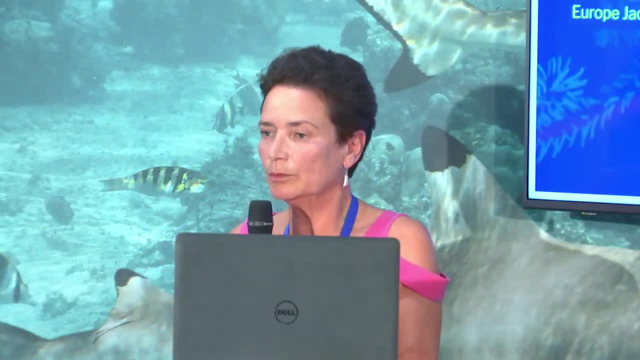 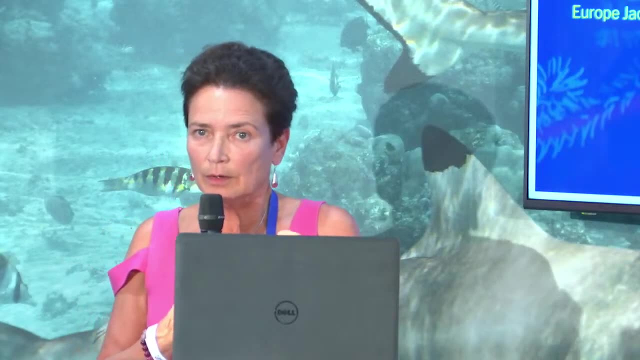 And then there is a deceit of biodiversity. Is that a positive statement? Is it a negative statement about the role energy and carbon is affecting human rights? Well, yeah, it is. It is certainly Yes. It is now being negotiated, and most people don't know that this high sea, which is more 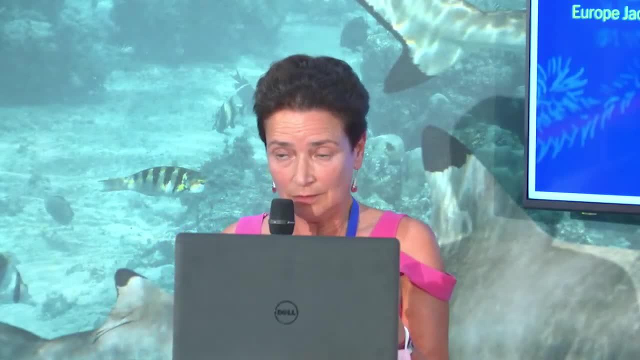 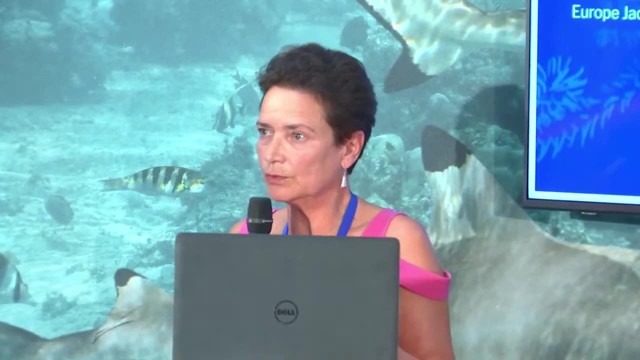 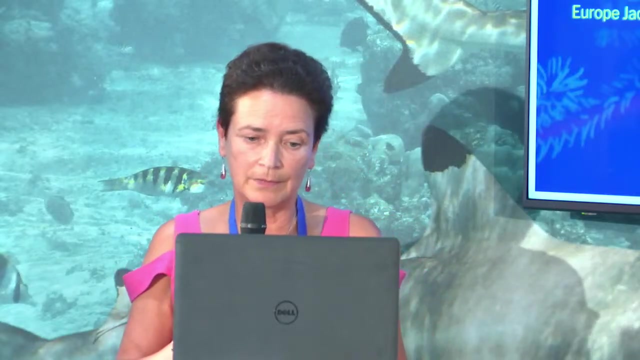 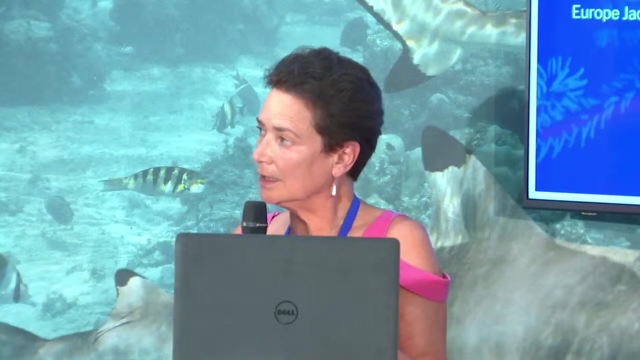 than half of the ocean is not protected. Only 1% of this huge area is highly to fully protected, So there is a lot of work to do and this also will be negotiated in the next month. Finally, it is extremely important for Antarctica. 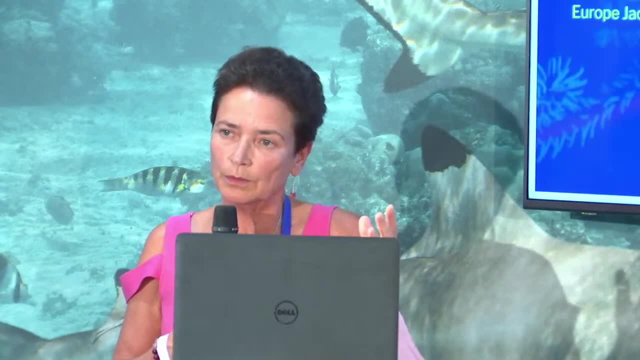 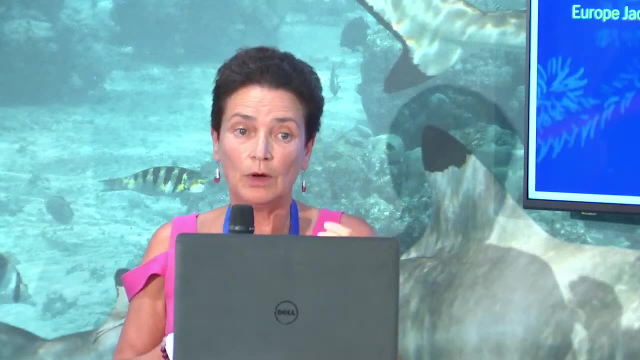 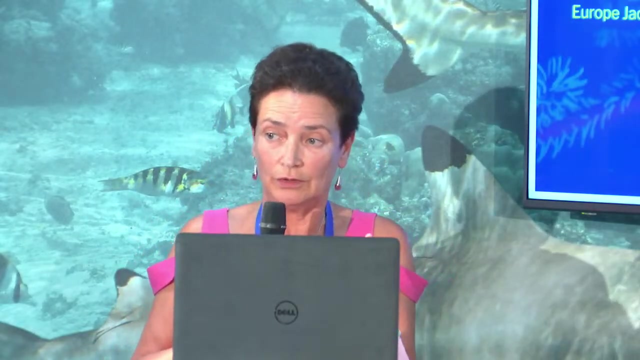 Antarctica is a zone which is very far away, so a lot of people don't know how Antarctica is important for their own life, for our biodiversity, for our climate. Antarctica represents 90% of the ice of the earth, 70% of fresh water. 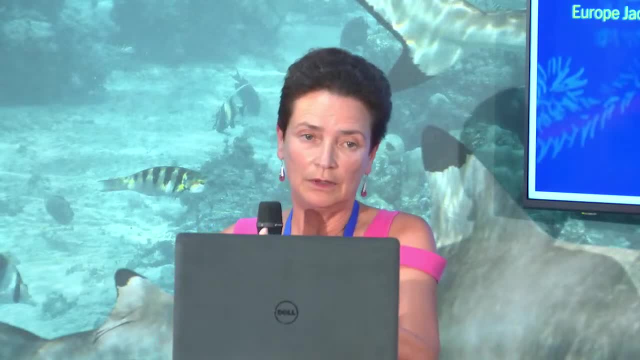 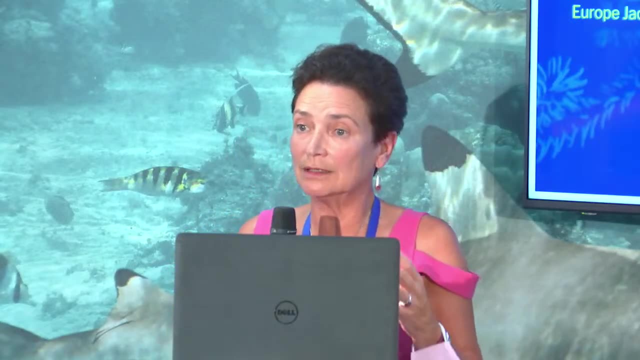 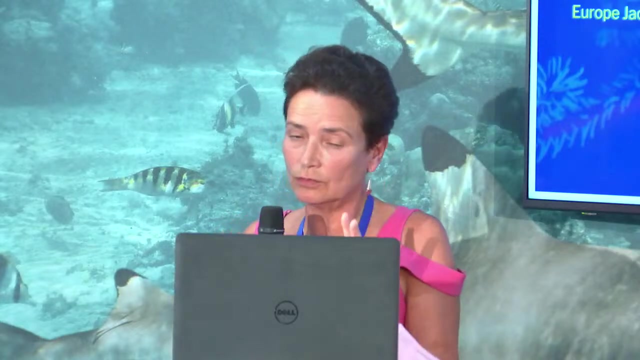 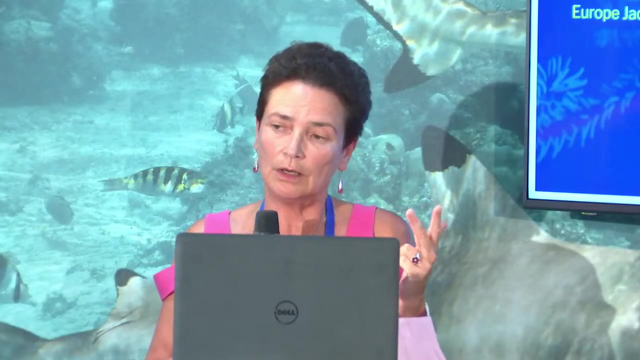 And a very high water content. A very powerful stream is around Antarctica that sends life all around. So we need to protect Antarctica. for our biodiversity and for our climate It is absolutely key. There are three areas that are proposed: One in East Antarctica, one in the Weddell Sea and one in West Antarctica. 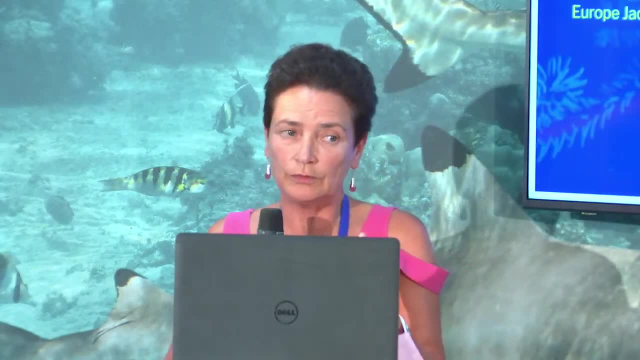 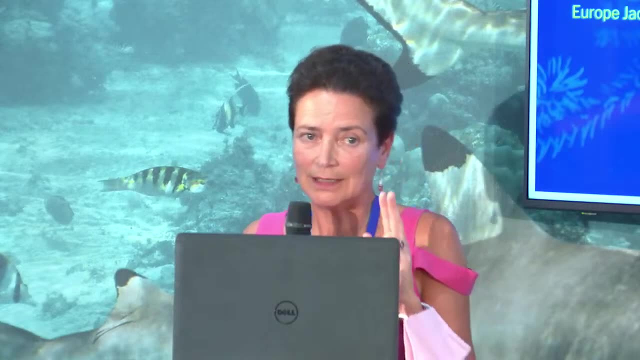 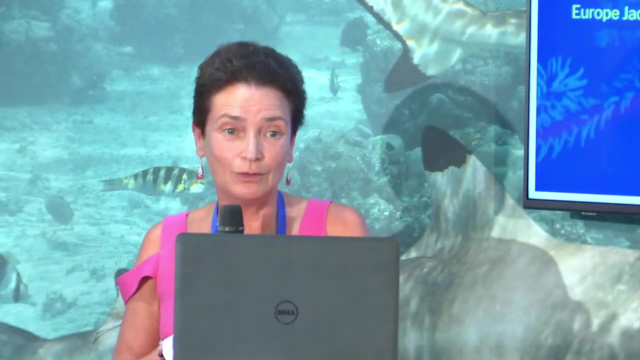 And these proposals are supported by most of the people, Most of the members of the relevant commission, the KAMLAR, except for two, China and Russia, And I had the occasion yesterday to speak with President Macron and tell him that it is now the time to act. 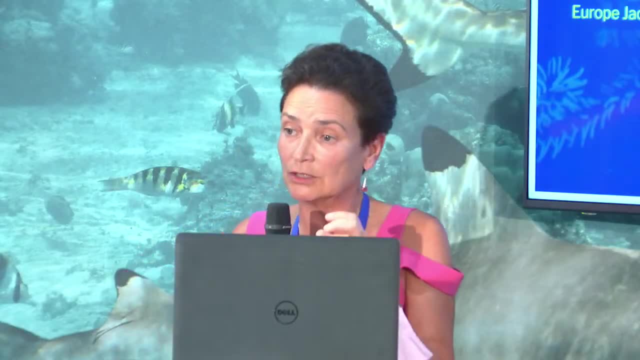 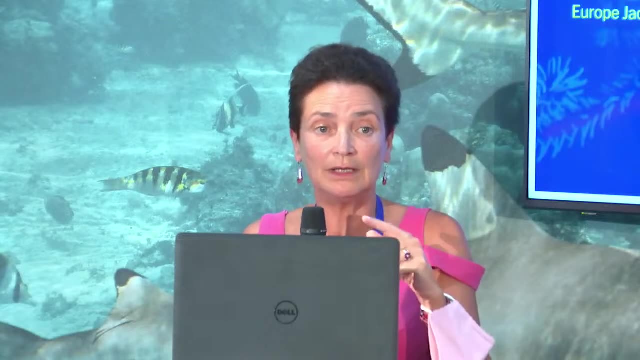 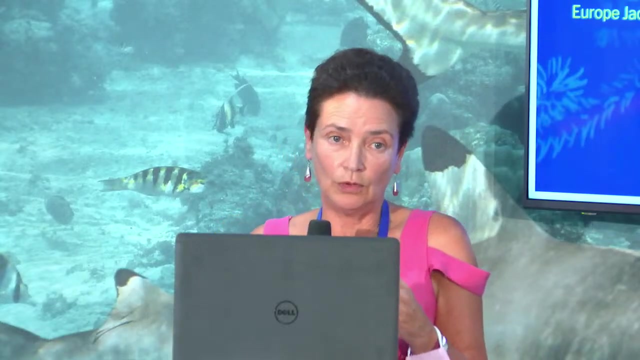 The France, as well as the EU, have been very great supporters of this protection, And now this year will be very special because France will take the lead of the European Union, Giving it even more power, And China will host the CBD Convention. 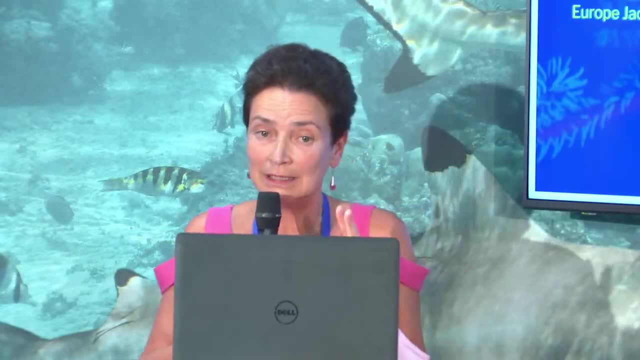 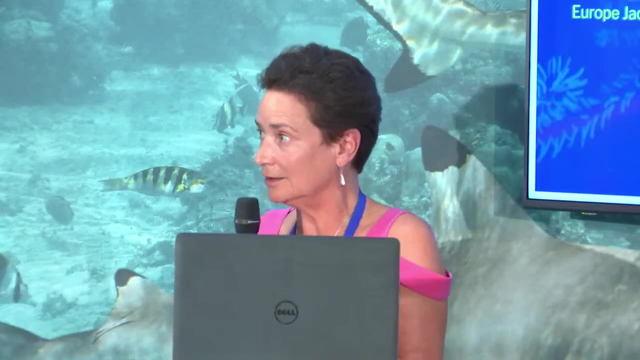 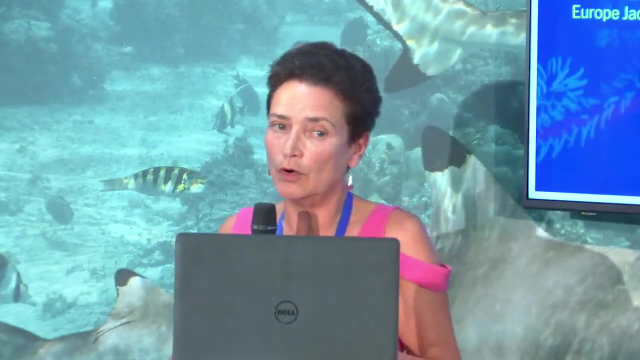 So these are two reasons why this year is absolutely key to get Antarctica protection. And finally, maybe I should say a word about Ocean Unite. Ocean Unite unites many people around the globe for the protection of our ocean And this 30-30 objective- it is at the core of the European Union. 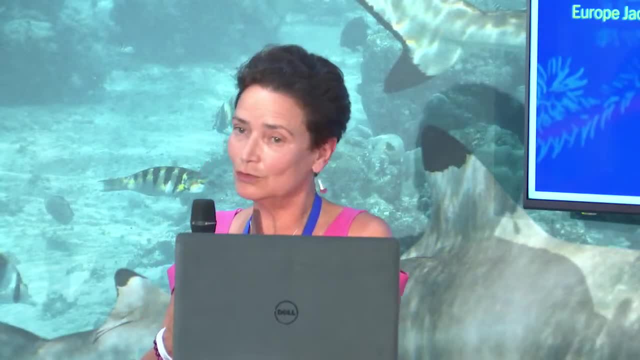 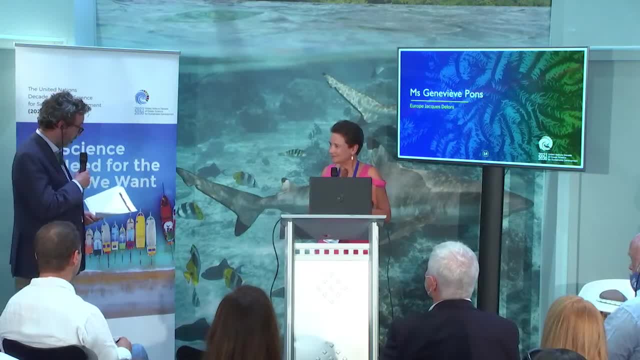 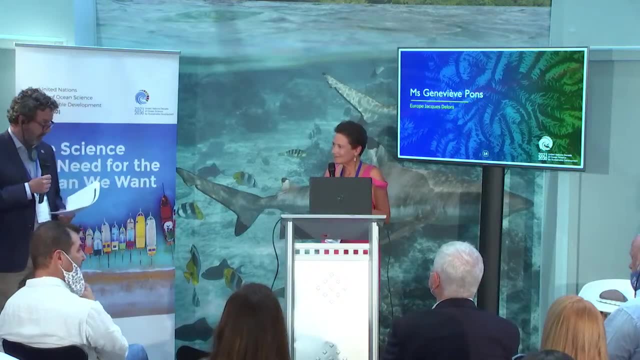 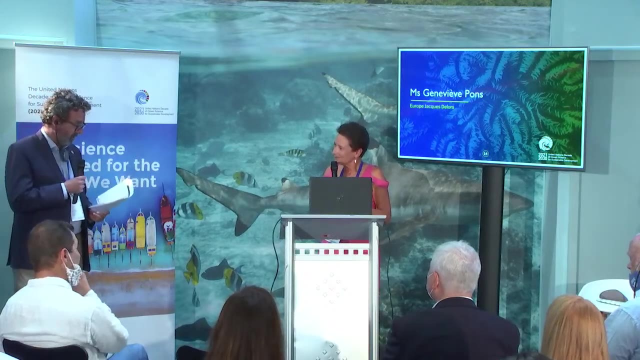 Thank you very much. It was actually quite heartwarming to hear this morning the DJI Environment Commissioner to also call for this target to be achieved. We wish you luck and more than luck, but I hope you will be able to mobilise support. 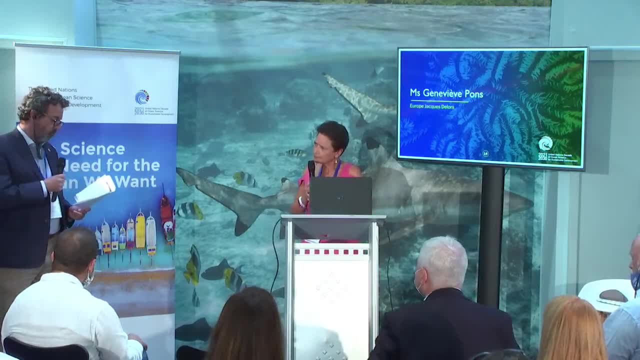 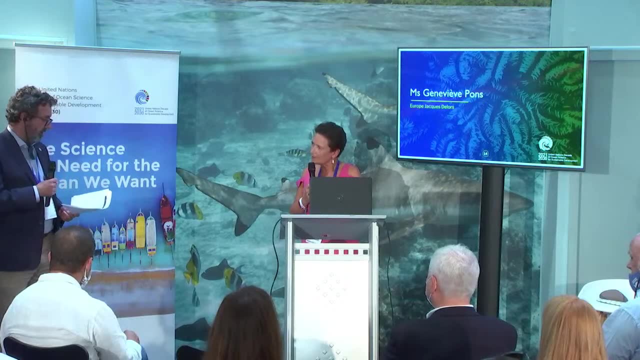 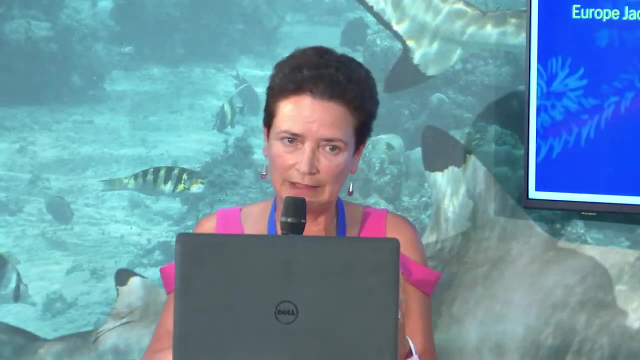 Now, a question I wanted to ask you is: from your perspective, what are the key ocean knowledge needs that are required to achieve this target? can you say maybe a bit more about this? well, I would say that there are some countries that are not able, that have 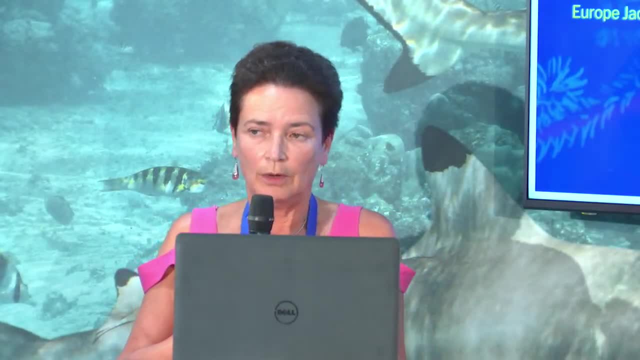 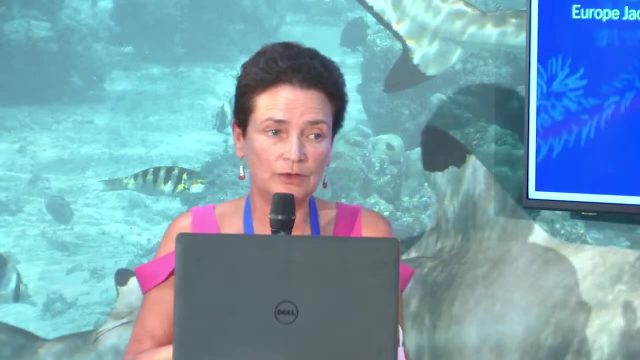 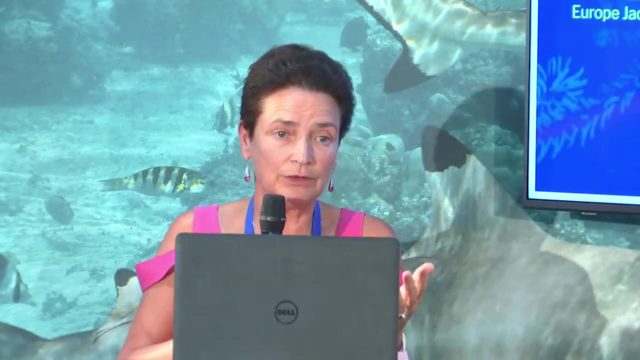 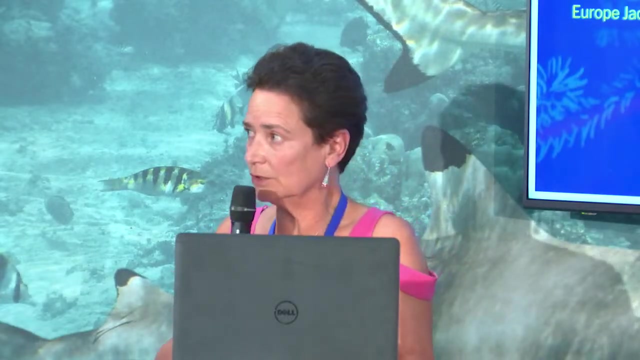 not the capacity to know what biodiversity is in their waters. they have not this capacity, so international cooperation could help them identify the areas in their marine territories that should be protected. this is the first link between knowledge and protection. then I would like to take once again the example of Antarctica. Antarctica has been made a continent for science and peace by the treaty- Antarctic Treaty- which was signed in 1959, and through the protection of this area we can gain a lot of knowledge and we have. there is a specificity, there are many specificities concerning Antarctica. it is far away. it is very difficult to 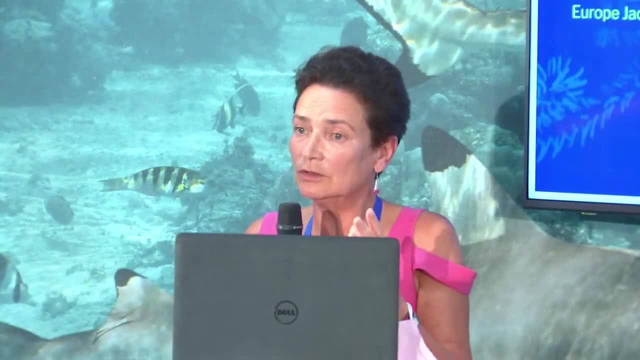 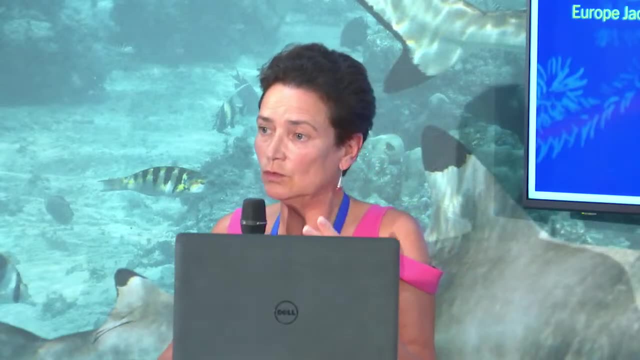 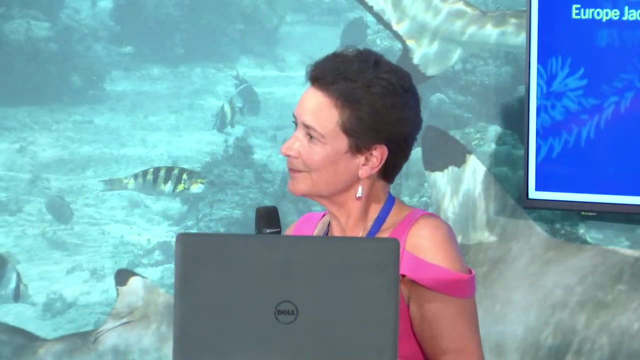 get there. it is very costly to get there, and so international cooperation is particularly important to not only get there, but to have common science coming from this part of the of our common planet right, thank you very much. India will take on some questions later on and again remind the audience that we'll 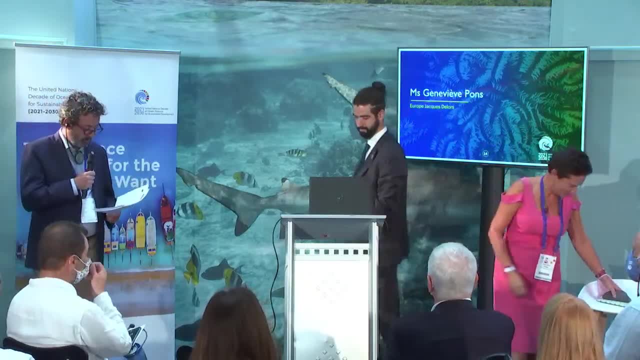 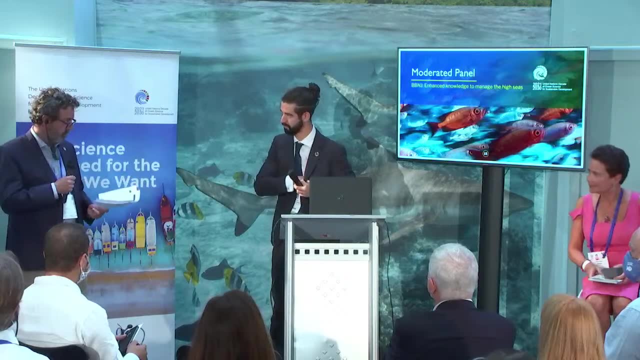 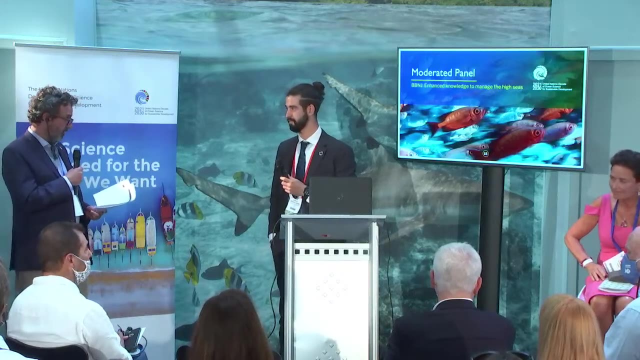 have a bit of time for live question as well as a question on slido now. the next segment is focusing on how to enhance knowledge to support the high seas conservation and management. we have an international negotiation which has been 15 years in the making. hopefully we will get a critical step next year in terms 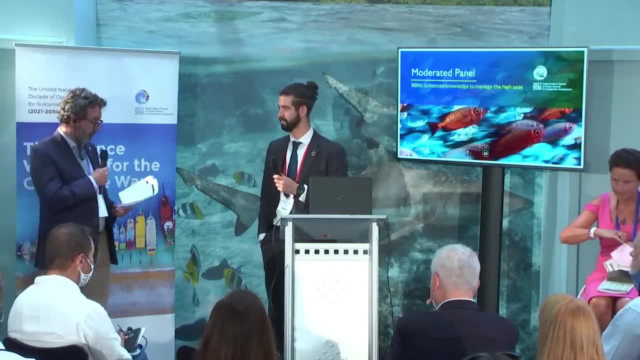 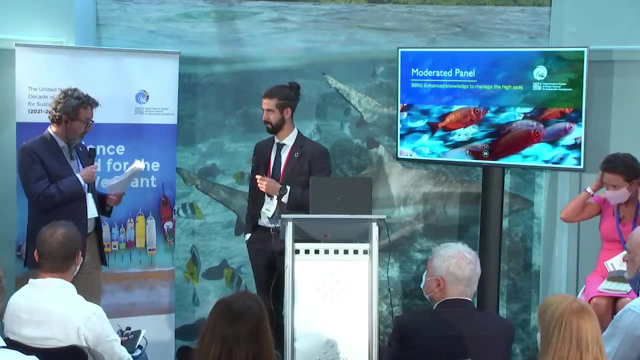 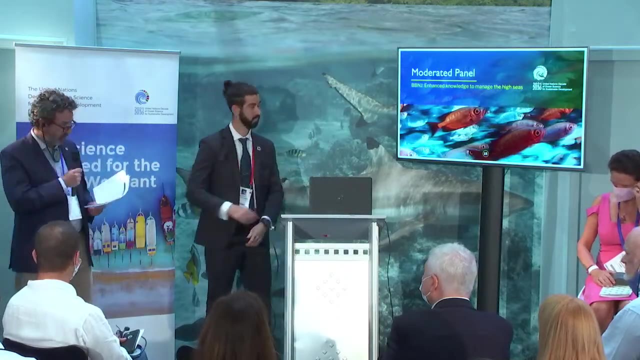 of getting the legally binding agreement for the conservation of the high seas. but what do we need for in terms of a sign? do we have the right scientific and technical mechanisms to advise the implementation of such treaty? before we go to you, Guillermo, we'll just gonna hear very briefly from one of our 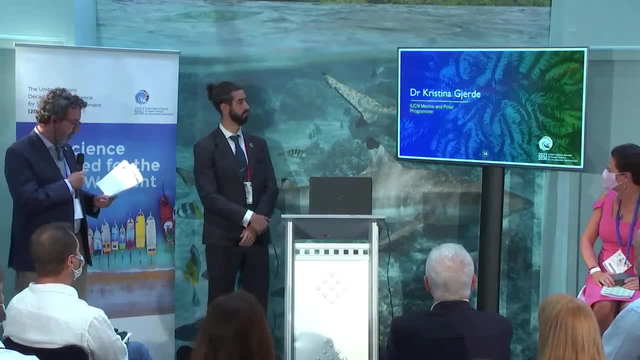 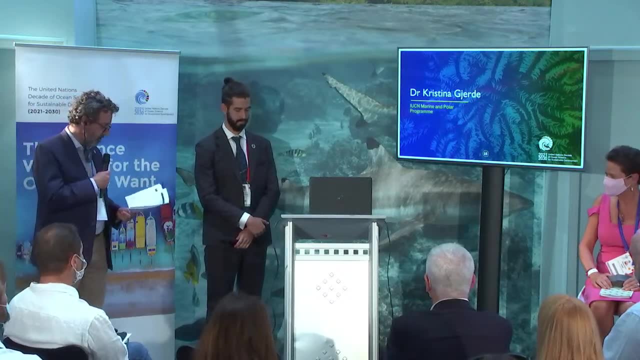 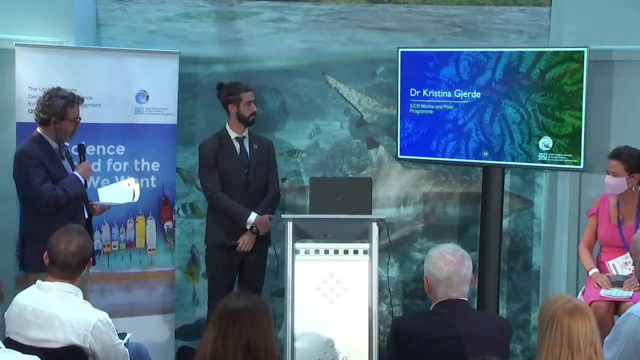 IUCN colleague, Cristina Gierde, who is a senior high seas advisor to IUCN's global marine and polar program. she's been the voice of IUCN in the BBNJ negotiation and she also sits on the decade advisory interim advisory board that's been helping in in preparing and implementing the decade. so 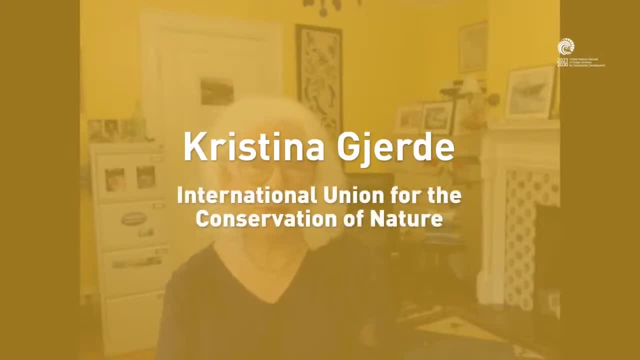 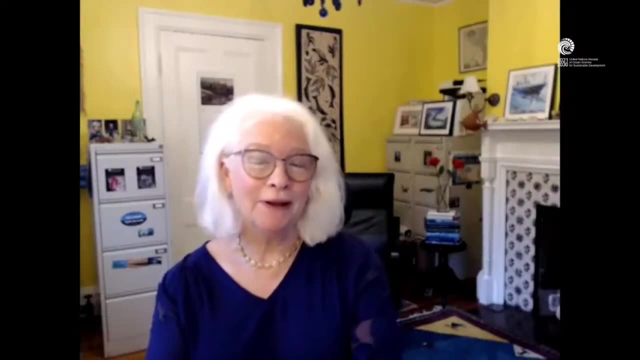 let's hear from Cristina greetings. United Nations State decade of ocean science for sustainable development offers a vital opportunity to collectively ensure that decisions on how we use, protect and manage two-thirds of our planet are based on the science, knowledge and indeed the humility we need in the face of a rapidly changing 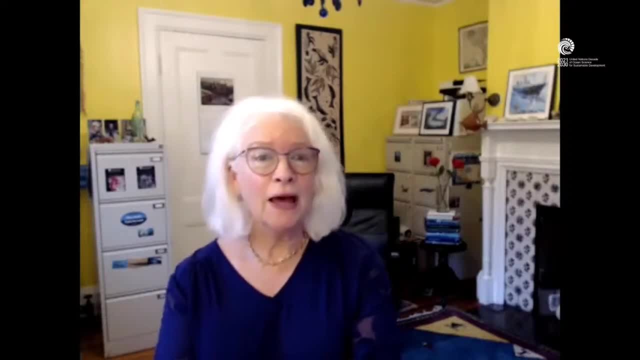 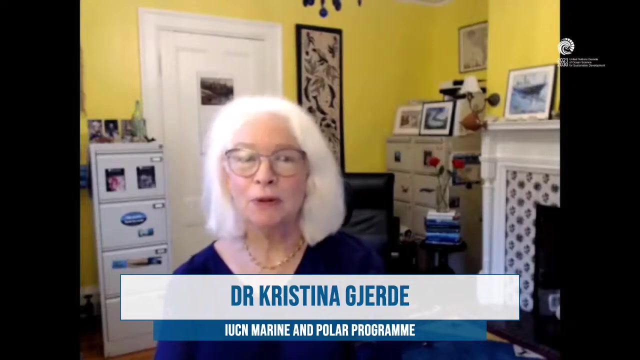 ocean. the ocean decade is well-timed to also support the evolving UN treaty for the conservation and sustainable use of marine biodiversity in the 60% of the ocean that lies beyond national boundaries. core components of this treaty will be conservation tools such as marine protected area networks and. 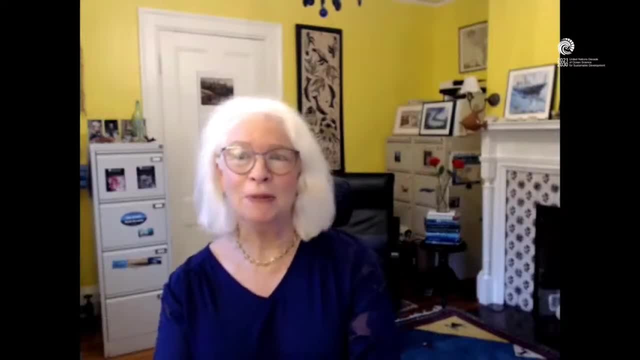 connectivity corridors. environmental impact assessments that reflect an understanding of direct, cumulative and climate change effects. equitable access and sharing benefits of marine genetic resources, combined with capacity and transfer marine technologies to enable all to equitably participate. thus the BBNJ agreement and the UN decade of ocean. 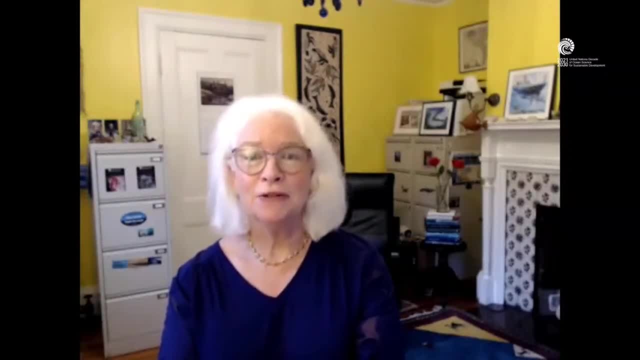 science are mutually supported and, indeed, interdependent. for this reason, I urge all with a stake in ocean health to join in crafting robust decadal research projects and research projects that are, and promoting an ambitious high seas treaty, For both are essential to safeguard our shared global ocean commons. 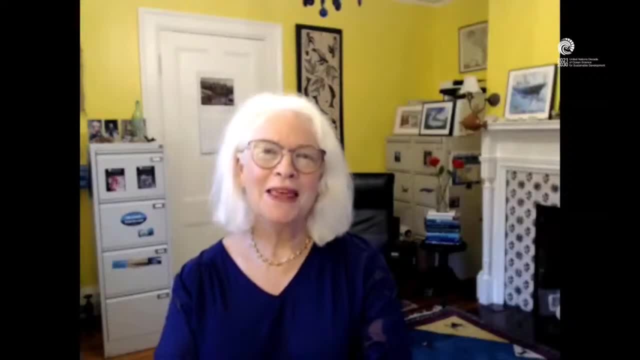 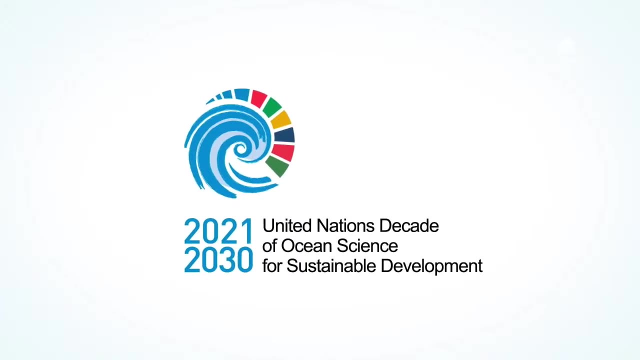 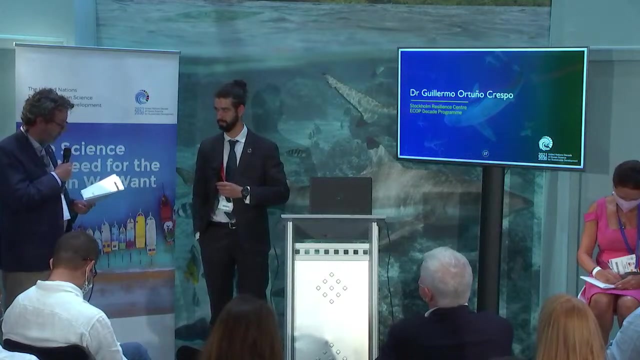 for the benefit of present and future generations. Thank you very much. Now let me go to Guillermo Ortono Crespo, who is a marine ecologist with a doctorate from the University. He now works at the Stockholm Resilience Centre. 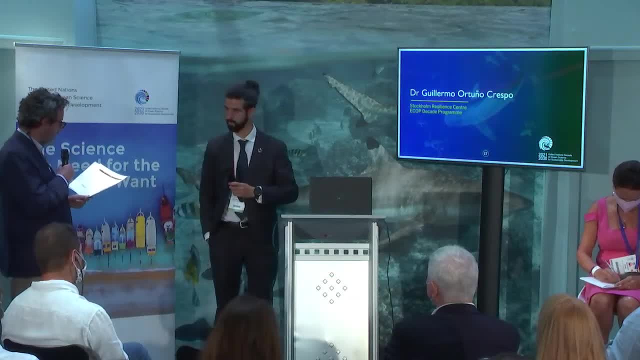 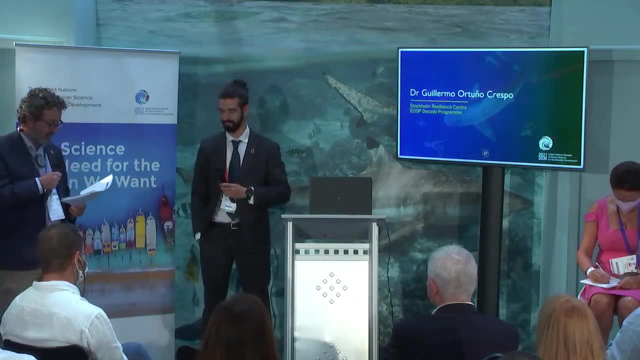 And, of course, Guillermo has been a member of the Early Career Professional Programme of the UN Decade, I would say from the start. basically, You've been one of our founding members of that excellent programme. So, Guillermo, can you tell us a little bit about what are the critical missing pieces of information? 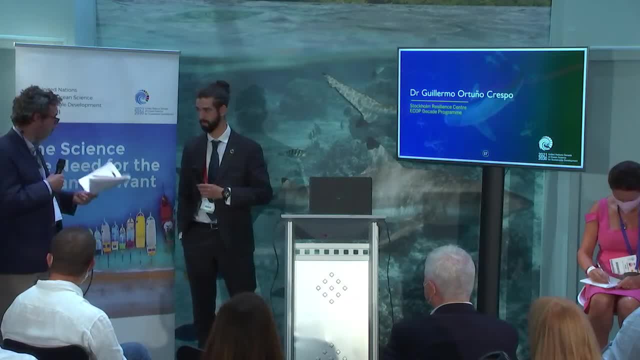 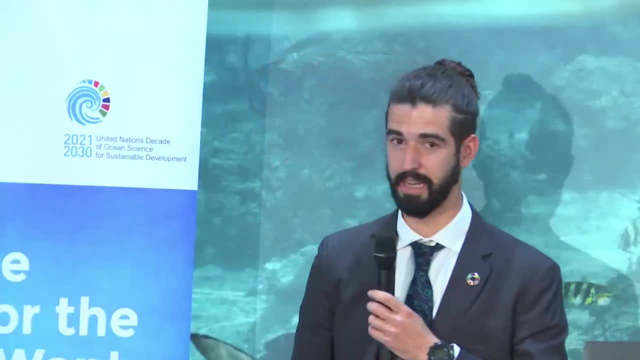 and knowledge when it comes to the BB&J that are going to be somehow defining the scope of this BB&J agreement. Certainly, Hello Julian and hello everyone. I'm assuming Christine has provided some inoculation of BB&Js. 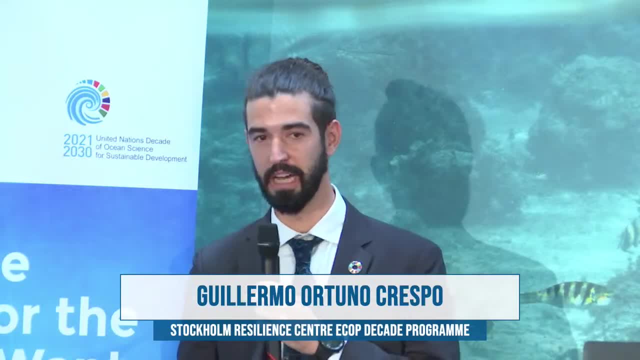 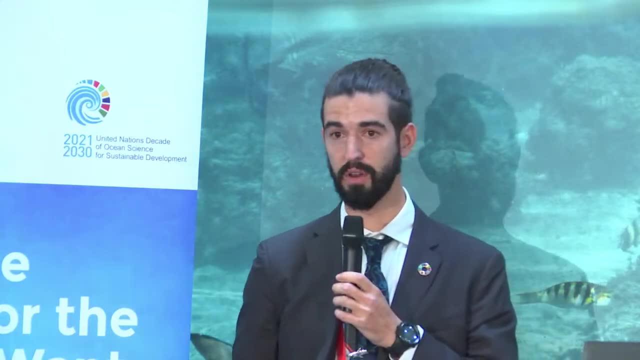 so you might be familiarised with some of the elements of the new treaty. If you're not. there are four elements, two of which are quite data intensive. I would say We have one of the pillars of the BB&J treaty that focuses on environmental impact assessments. 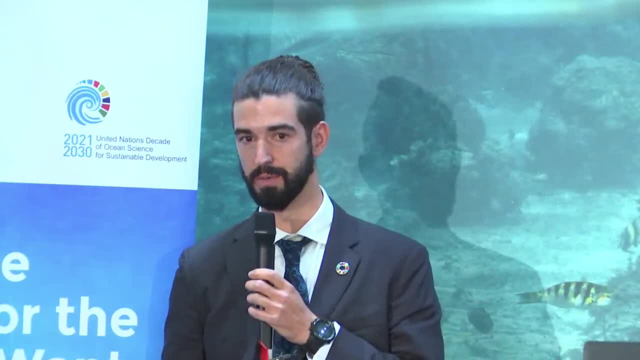 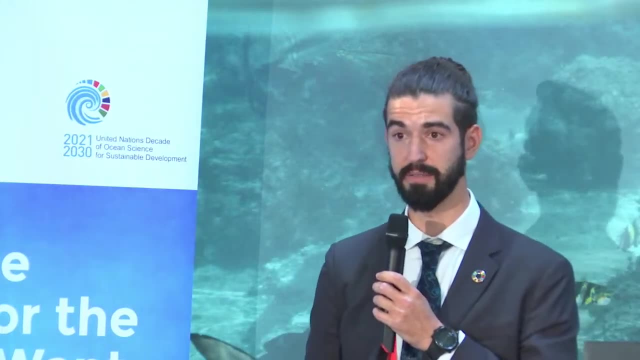 and the other one focuses on area-based management tools. I'm a spatial ecologist by training, so the area-based management tool portion of the treaty is very dear to me. I've spent lots of hours trying to figure out what we need to know about the spatial and temporal distribution of biodiversity. 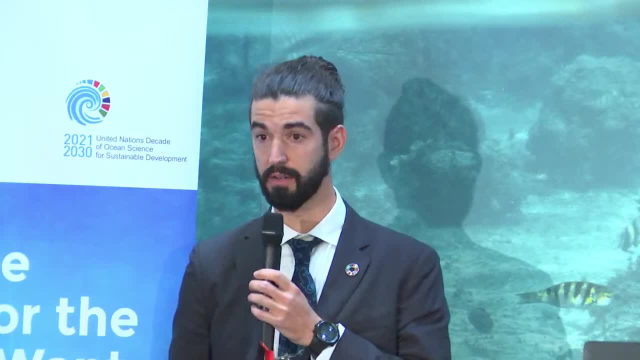 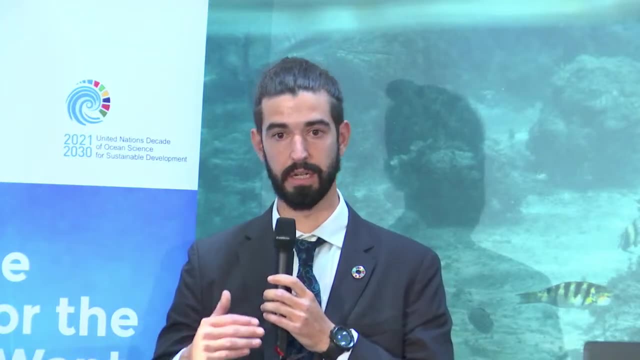 in order to protect it. The treaty comes at a critical time. as human beings, we're expanding further and deeper into the ocean than ever before, The depth at which we're fishing both pelagic and demersal gears. we're going deeper to catch different species across the food chain. 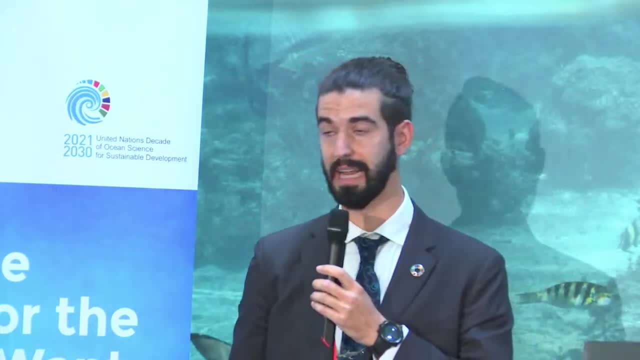 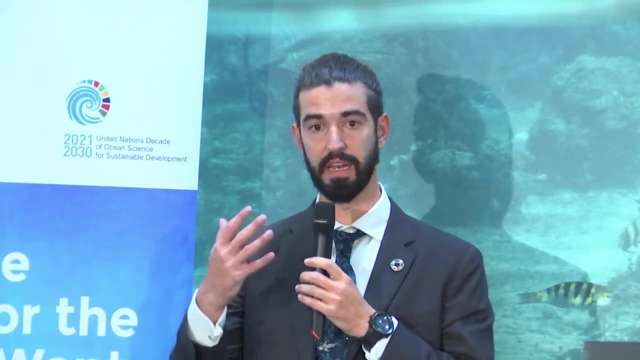 One thing that we have not done a good job at doing in this last 70 years of expansion is documenting what we're catching. We don't have proper baseline information, so this new treaty is filling a governance gap that the law of the sea left behind. 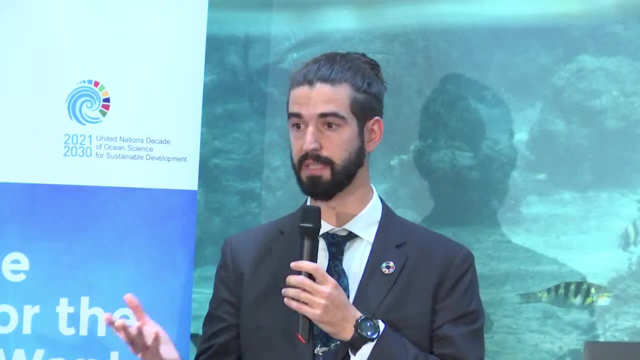 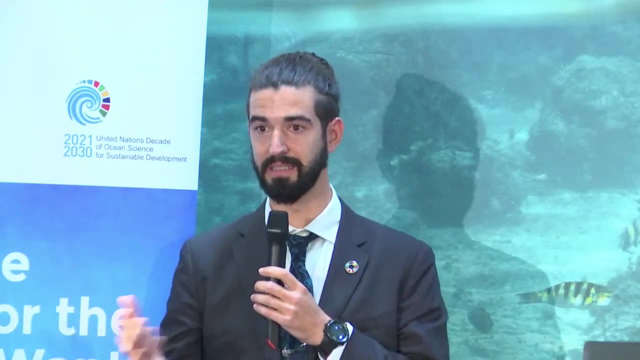 We don't have a mechanism, an official mechanism, to establish area-based management tools in the high seas. But now that we're creating one, the question is: do we have enough knowledge across sufficient species, in space and time to implement these measures? 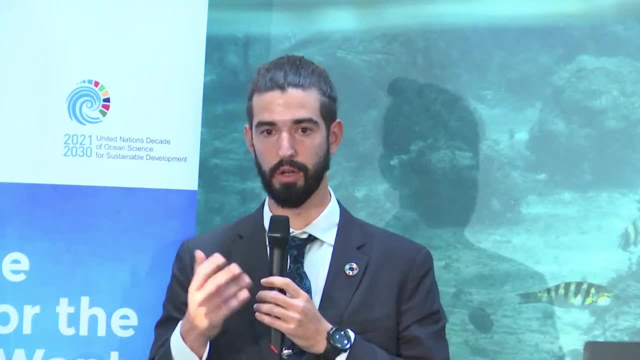 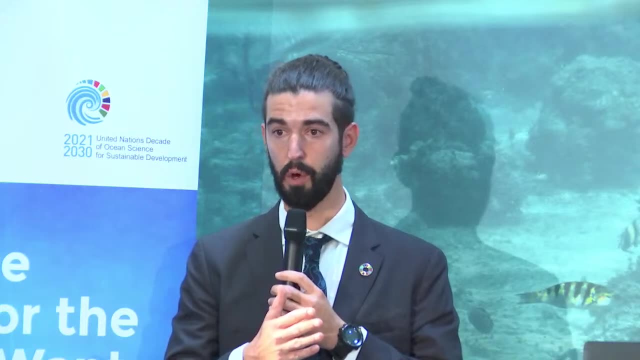 I am finalizing a study together with colleagues at Duke University, University of Queensland, supported by IUCN, I should say, that uses data from the Ocean Biodiversity Information System housed at UNESCO. They host the most comprehensive repository of high seas data in the world. 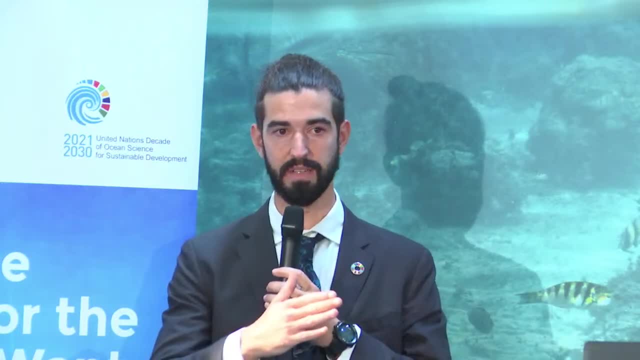 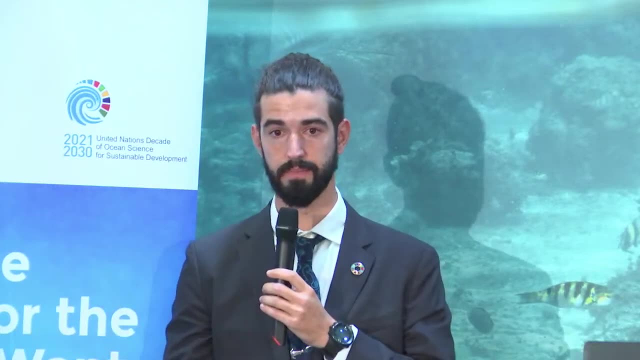 over 6 million records and we analyze that to see what the spatial, temporal and taxonomic distribution of data is. We do not have enough knowledge in the high seas, Not even close. We do have 6.2 million records. 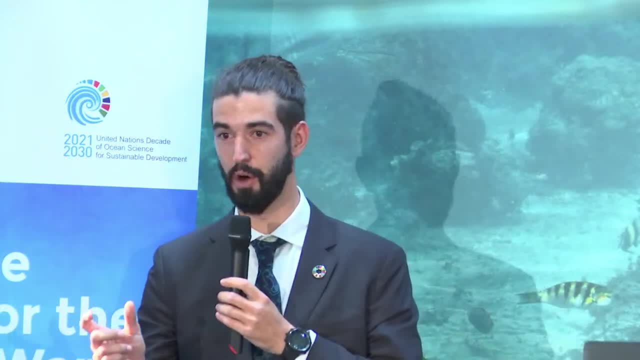 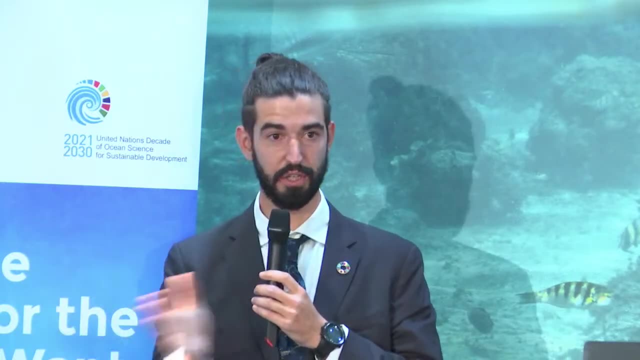 10% of the species account for 62% of all the data. The top 0.1% of species account for 40% of the data. It's very skewed taxonomically to the species that we know well, some in the Southern Ocean, some in the Northeast Atlantic. 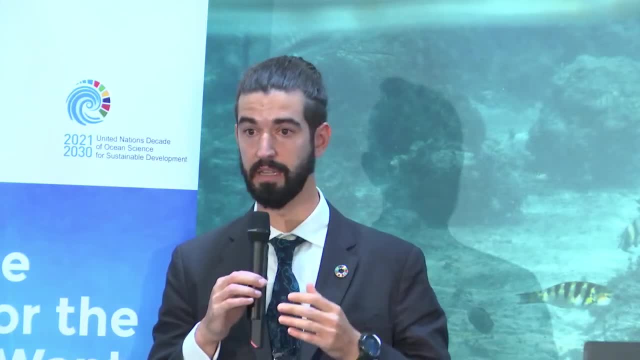 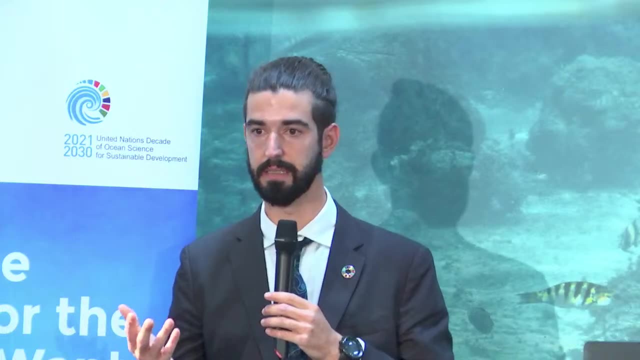 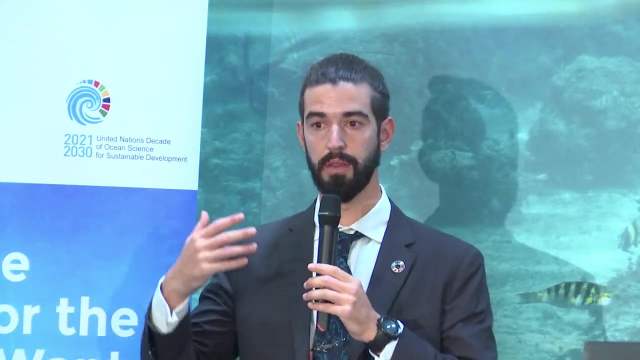 Geographically, we have huge, huge gaps in the tropics, in the Pacific, and most of the data that we know come from pelagic species. Quite surprisingly, we are not doing a good job at bringing data connecting data streams. OBIS doesn't have access to data generated by RFMOs, for instance. 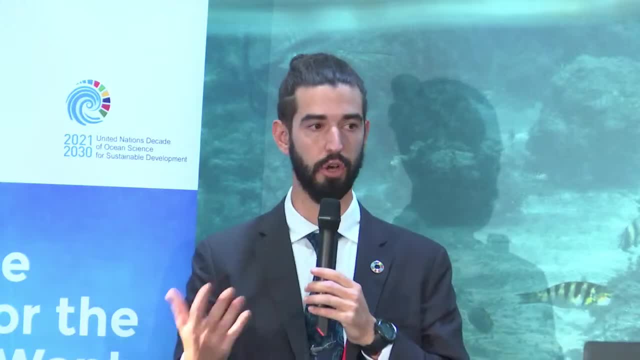 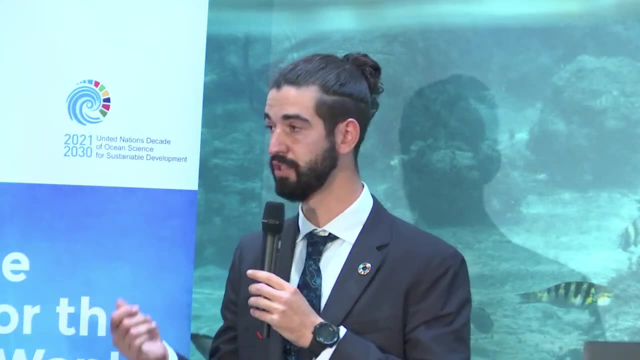 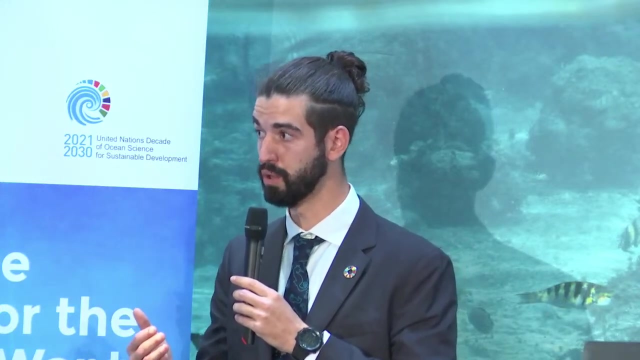 So there's an opportunity through the Ocean Decade not only to generate new knowledge, but to encourage national governments to share whatever knowledge they have. The answer is no, I'm afraid. I don't think we have enough data to even consider establishing comprehensive air-based management tools in most of the high seas. 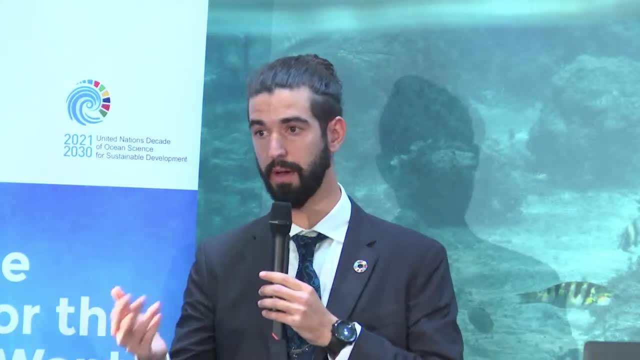 Now some folks might say: the Northeast Atlantic- we do have data. or the Southern Ocean, or the Antarctic Peninsula, we do have data. So we don't have enough data. We do have hotspots, But for the most part, unfortunately, we do not. 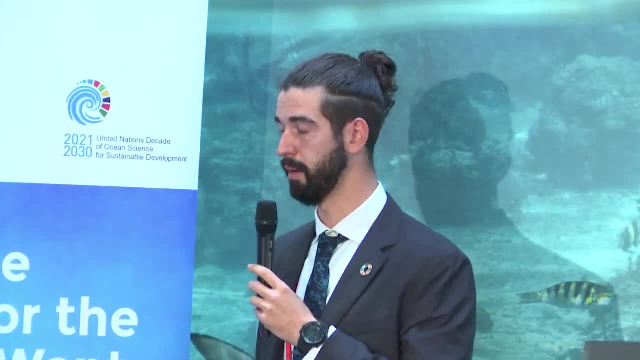 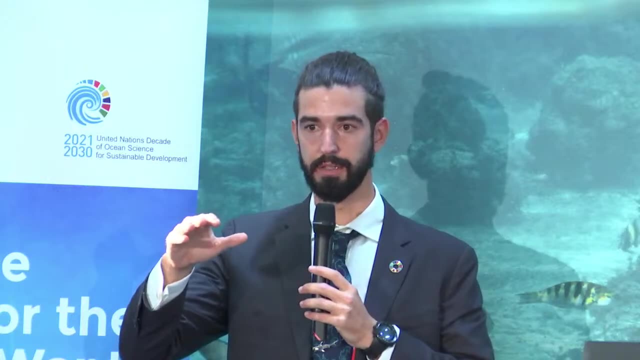 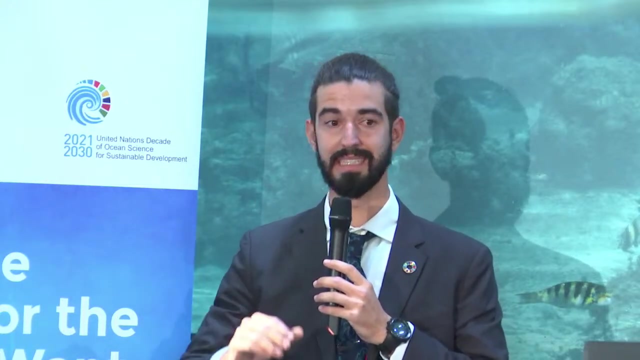 And just one statistic from this paper that will hopefully come out soon. We split the high seas into one-by-one degree cells, so 100 kilometers by 100 kilometers, The percentage of the high seas that have less than 100 records, 100 species records, is 70%. 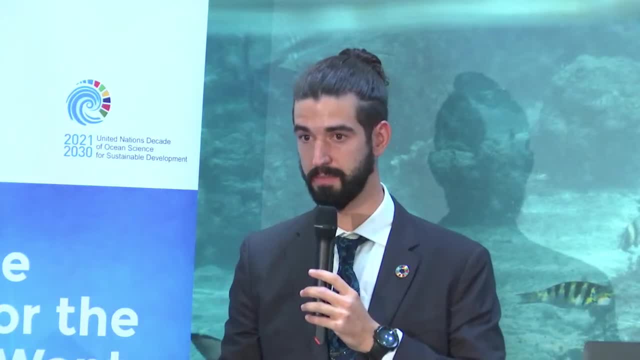 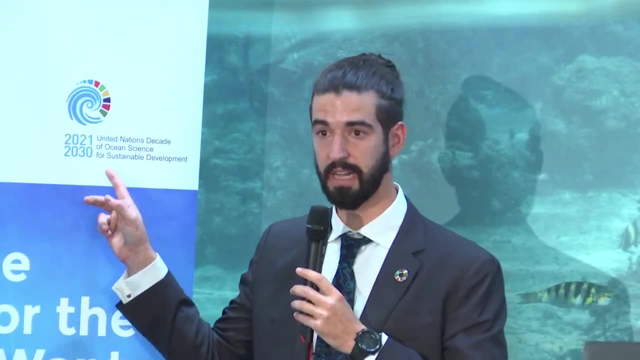 So 70% of the high seas. we don't have more than 100 records in the whole time series of OBIS. So no, we don't have data, but the UN Decade of Ocean Science can hopefully change that. We have to capitalize on those who are out there. 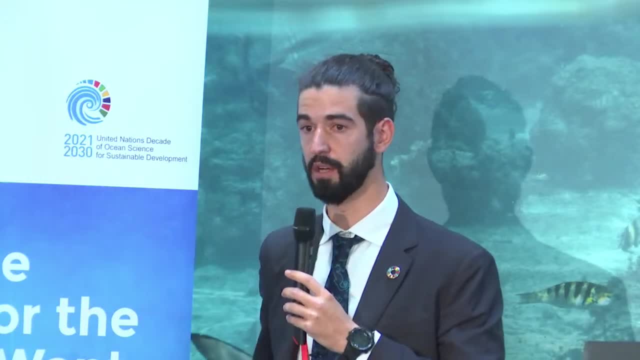 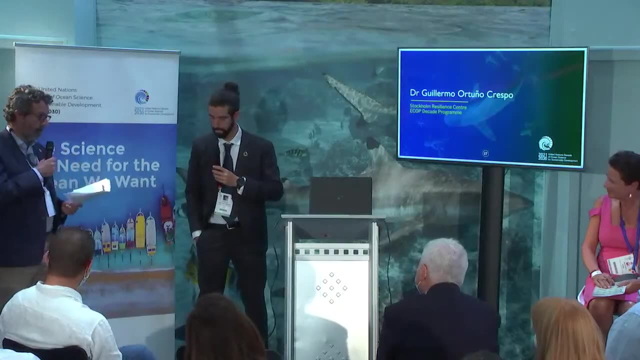 shipping, fishing industry, governments, who are out there and really increase our knowledge if we want a successful BB&J treaty. Thanks very much. Now, of course, that also links up to the issue of capacity development and technology transfer, which is also another core area of a negotiation of a treaty. 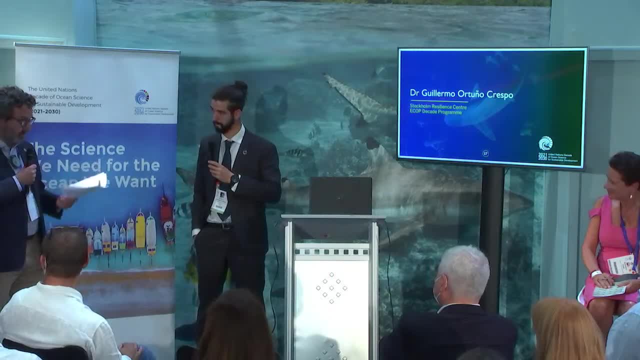 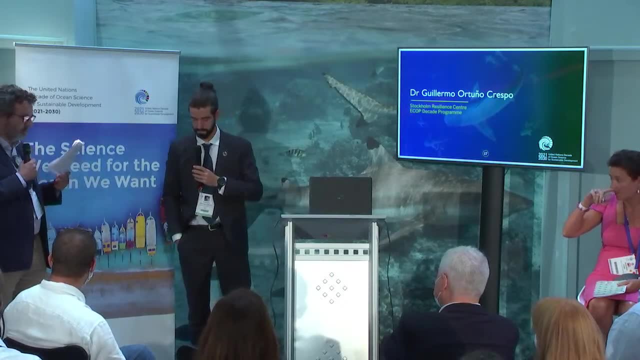 So, from your perspective, I mean, how can we you know we have this negotiation coming up next year? How do we make sure that you know the science is at the heart of the treaty and that you know we have the right advisory mechanism? 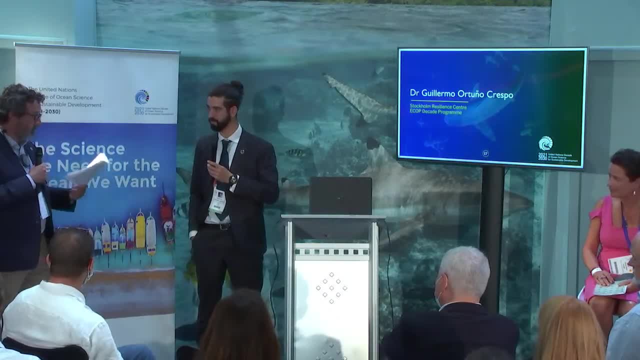 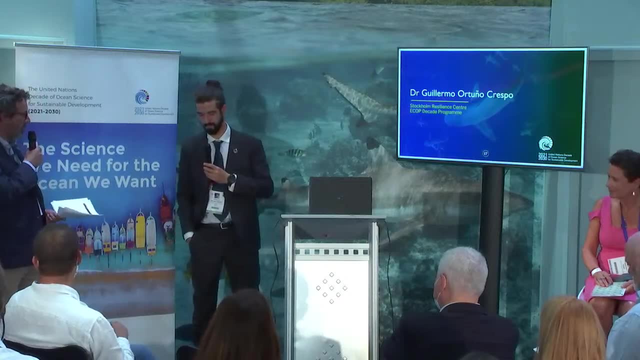 to drive the definition and the implementation of marine protected areas in the high seas. What would be your advice to scientists, for example, who are interacting with their governments? I don't know that my advice would be to scientists at this stage of negotiations. 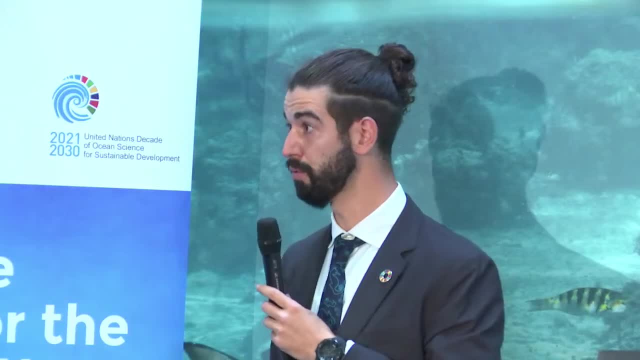 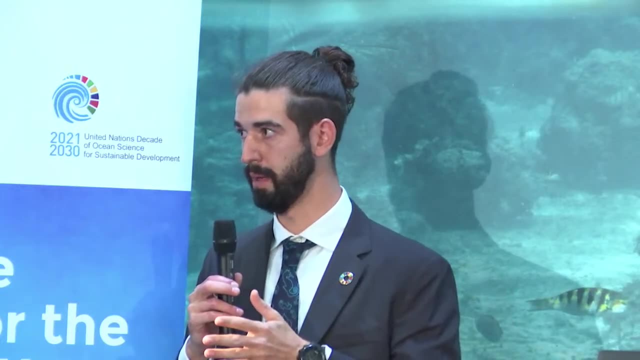 We're not that present in the negotiating room. We're normally set at the back, and we do get to participate every so often. I think the elephant in the room for successful implementation is how this new instrument, which we agreed was not going to undermine existing bodies. 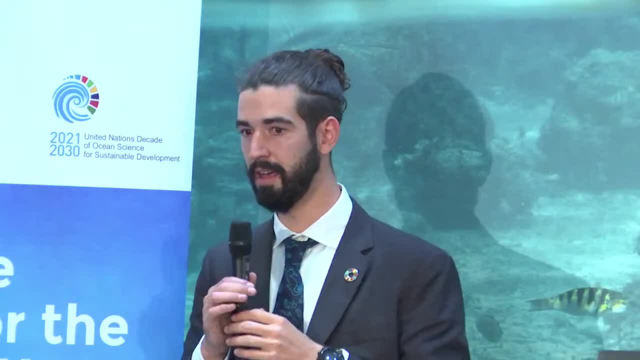 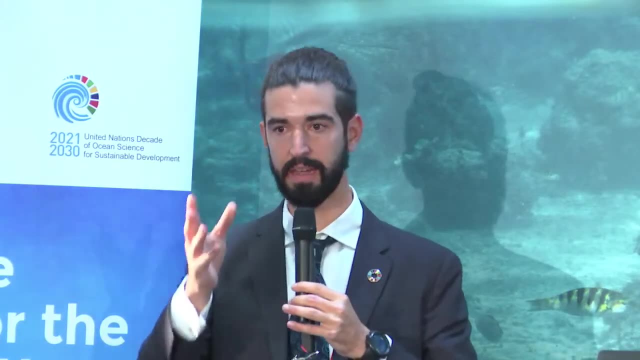 It was not going to undermine RFMOs. It was not going to undermine the International Seabed Authority or the IMO. How are these instruments from a legal perspective? that's when we need to bring the forward-thinking lawyers. how are they going to interact? 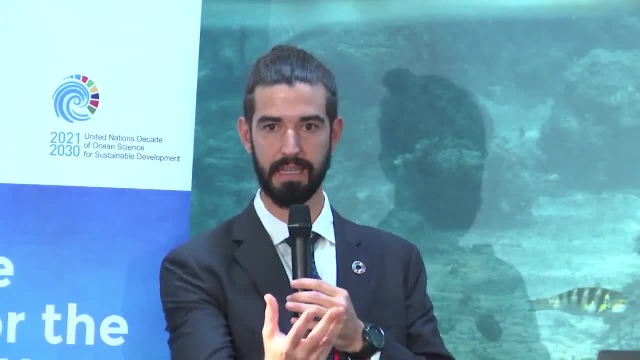 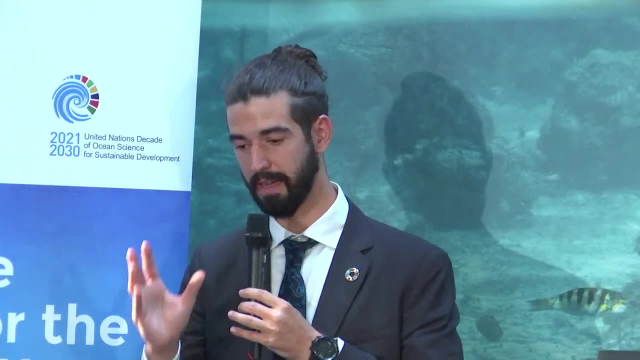 Because if BB&J has a mandate to establish MPAs but the ISA, the IMO and RFMOs do not recognize those MPAs, we have nothing. So I think that's where being more transparent about the legal mandates of each body. 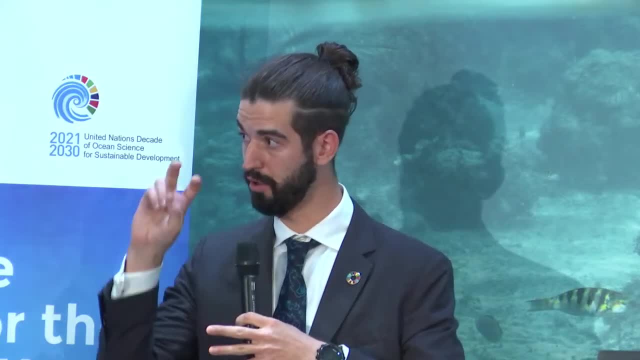 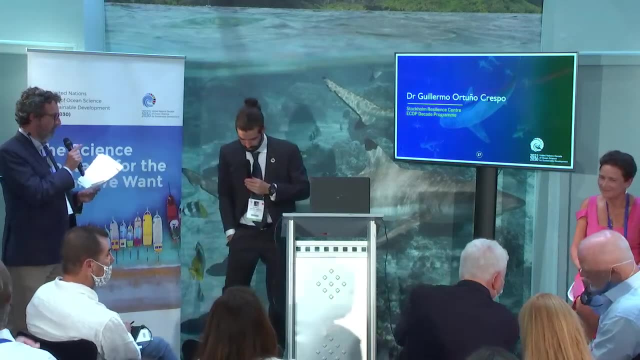 so that they can interlock and work together as opposed to undermine each other is where we need to be placing our focus, I think, at this negotiation stage. Just one last word very quickly. Can you say a little bit more about the engagement of early carrier ocean professionals in this process? 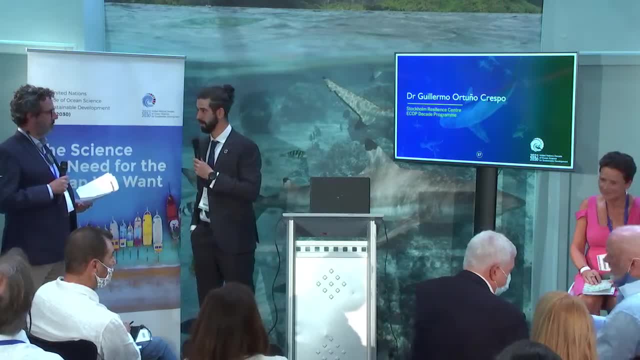 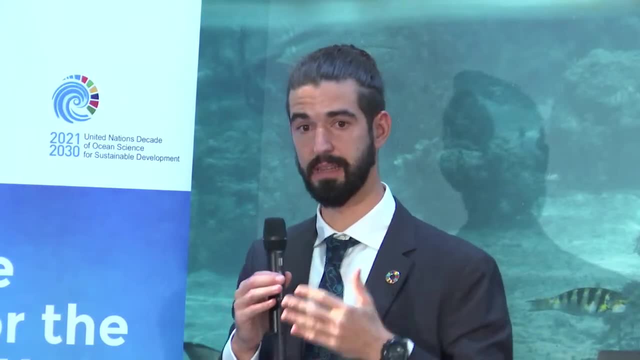 It's been limited, I would say. I think over the last five years I've been able to participate in some of these conferences. I've been one of the lucky ones purely, I had a major chance that the lab where I did my PhD 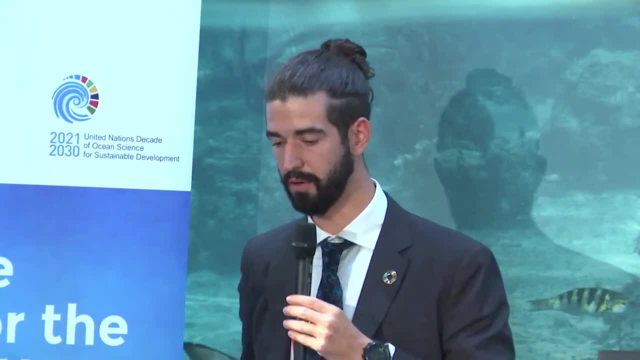 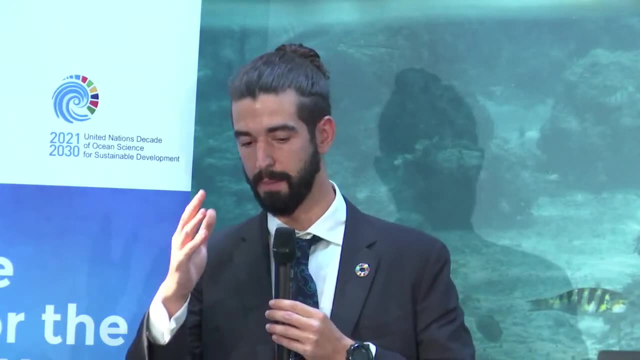 had connections with the CBD, with the ISA and other UN processes. We need to start training the next generation of ocean professionals so that they can both generate science and policy briefs. They need to be able to translate in both directions. 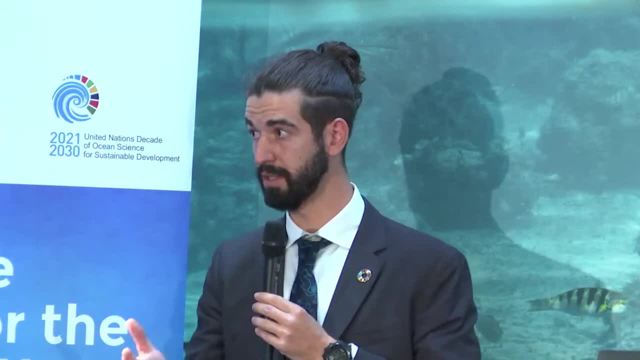 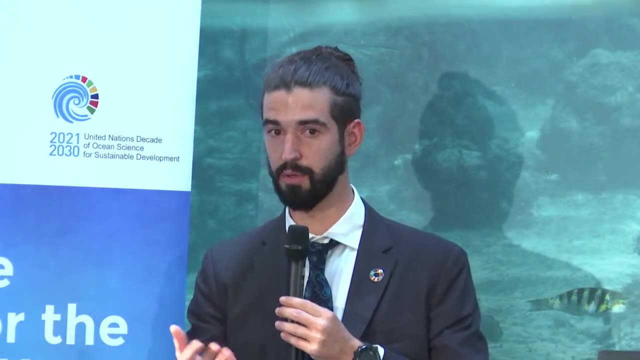 and that takes time. I've been attending these negotiations for five years more or less, and I'm still learning about when to speak, when to share knowledge with whom, so that it can be used strategically to advance a text negotiation. So maybe I've seen 10, 15 early carrier professionals in total. 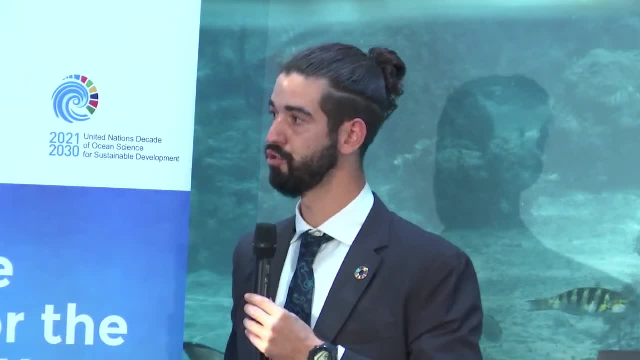 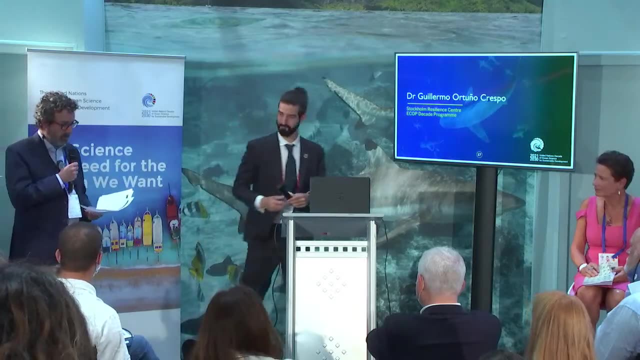 So we need national delegations that should try to bring in the next generation of ocean leaders into these negotiations to learn Very good, Thank you very much. Clearly, BB&J is about defining the ocean governance, probably for the next 40 to 50 years. 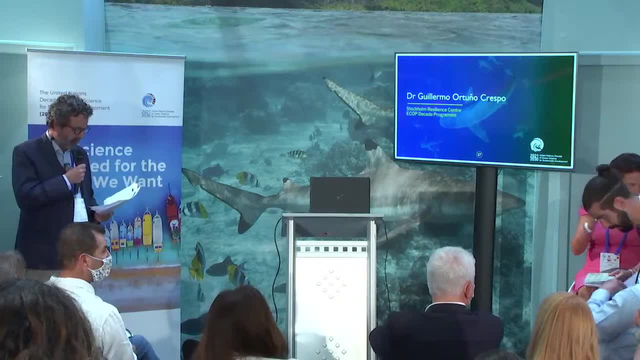 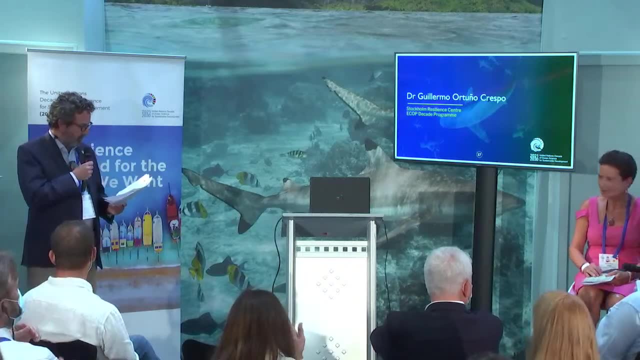 so I think it's important that all generations get involved in that process. Okay, now let's go to Thank you very much, Guillermo. So our last segment is really about really trying to sum it up and, in particular, why we need co-design. 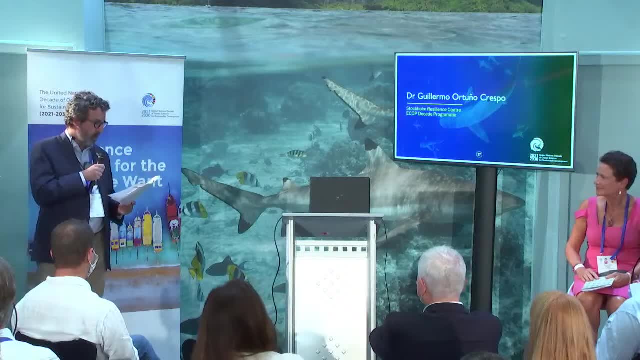 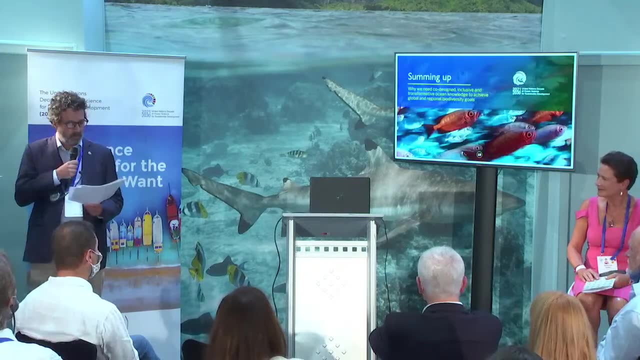 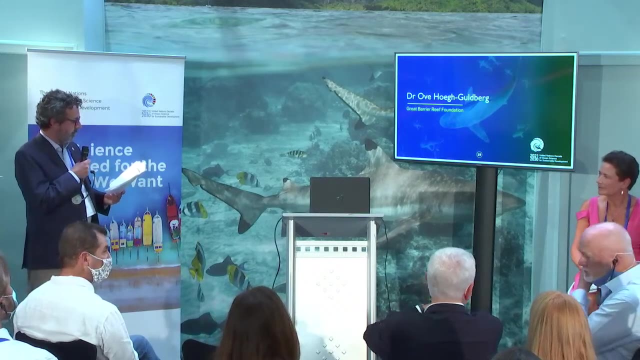 inclusive and transformative ocean knowledge solutions to achieve our biodiversity goals. Before we go to my next speaker, we have one more little video, and this is from the Great Barrier Reef Foundation, the chief scientist, Professor Uwe Goldeberg, who is an internationally acclaimed marine scientist. 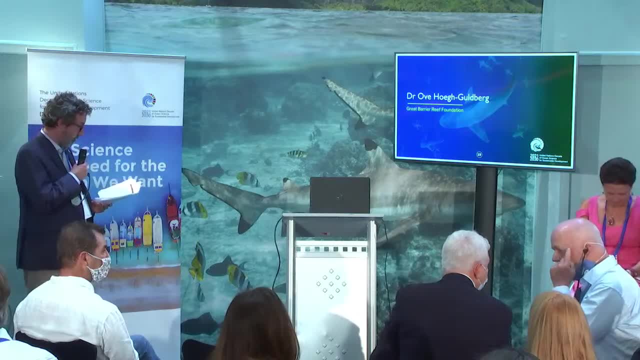 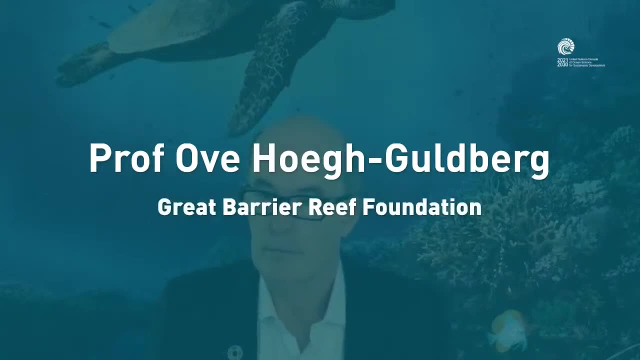 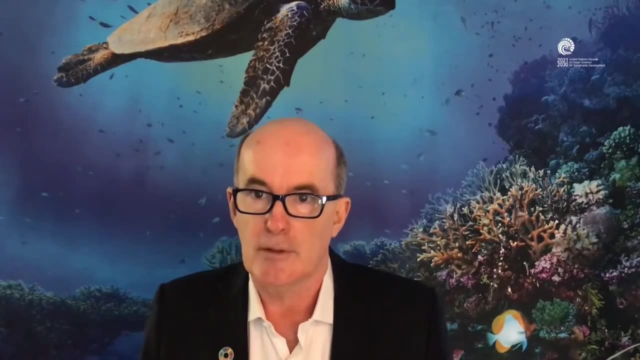 and leading author on coral reef science and conservation. Let's go over to Uwe and then we go to our speaker. The ocean is one of the great reservoirs of biodiversity on our planet, providing habitat for hundreds of thousands of species, many of which are still undescribed by science. 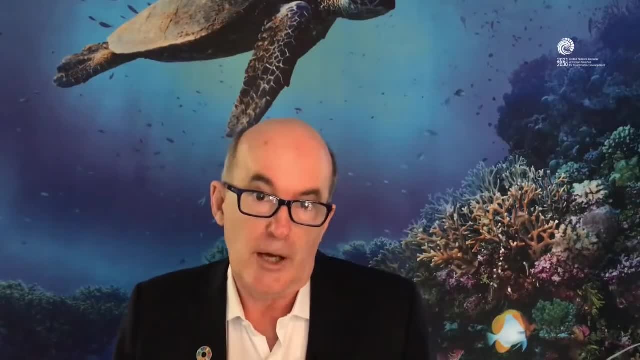 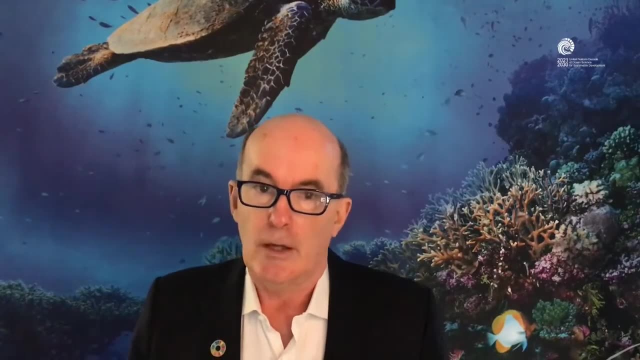 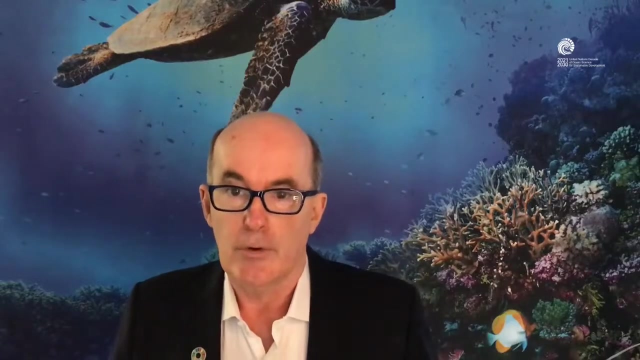 Despite the importance of these species, however, ocean biodiversity is declining at an alarming rate and will have catastrophic consequences if we don't turn it around. If we don't do anything, we will face an increasingly dangerous and unstable world, And this is why the UN Decade for Ocean Science. 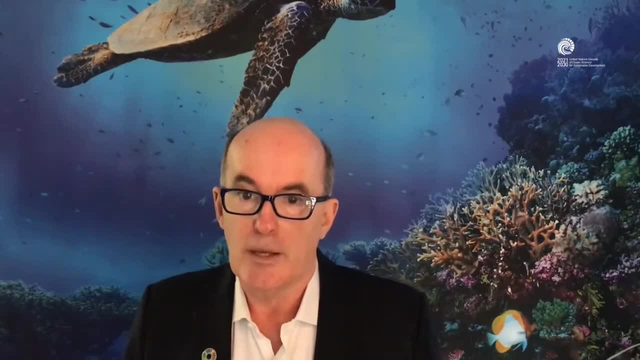 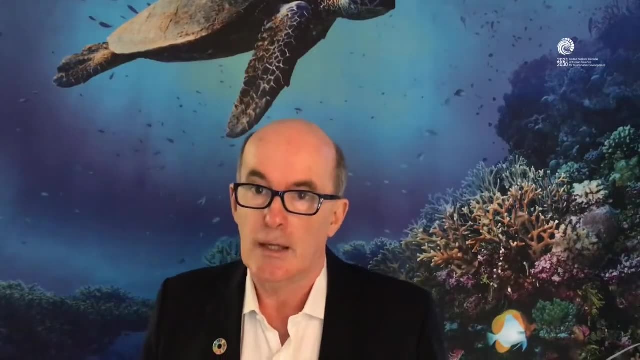 is so important and why we must seek science-based answers to turn this situation around. We need to know how we can use the ocean decade to galvanise a global effort to reverse the tide of habitat degradation and biodiversity loss. We also need to develop innovative solutions. 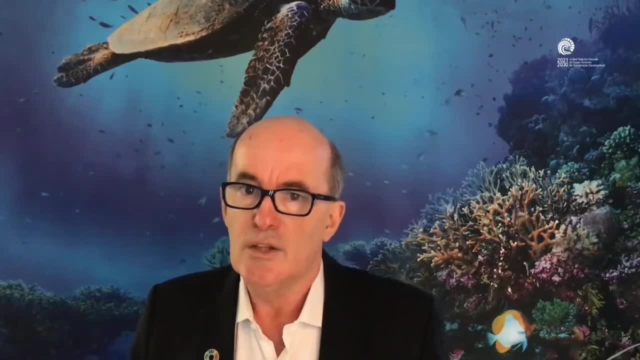 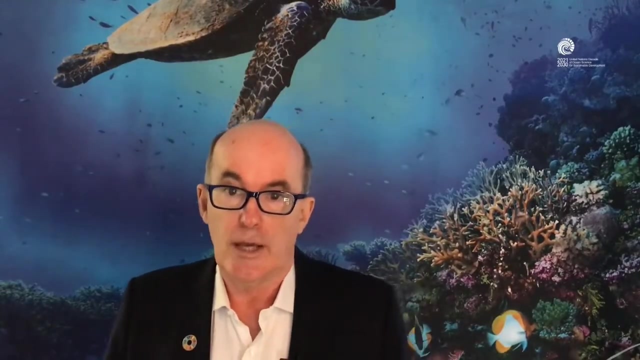 that are co-designed with those who need the knowledge to make the critical decisions at the local, regional and global scales. And this effort will need to be turbocharged in terms of innovation, such as we're doing at the Great Barrier Reef Foundation through the world's largest coral reef grants program. 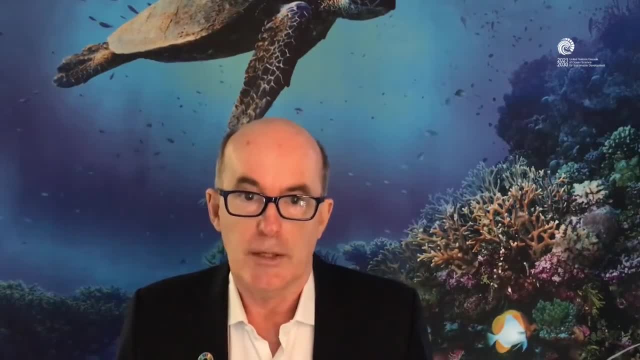 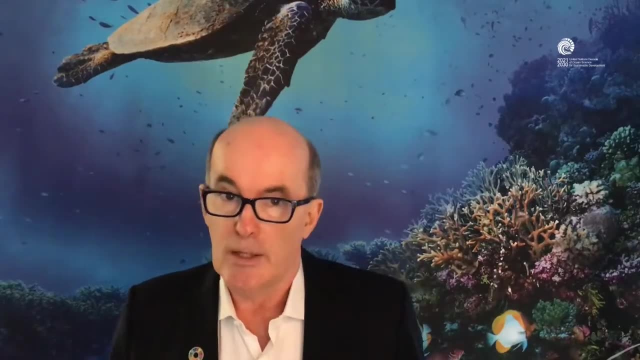 And, most of all, we must be bold. Time is running out And, finally, we need to know where we're going and what success will look like at the end of the ocean decade in 2030.. Hopefully, we'll have a reinvigorated ocean. 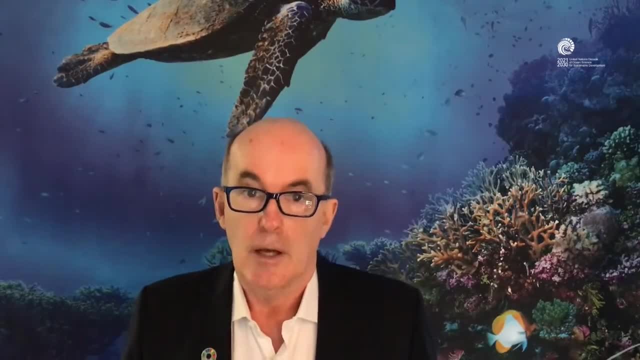 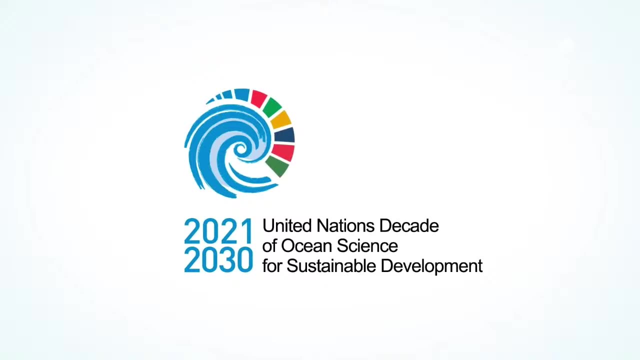 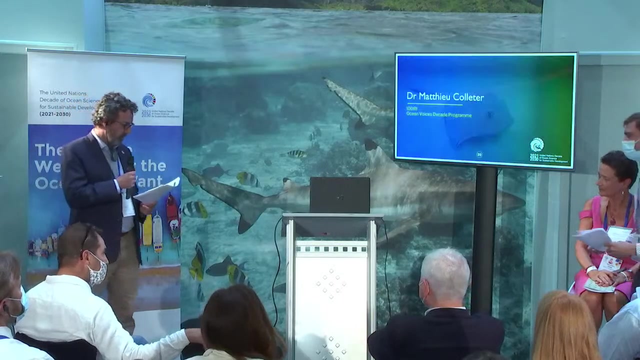 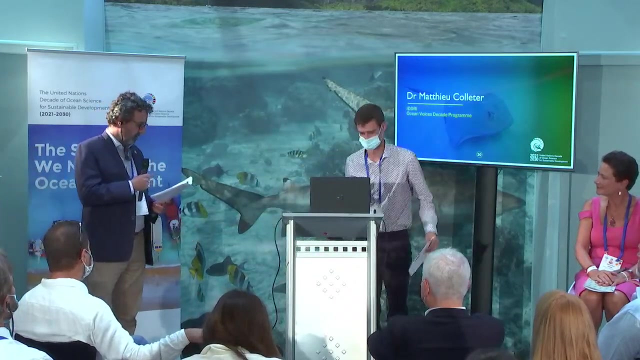 that's bursting with life and opportunity. again, I hope, and I believe so. Thank you. Now let's go to our next speaker, Dr Mathieu Colleté, who is an agronomic engineer specialising in fishery science. Mathieu works as a 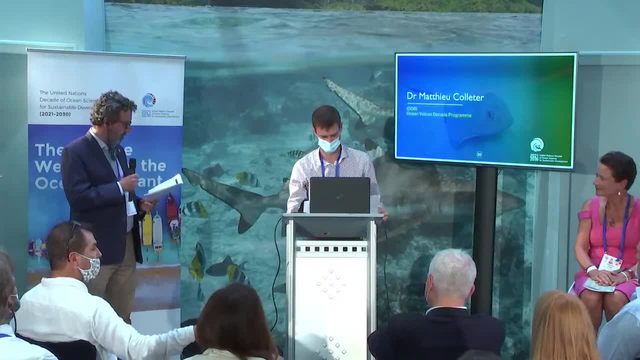 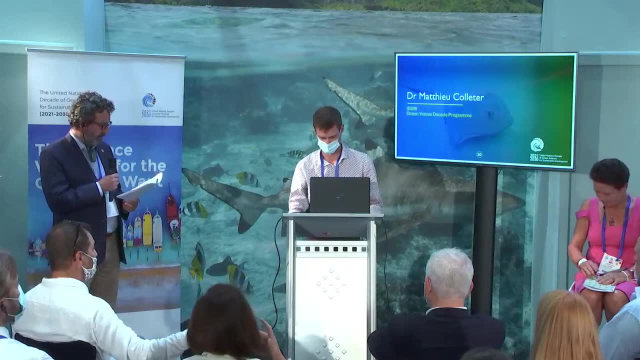 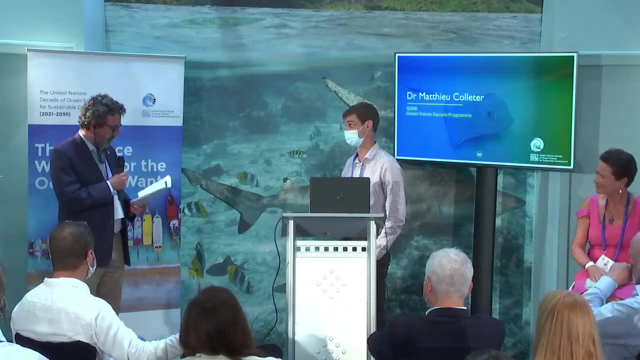 focuses on small-scale fisheries industry and particularly how they integrate within larger European fisheries policies. He's involved in the Ocean Nexus International Research Programme, which is hosted by the Institut National Polytechnique and the Institut du Développement Durable pour les Relations Internationales, LIDRI. 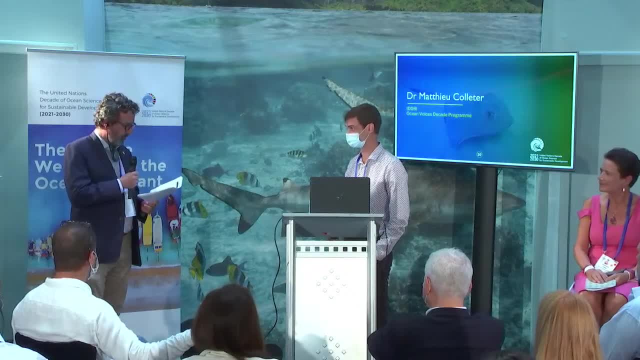 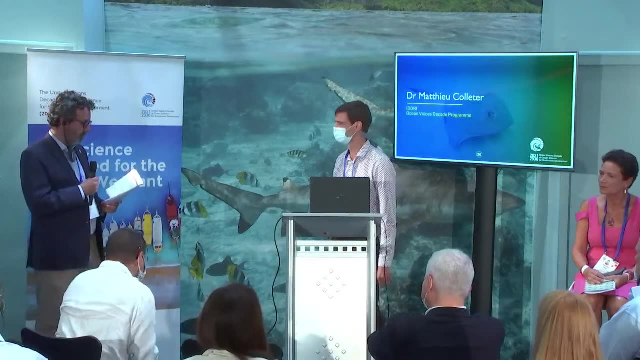 And he's also a member of the Ocean Voices Ocean Decade Programme. So, Mathieu, why is ocean science such an important part of the solution to achieve global and regional biodiversity goals? Can you give us some examples of critical gaps in ocean science and knowledge? 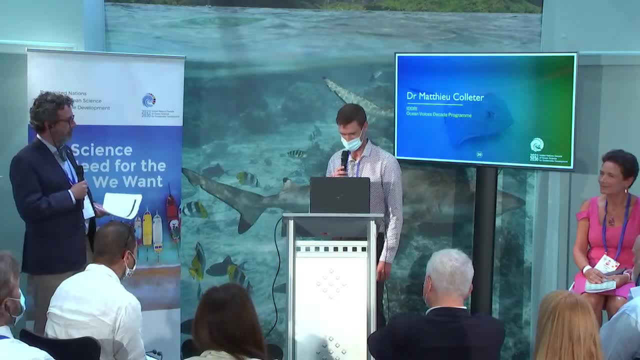 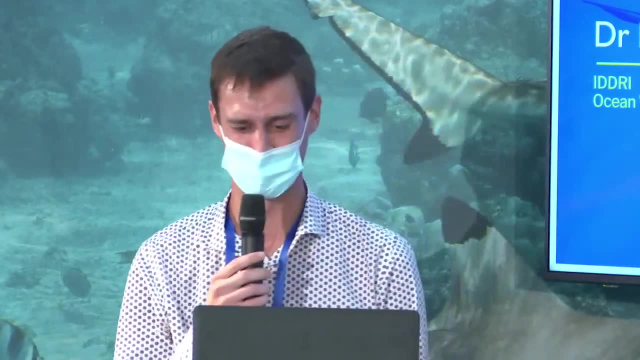 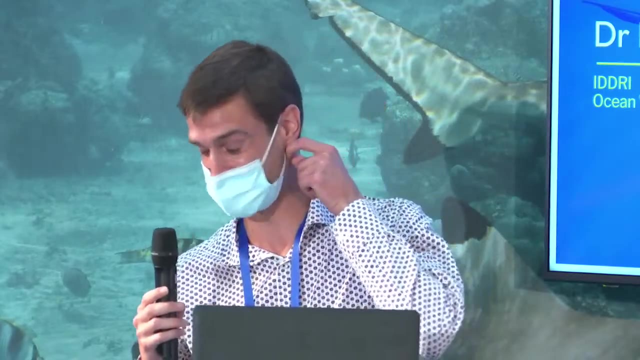 that are impairing our ability to achieve those goals Absolutely. First of all, thank you very much for the invitation and for the opportunity to speak today about ocean science and the Ocean Voices Decade Programme that is supported by the Ocean Nexus Centre. I'm part of 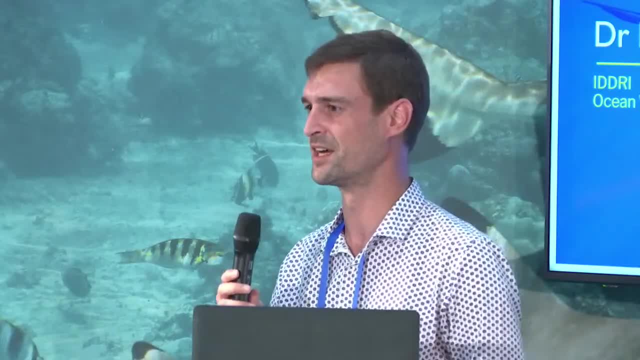 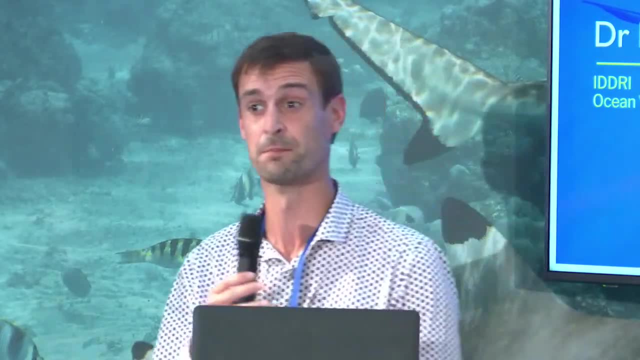 First, I think it's important to note that ocean science includes a great variety of disciplines- I mean absolutely. we are talking about oceanography, biology, ecology- that provide very important data to monitor, etc. But we also talk about social sciences and humanities. 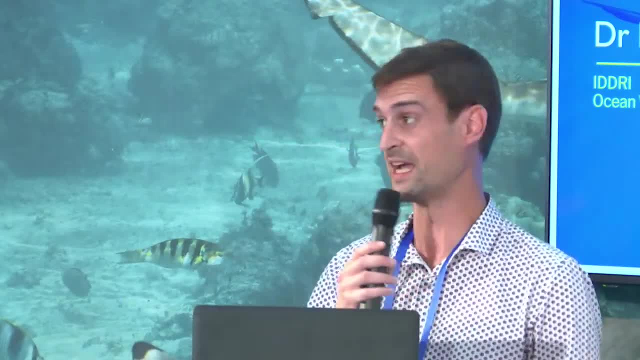 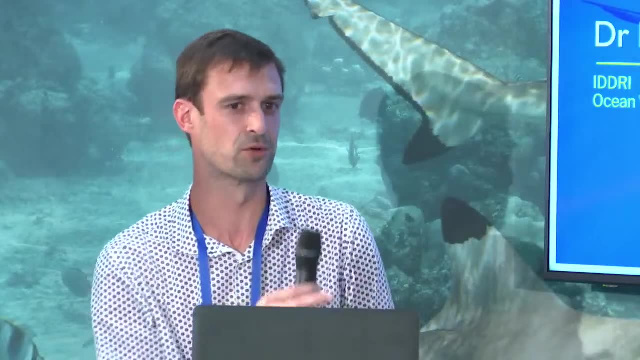 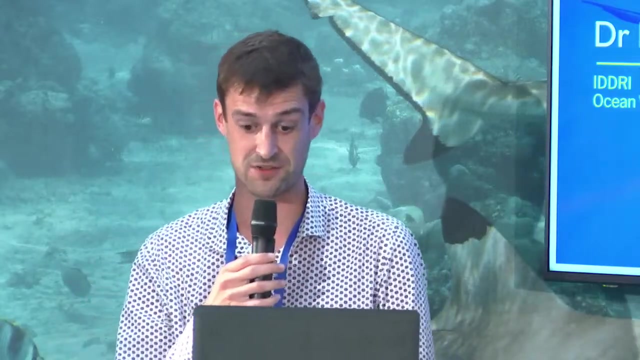 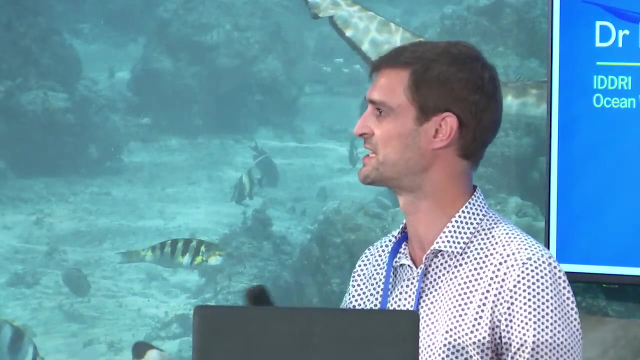 that are key to tackle equity issues and to design more inclusive approaches of designing and conducting marine science, And so we all know that the ocean represents 90% of the volume that life can support, And so biodiversity there plays a vital role in maintaining the productivity. 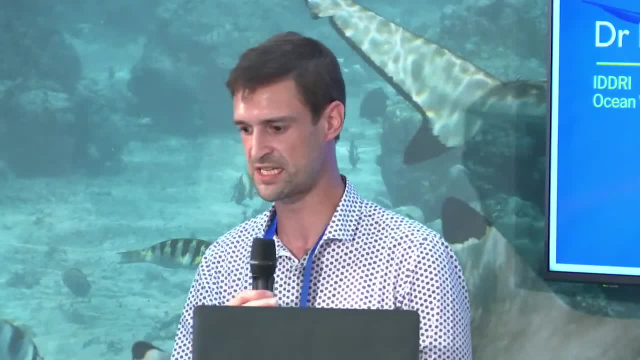 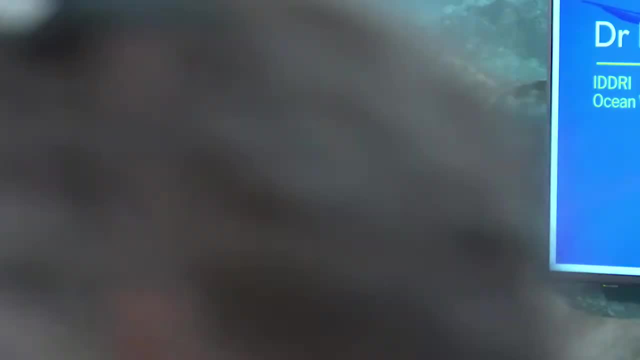 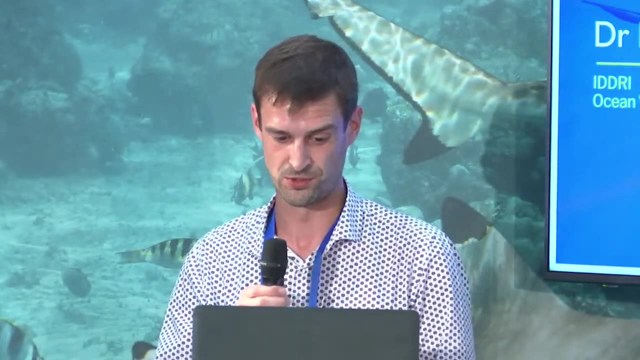 the resilience of ecosystems And so marine biodiversity, with the multiple stressors we know, be it climate change, pollution, transportation, overfishing, and so ocean science in all its diversity is key really to monitor, but also to develop these solution-based approaches. 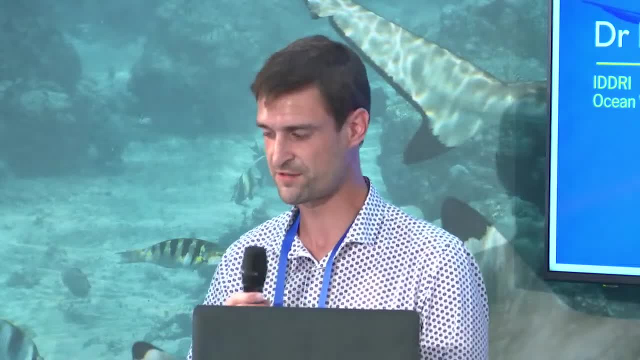 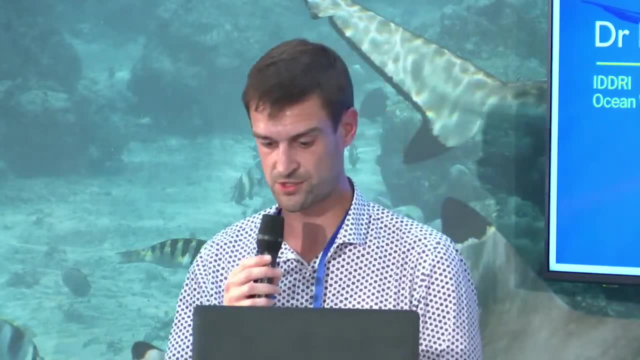 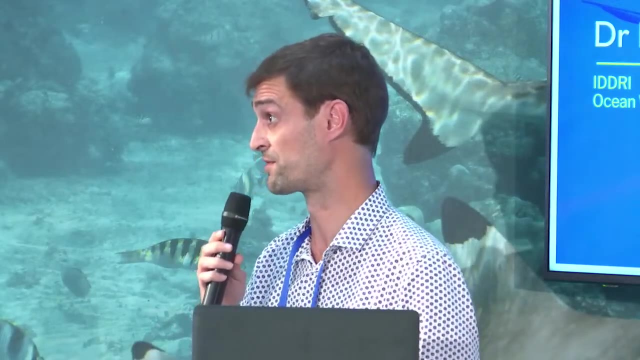 we are asking for, And so there are different important gaps, but I think one gap that we really identify within the Ocean Voices Program is the need to better understand the needs and the priorities of ocean-dependent people and evaluate potential solutions for them. Gerald Singh, Harriet Arden Davis. 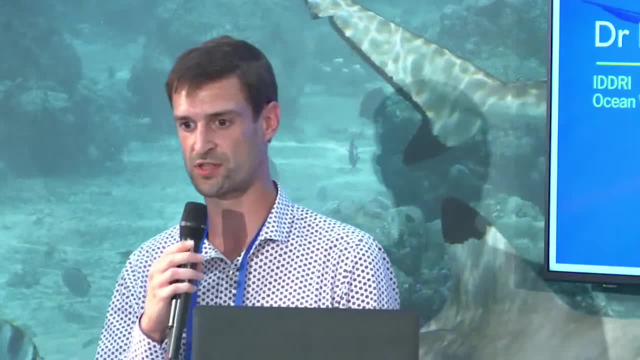 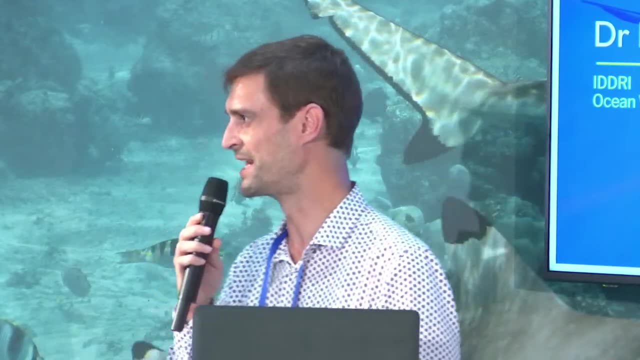 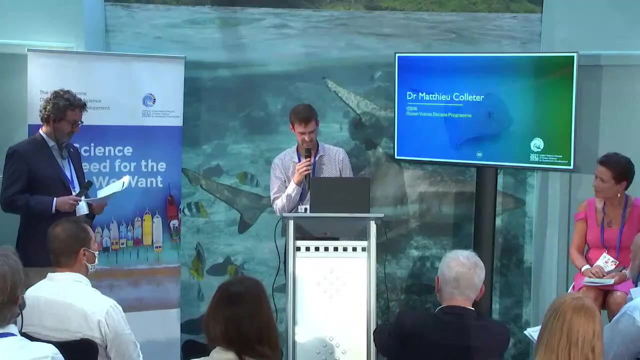 and other colleagues from the Ocean Nexus Program wrote at the beginning of the year an opinion paper entitled Will Understanding the Ocean Lead to the Ocean We Want- And it's a bit to echo the phrase of the decade- And they really outlined that science does not inherently lead to. 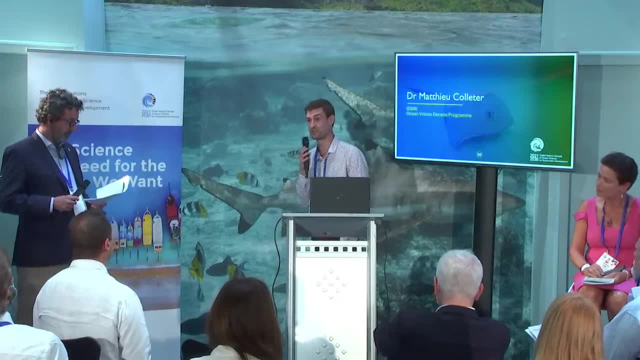 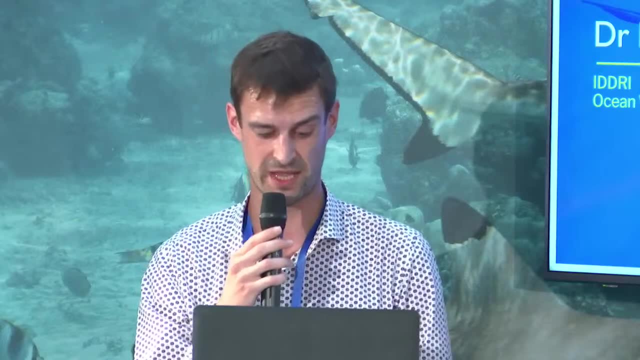 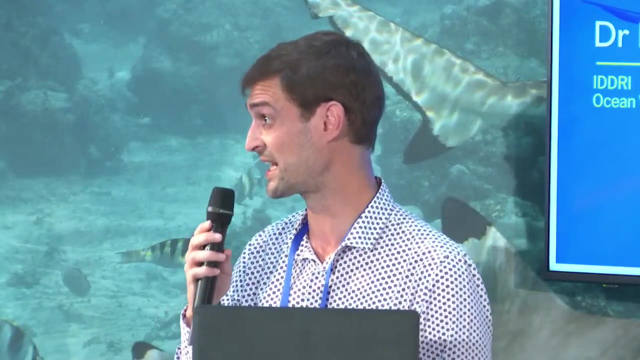 sustainable or unsustainable, or equitable or unequitable outcomes. It really depends on how, where, when and by whom the science is going to be either funded, conducted and used, And so there is a need to really consider explicitly the leaving no one behind commitment. 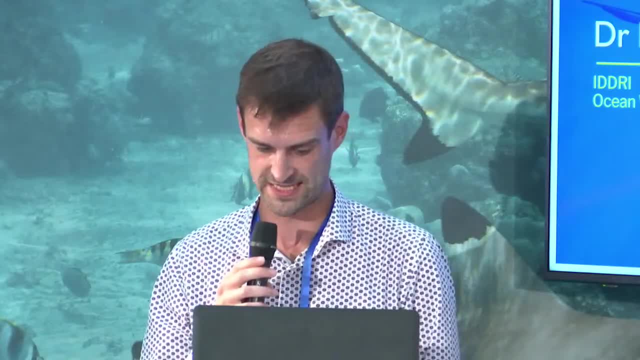 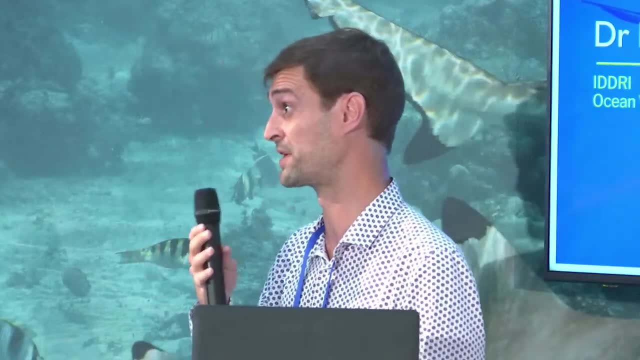 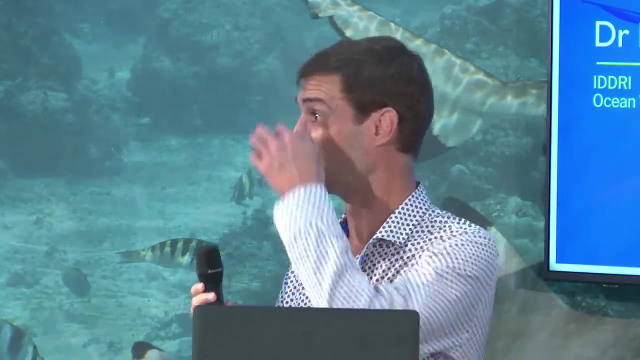 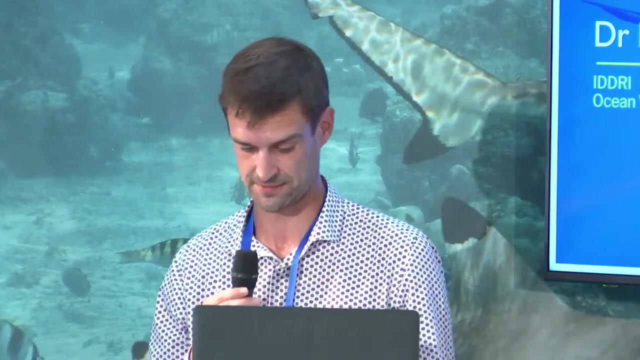 of those sustainable development goals, And that's really because otherwise you may have scientific solutions that may lead to unsustainable or unequitable outcomes, And so, in our opinion, solution-oriented research is really a key and a critical gap to fill to achieve collective goals that are being set. 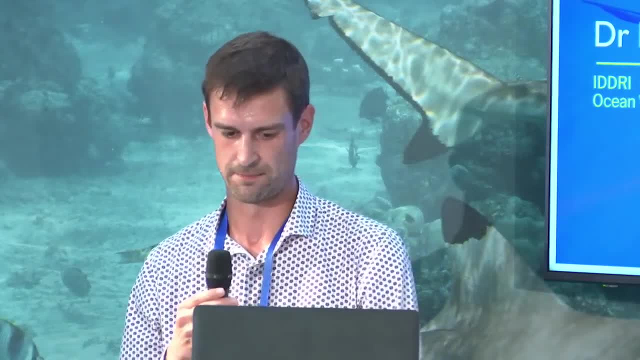 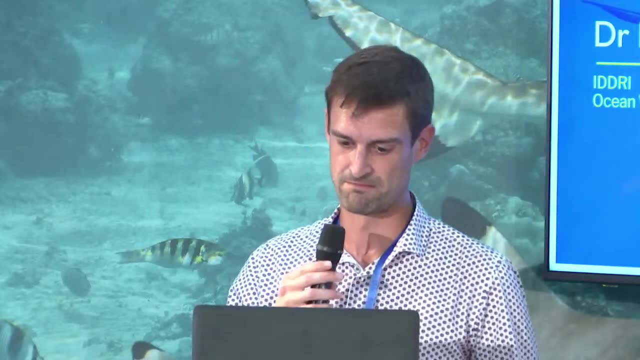 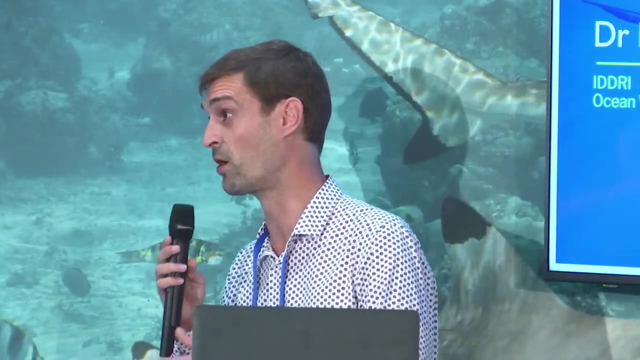 I think a second element is that we need to develop approaches that are really responsive to diversity, that are inclusive and being conscious not to decouple this from the political economy. So we should really aim for a renewed dialogue between all communities- ocean communities. 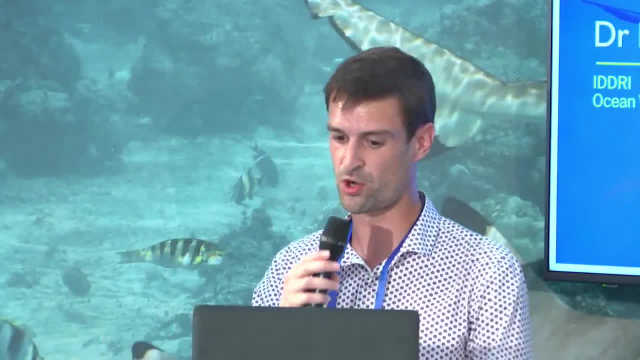 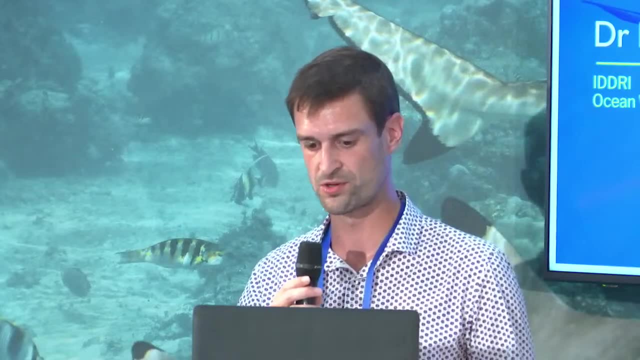 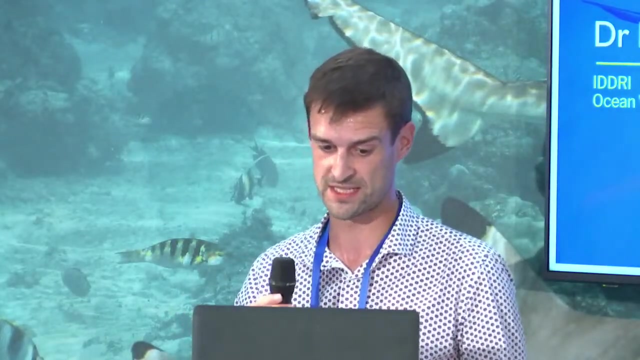 ocean stakeholders and to work across the ocean science policy interface. And an example, an iconic example, a very important one, is, for example, gender equality and equity, Because it's part of the principle of good governance, It's recognized And, within fisheries, 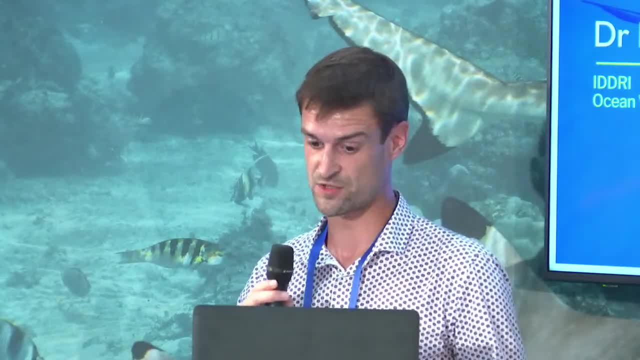 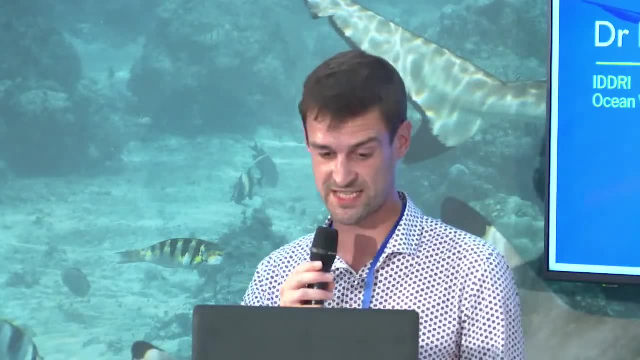 it's critical for effective governance, And so, for example, within the Ocean Nexus program, we got a project called Gendered Inequities in Ocean Restoration. It investigates structural power asymmetries in the rapid station of constant nature, And so this is, for example, 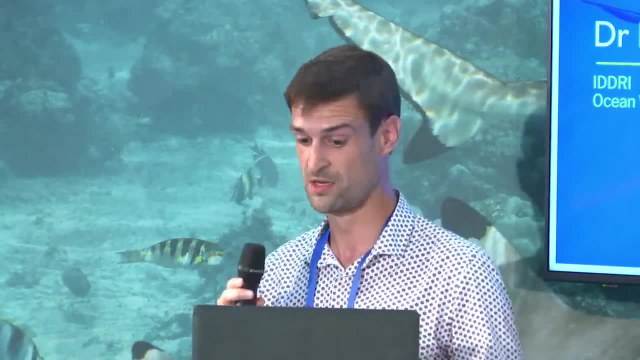 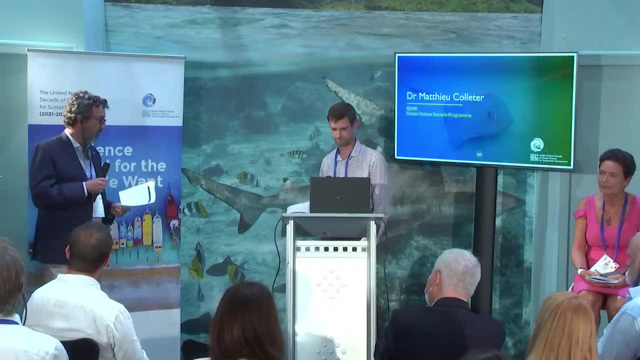 crucial research that needs to be done to achieve these collective goals. Great, Thank you very much. So it's all about co-design and co-delivery. Can you maybe identify some factors of success that can really help us to do that, Because we talk a lot about it. 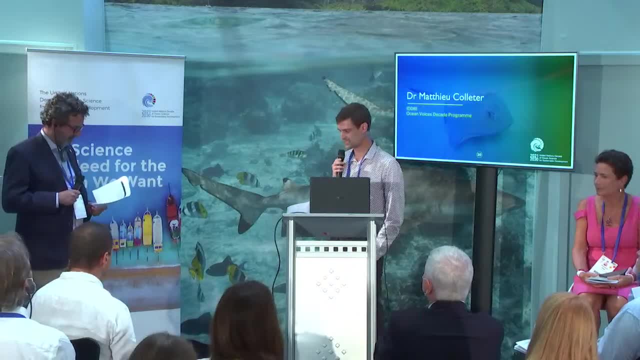 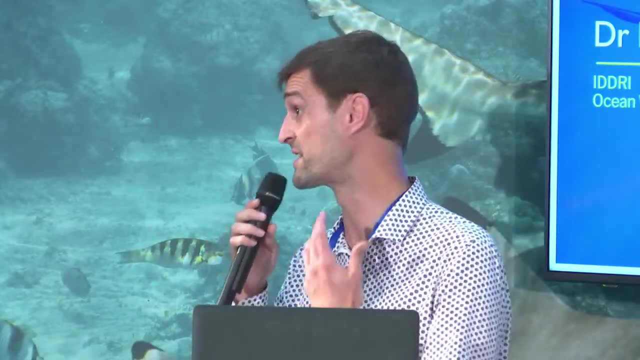 but concretely, what does it mean? Yeah, no, absolutely, And it's the whole process, not only for everybody, but also a lot for the scientific community to think about, the research we do and how we do it And, I think, to be successful. 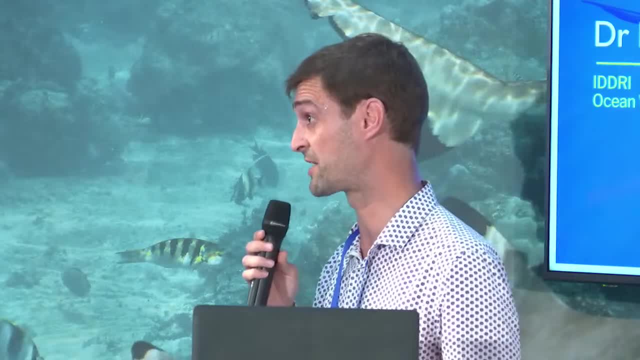 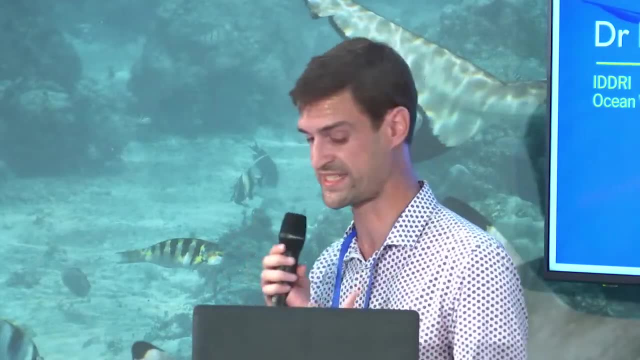 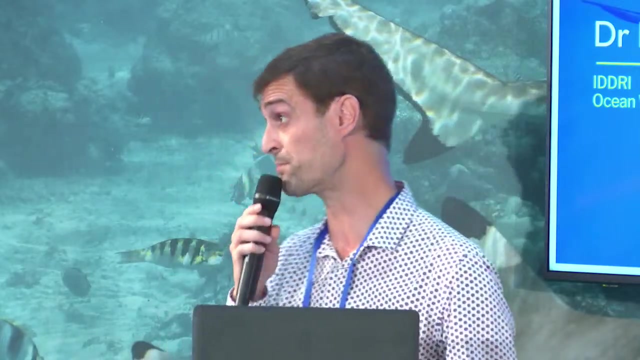 co-design. ocean science needs a refined understanding of the actors involved, of their culture, of their well-being, and how power dynamics and decision-making processes influence our oceans, So developing strategies, governance frameworks and enabling conditions to improve equity and inclusiveness in the design. 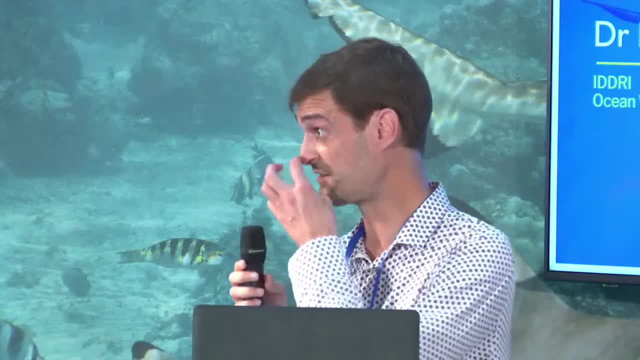 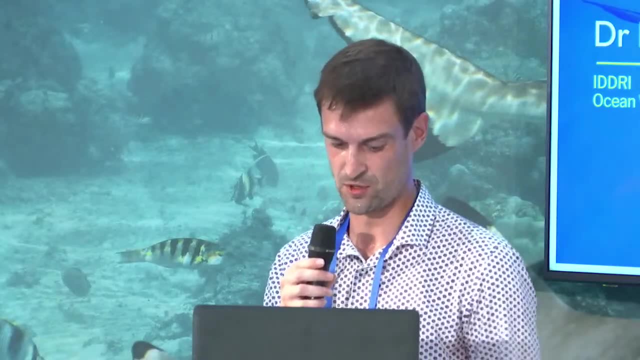 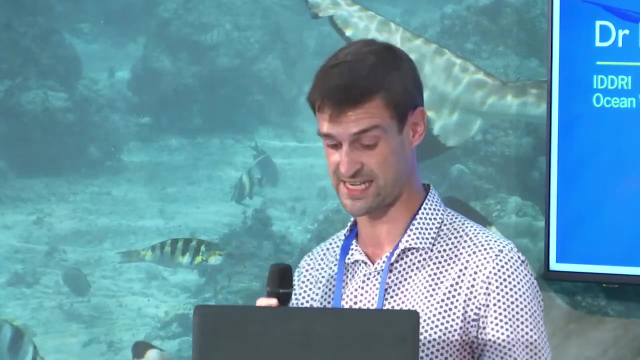 conduct of science will be key to leave no one behind, as committed in the SDGs, And so the Ocean Voices Program, led by Harriet Arden Davis, will conduct research, incubate ideas, facilitate discussions, convey capacity-building partnerships to advance equity within the decade. 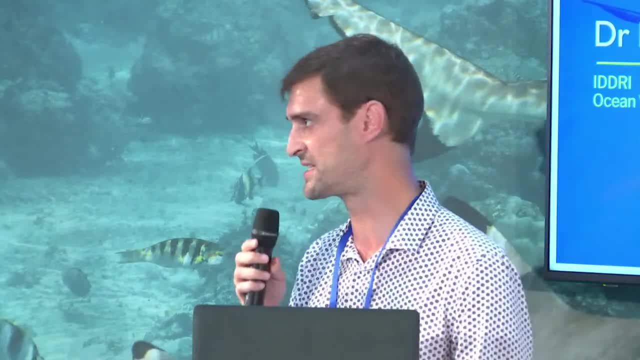 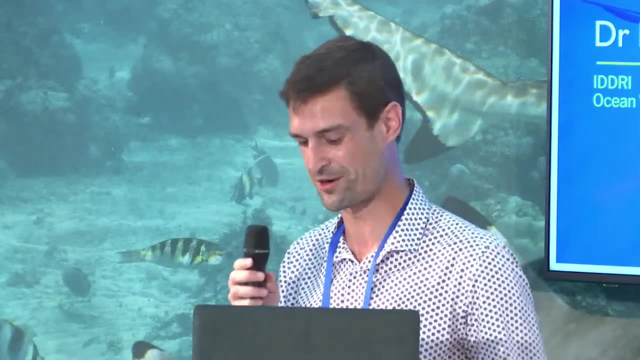 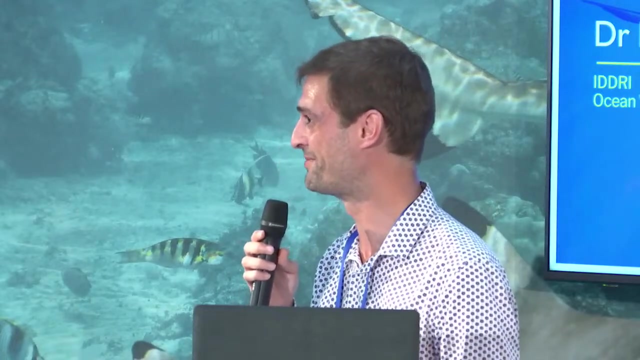 And we really aim to do this and stimulate discussions across disciplinary, sectoral and geographical boundaries, And so that's our aim- and to really also focus on this solution-oriented research. If we achieve this objective, that would be quite successful. So, yeah, let's go back to work. 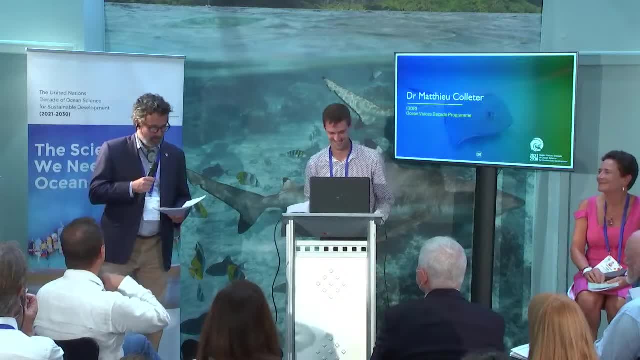 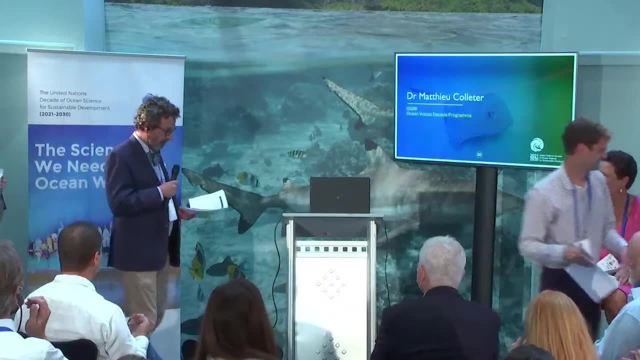 All right, That's the way of doing business. Thank you very much, Mathieu, And please stay with us. We're now going to go into the Q&A session, So we have a Slido where you know our webcast audience. 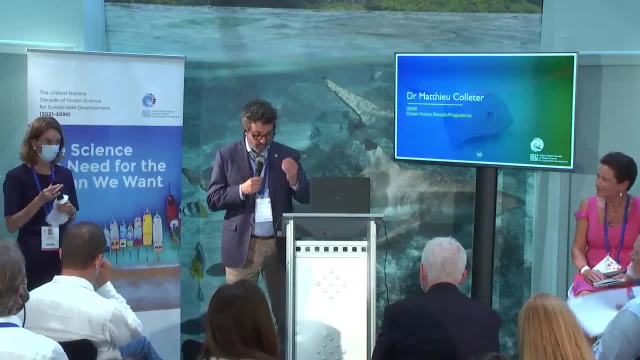 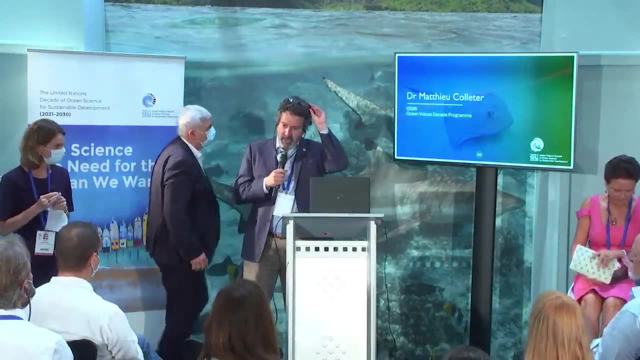 can certainly post questions, but we can also take live questions from the audience. Maybe before I see there's some Slido questions coming up here And also this: yes, Vladimir, you are one of a person that can also answer the questions. 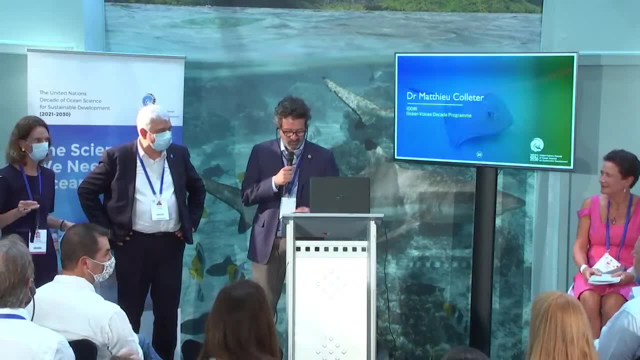 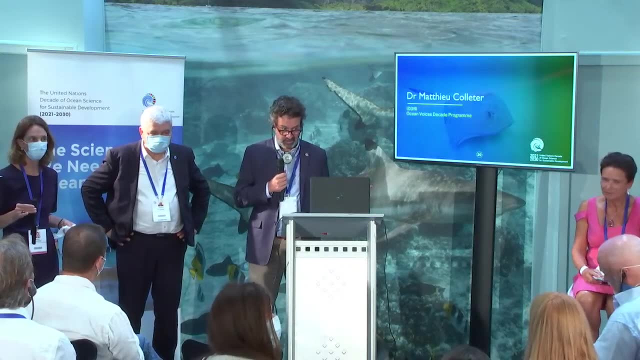 So if you have questions about the decade, don't hesitate. We have our executive secretary here with us. Let me just ask if there are any questions in the audience, live before we go to the. Yes, I see the gentleman here. You'll need to speak into the micro. 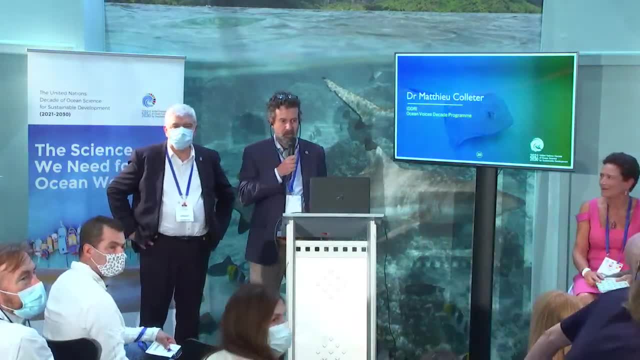 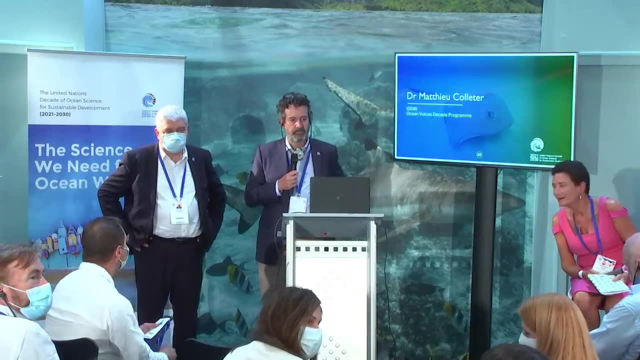 even if you can't really hear yourself. it's for the streaming. If you could please introduce yourself and then ask your question. Yeah, my name is Ralf Sonntag. I'm with the World Future Council in Germany And first of all, 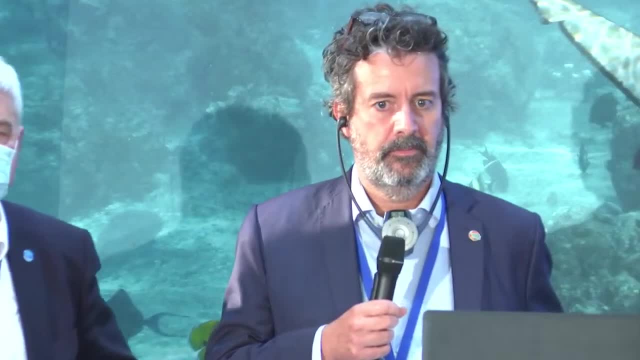 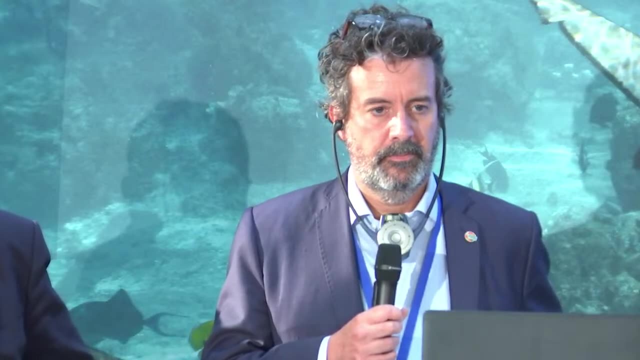 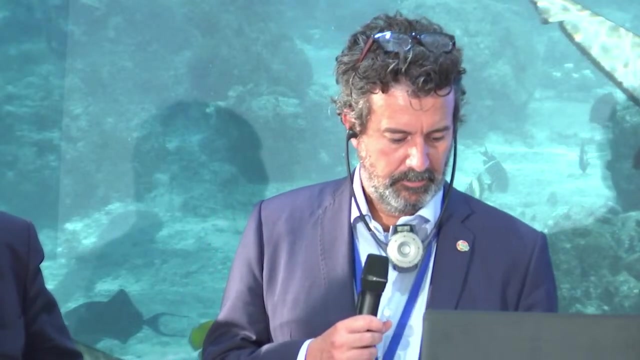 I would like to thank you, the presenters. It was some very nice and very interesting presentations And I mean my impression is that of course we need much more science. We need a lot more science to understand the oceans. We only have very little of this. 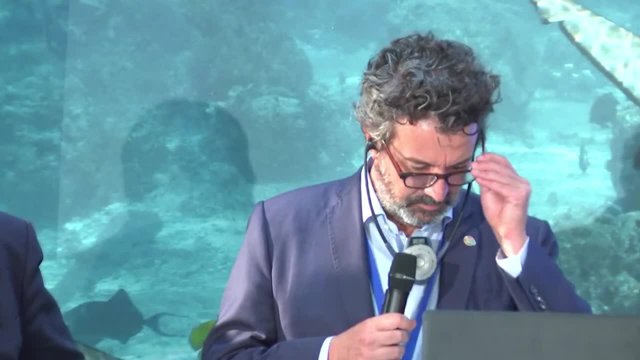 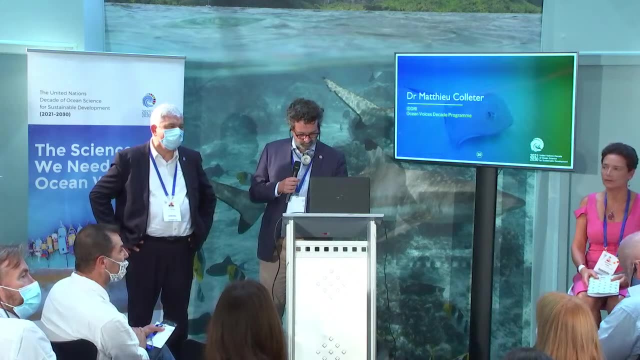 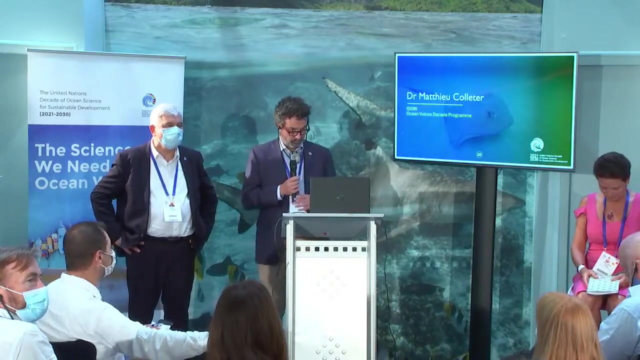 But I think we do have enough science to know that the oceans have a problem right now and that the problem is growing and that we need to act. So I really think the very important thing is that we have now political action, that politicians around the world 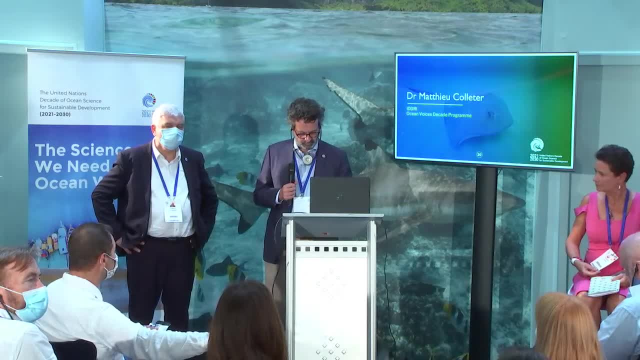 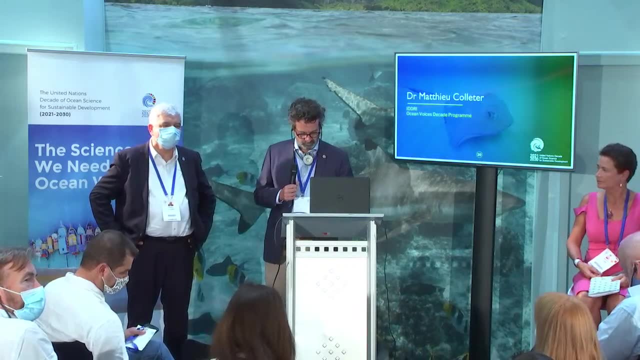 agree to the BBNJ Treaty and politicians around the world agree to the 30 by 30. I think those are the key issues which we should start right now. Thank you, Okay, So more, I guess, a commentary from our audience. 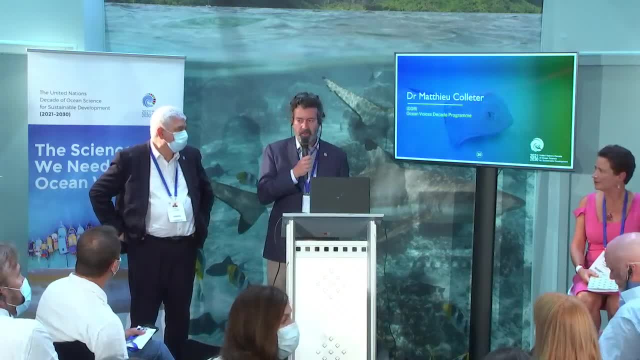 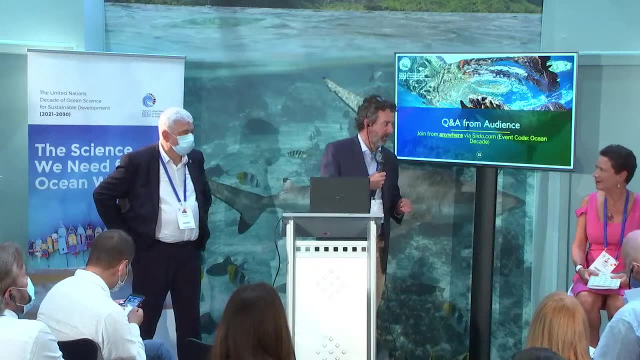 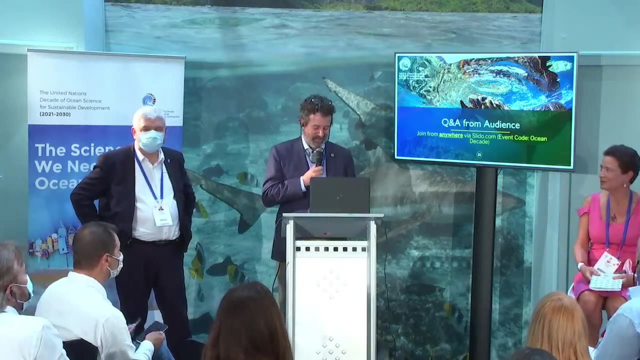 Anybody else would like to pose a question? You didn't hear the question. This was not a question, It was more like a comment. Okay, So you're off the hook for the time being. Anybody else? Okay, I have a couple of questions from Slido. 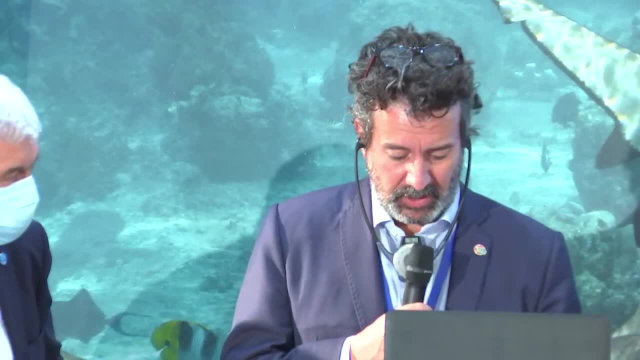 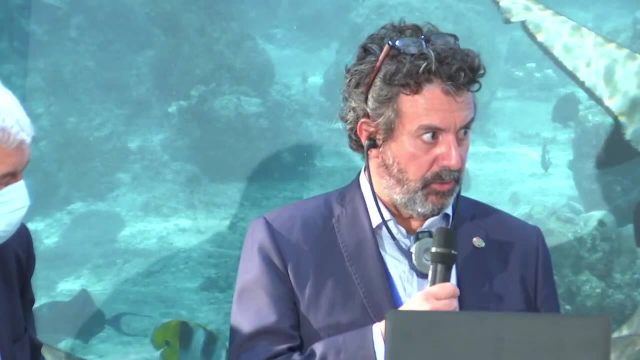 Well, first, Geneviève, you will have a question because somebody is asking about how can we find out more about Ocean Unite, So maybe you can take a minute to mention that. A question related to data, I don't know. 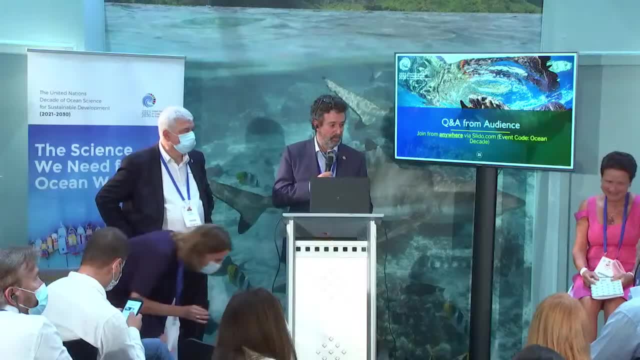 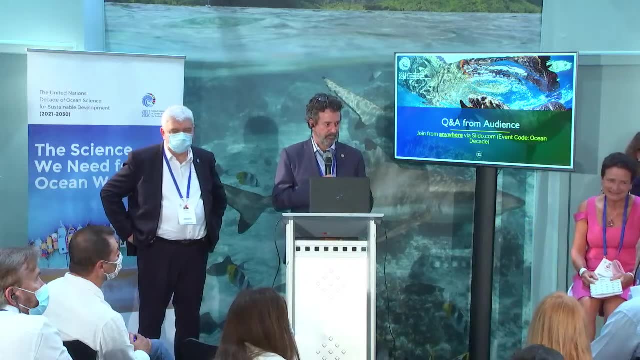 Oh, we have a live question. Let's take the live questions. If we can, please pass on the mic. Thank you very much, Francois Galgani from IFREMER. I'm part of the mission board for the mission Starfish. 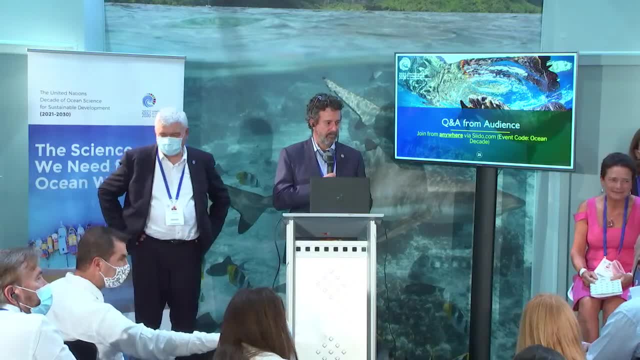 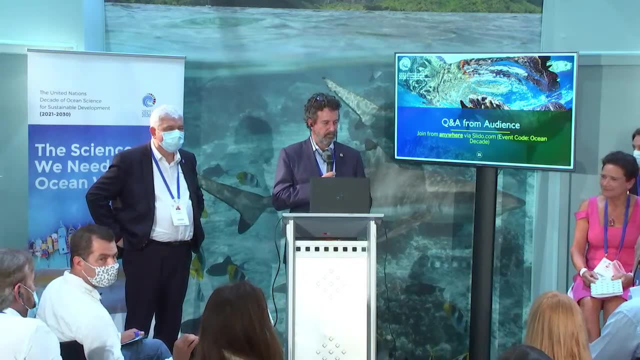 And the question is about how you will harmonize the program of Ocean Unite in different countries. You did have regional initiatives already to set up a recommendation and set up the program then. But I mean, would there not be any difference in the way to solve the problem? 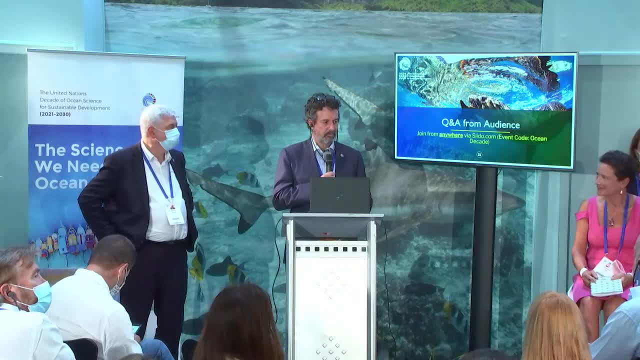 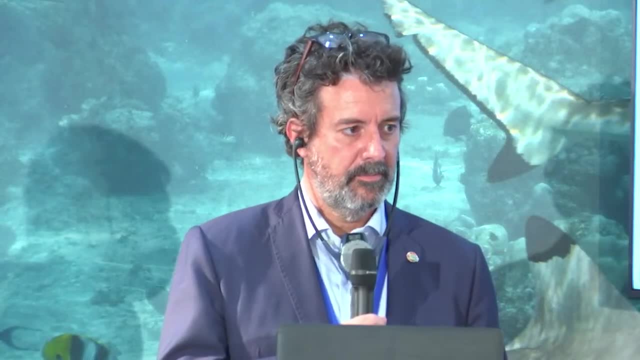 and involve scientists in the decadence zone, And what could be the role of, how we say, regional initiatives such as the mission Starfish from the European Commission, for instance? I think it could help And we may, I mean, harmonize both, probably somewhere. 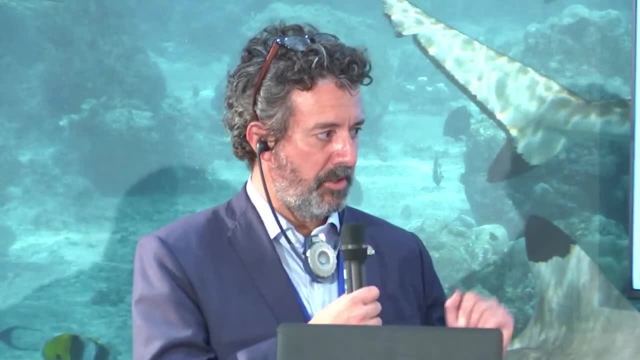 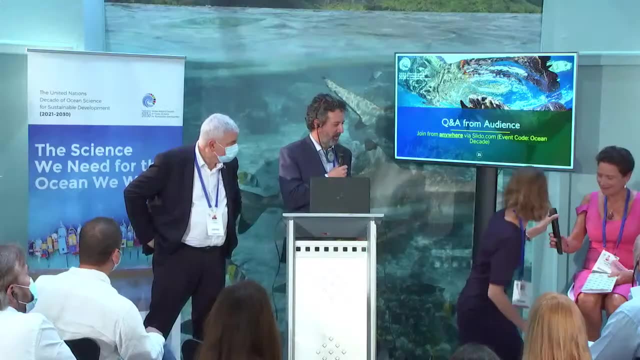 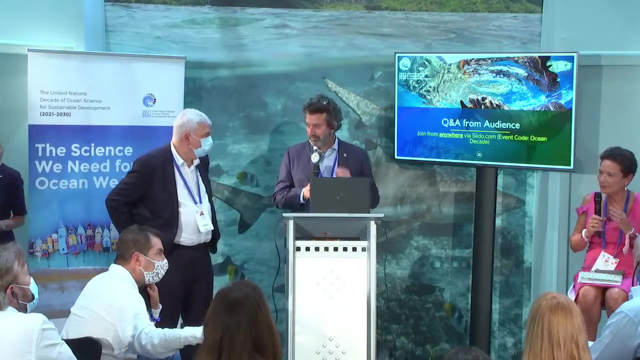 Thank you. So, mission Starfish, I see I have a client here. So Geneviève will make the link between the decade and the prioritization. Thank you very much. I think Vladimir is already open, But there is a strong similarity between the ocean decade. 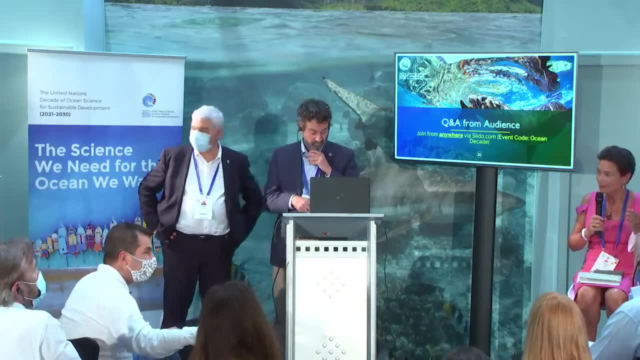 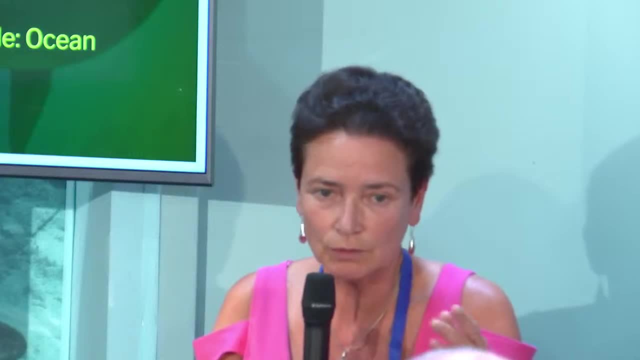 that has been launched at international level, and the mission on restoring ocean and waters that has been launched at European level and that has led to the adoption of the Starfish 2030 mission report. François Galgani. François Galgani from IFREMER. 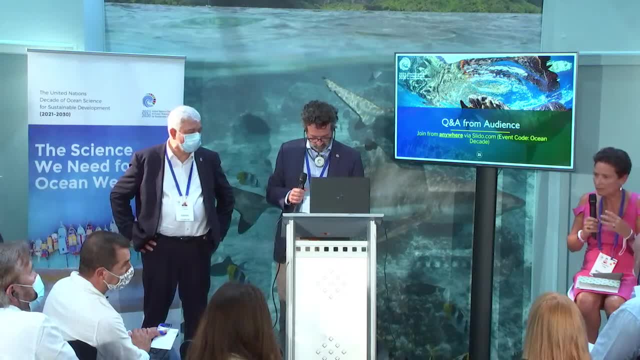 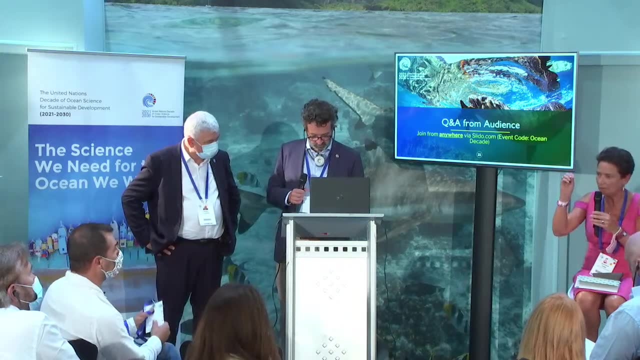 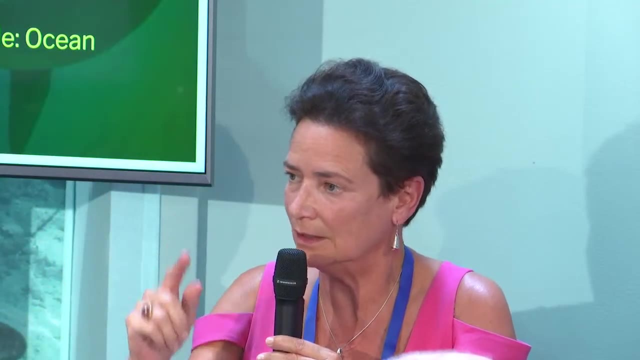 is part of this, of the team that created that, And we have called our report Starfish 2030, because we have a central objective, which is restoring our ocean and waters, And then we have five ways to get there, And one of the main ways 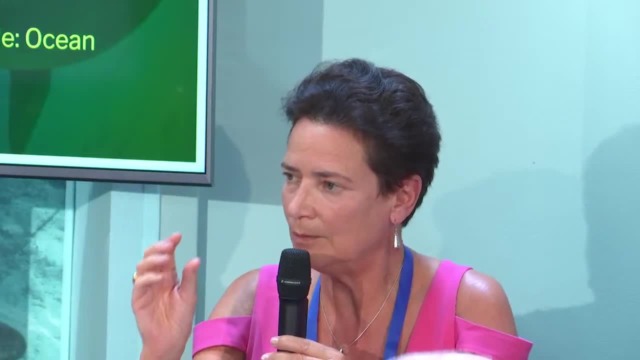 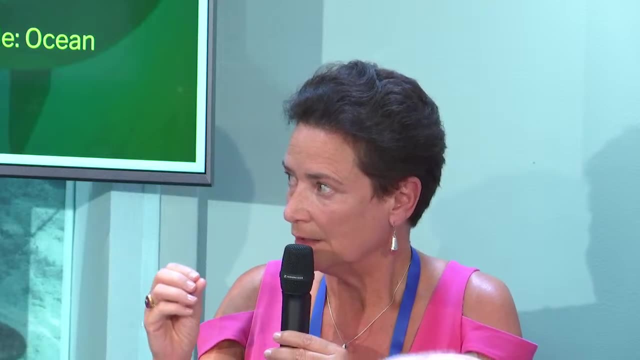 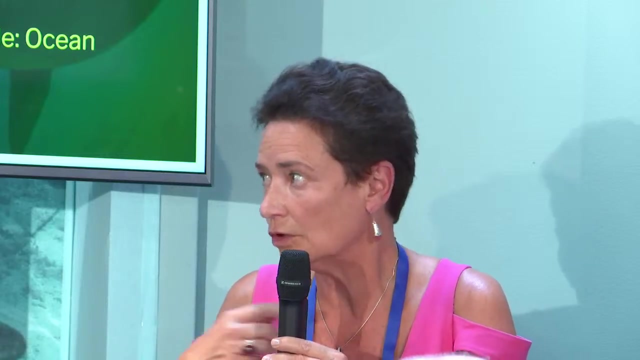 that we could call the first way absolutely necessary is to fill the knowledge and emotional gap. It's far from our sight sometimes, ocean, and far from our heart. Not for me. I was born nearly in the ocean and it is deep in my heart. 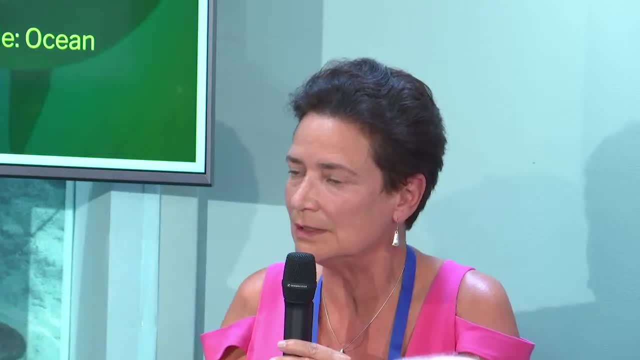 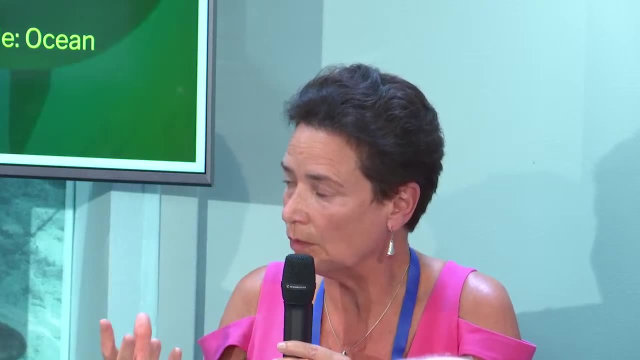 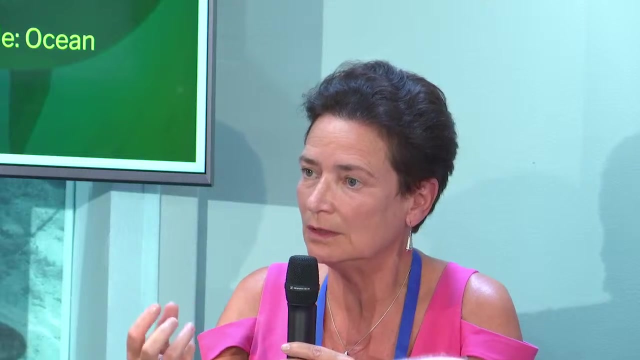 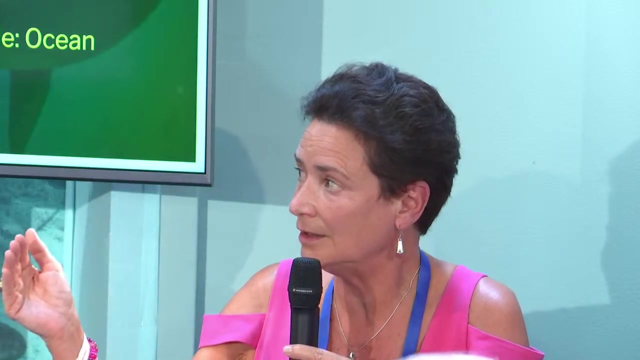 But this is not the case of everybody, And science shows that the emotional gap is most of all a knowledge gap. So one of the main aims of the Starfish 2030 mission will be to fill this knowledge gap. So we are fully in line with ocean decade. 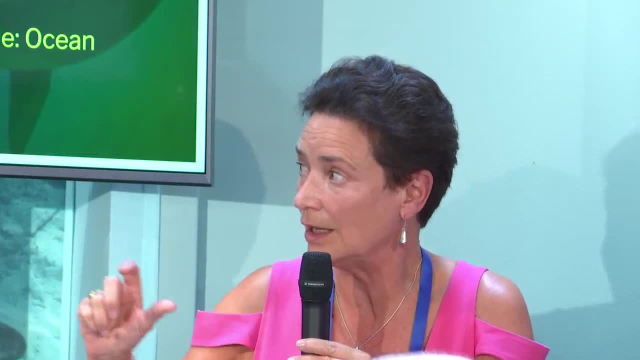 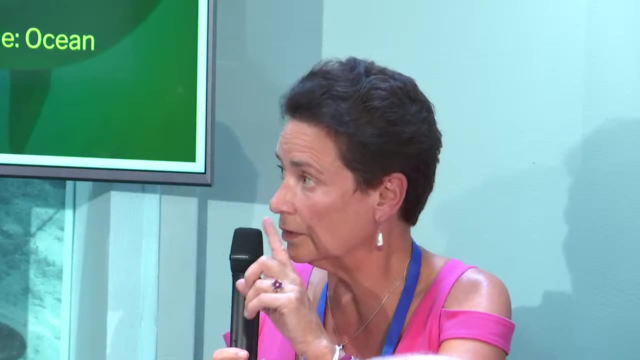 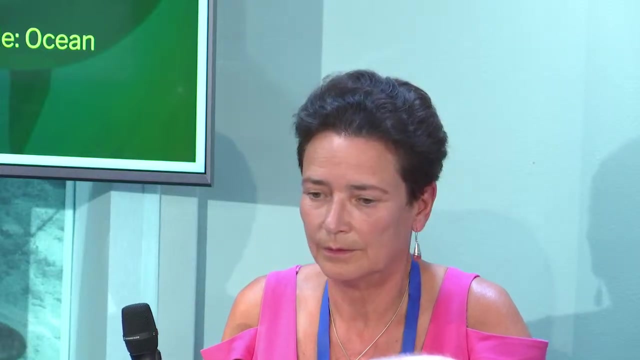 not only for the timing- because our aim is 2030, but also for the core objective. So we need to work together. Great, thank you very much. And, Birma, I have a question here which relates to data, which is also an essential element. 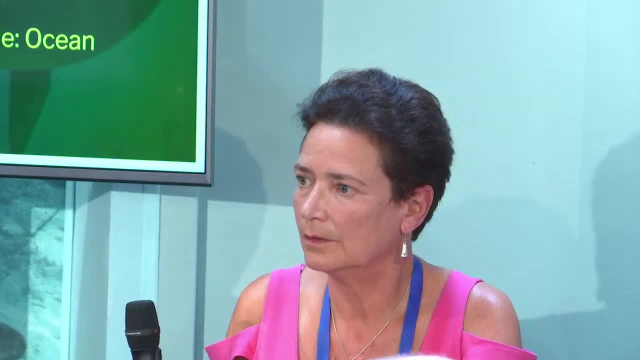 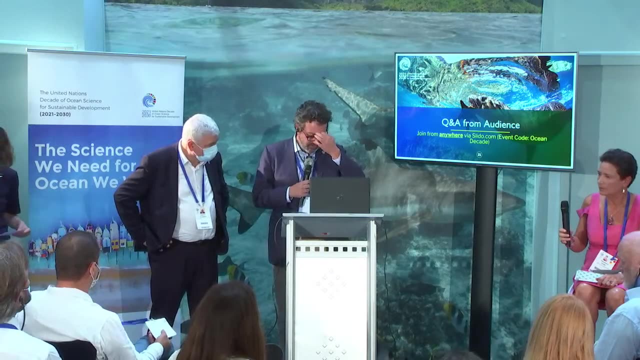 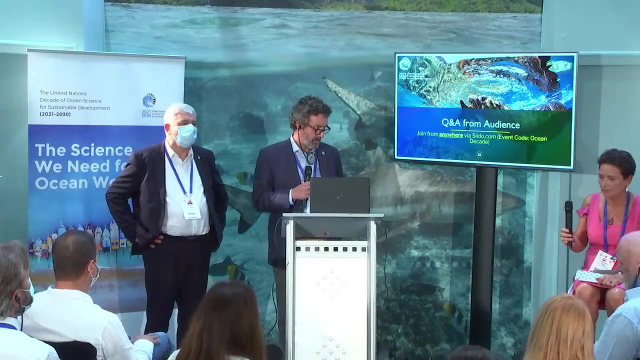 We know that there's a lot of data out there which is not being used, which is sitting in drawers and databases. So what digital or data-related actions are really needed to enable the transformation that the decade is trying to achieve? Maybe Guillermo or Mathieu? 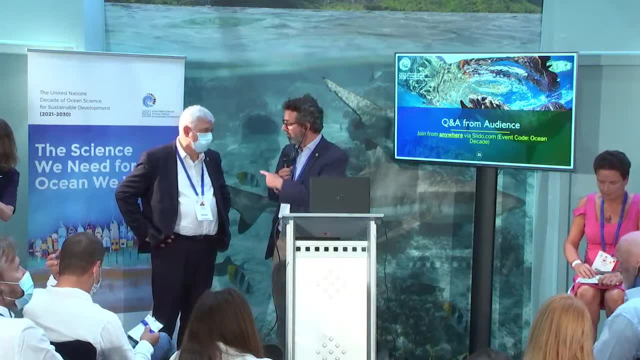 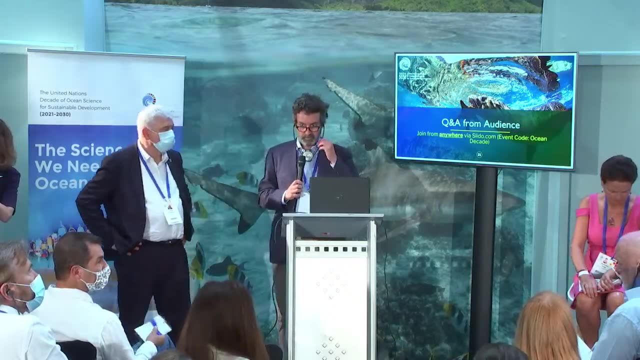 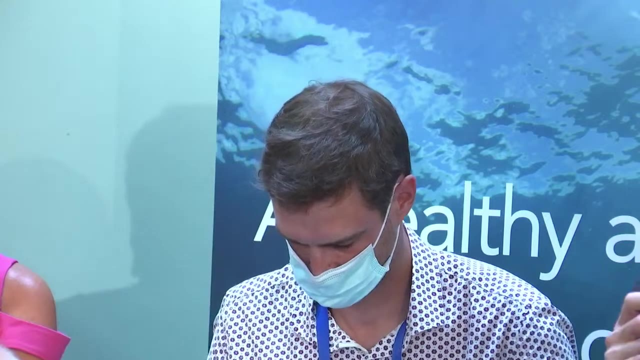 would you like to give some ideas? Just some brief comments, sort of reflecting on some of the previous comments I made. I think there's a need to connect existing databases. Sometimes the most attractive thing is to find a pot of money to coin a new acronym. 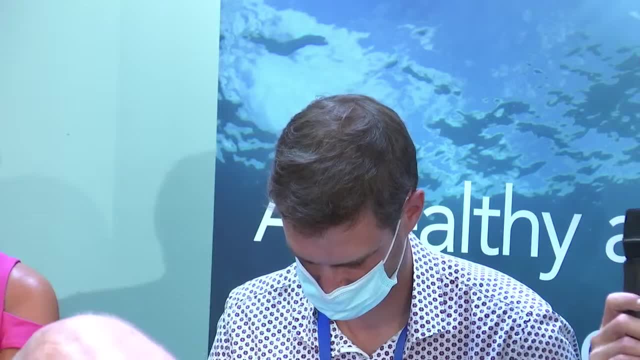 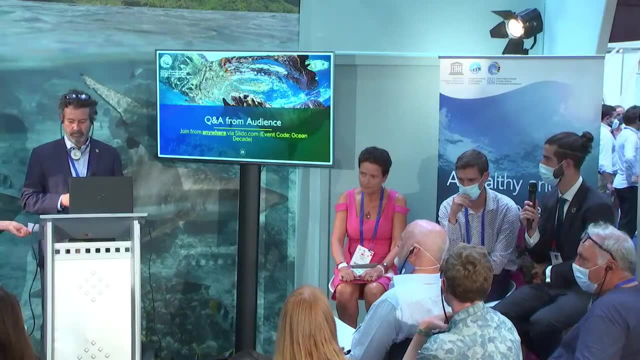 We are drowning in acronyms. We have plenty of acronyms. we have plenty of intergovernmental international data repositories and we need to maintain those Right now. the Ocean Biodiversity Information System, which is comprised of geographic nodes. 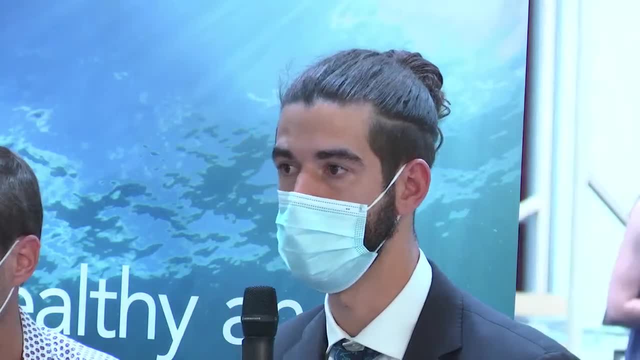 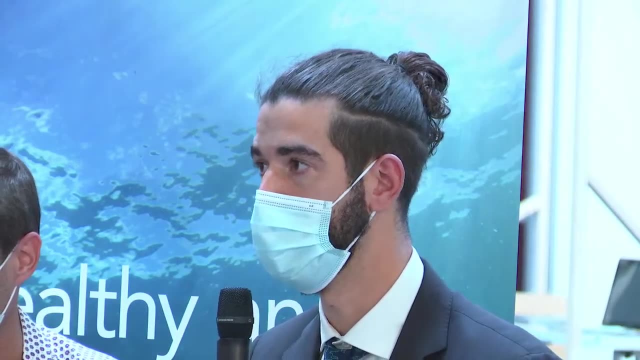 and thematic nodes is severely underfunded, So I think that funding the infrastructure that we've already created would be a good first step. But also, like I mentioned, OBIS doesn't have access to a lot of existing data that is housed in hard drives. 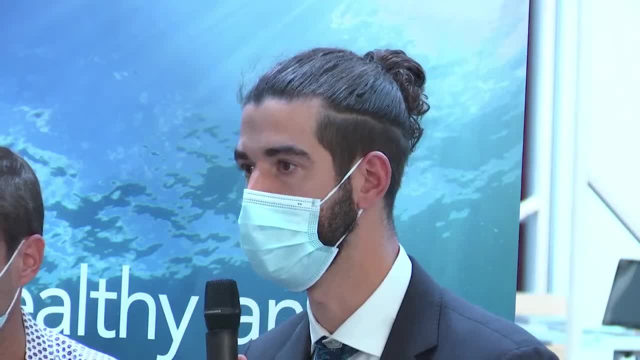 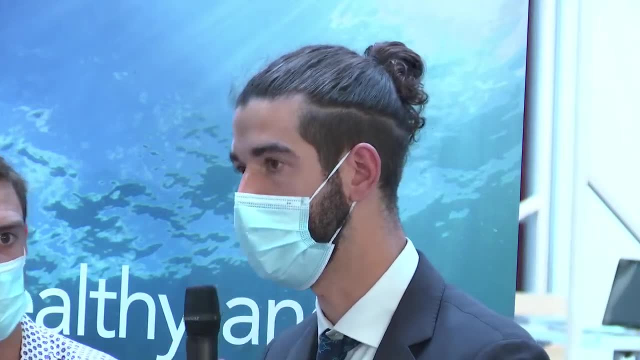 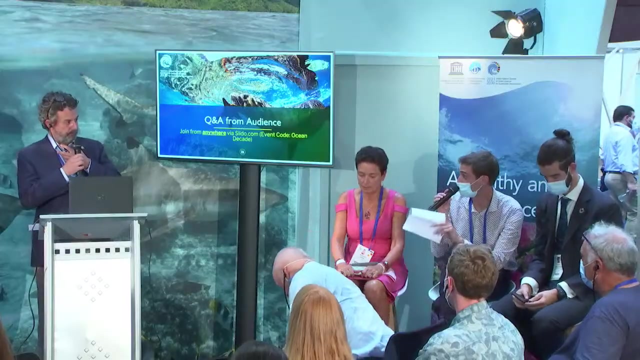 within national governments, within intergovernmental bodies. So let's align what we already have and then we'll have a much clearer understanding, geographically, taxonomically, where the decade can invest its resources. Thank you very much, And maybe just to add one point on this: 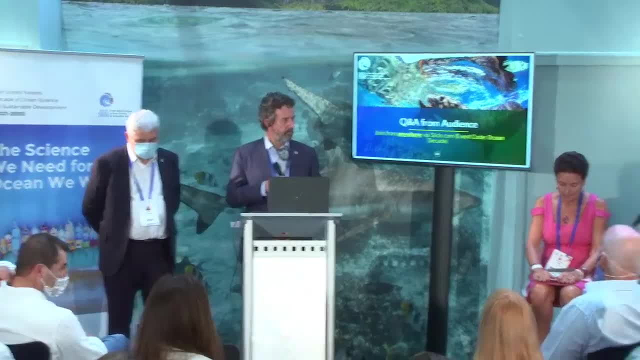 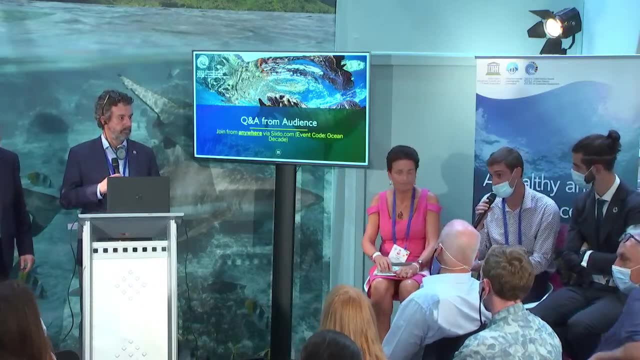 it's not only we need more data, it's also we need this data to be shared more equitably, because at this point in time, marine knowledge is not equitably shared, And this is of particular concern when a lot of coastal people 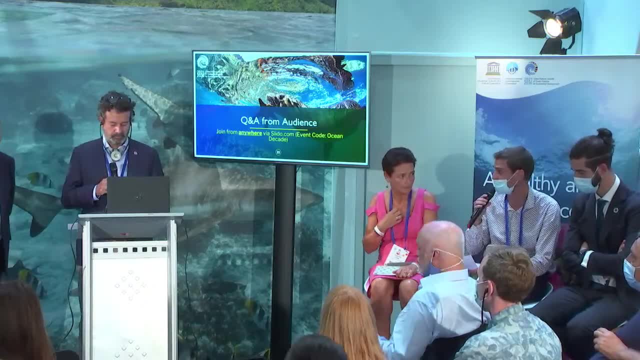 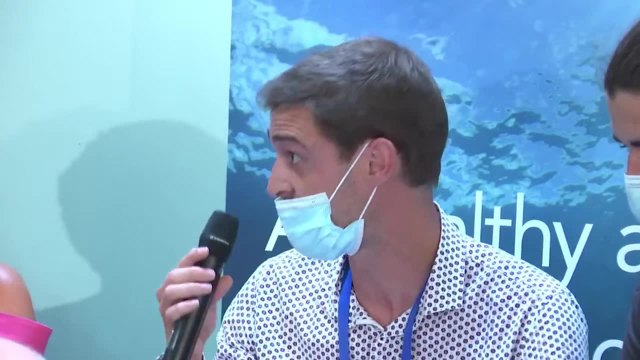 and especially in least developed countries or small island developing states, are the ones that are the most in danger in future changes of the ocean, So we need this data also to be more equitably shared so to be able to reach a lot of people. 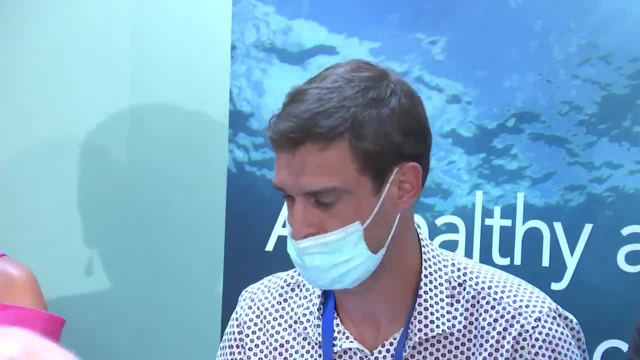 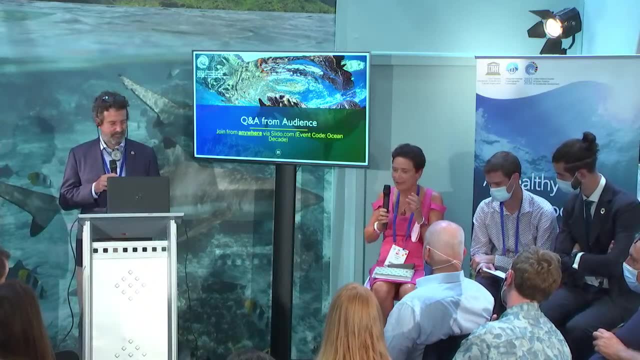 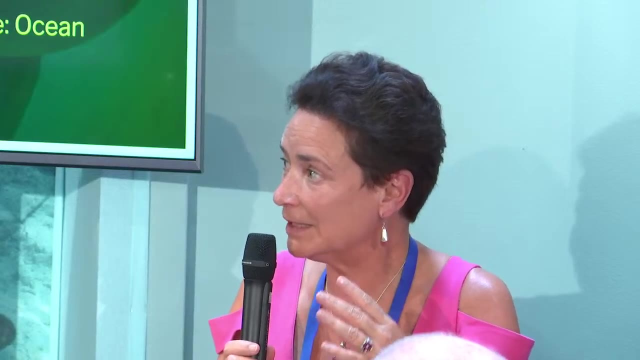 in a lot of countries, And I would like to add that we propose a digital twin of the ocean and waters, And this will be common knowledge, but also commonly built knowledge, And we will develop applications that will allow people, citizens, to take part of this knowledge building. 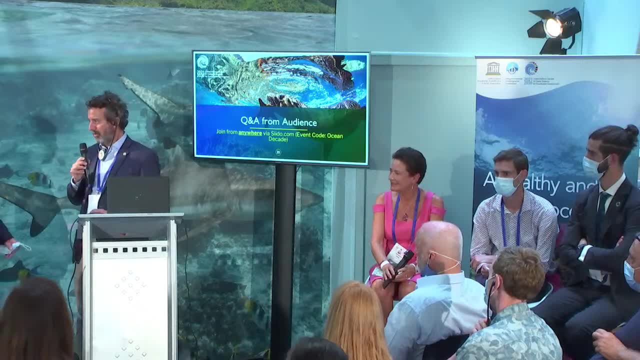 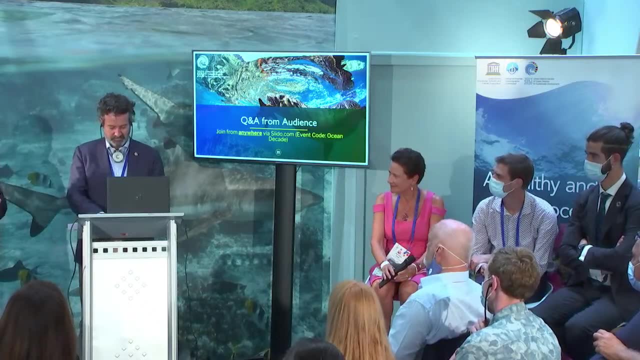 Let me also ask Vladimir, who also has his vision of what the data should be. You know, I think my response will be quite peculiar because I haven't heard the question, I haven't heard the previous answers. The only thing I know is that what Julian said. 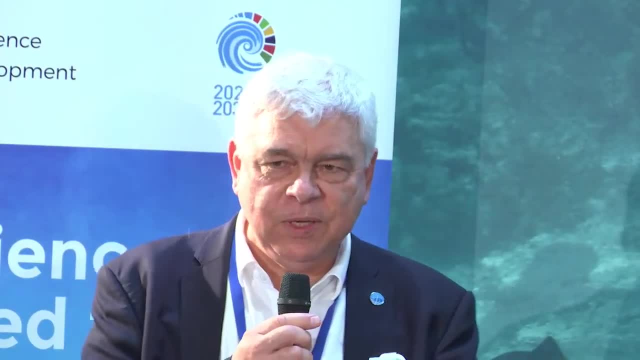 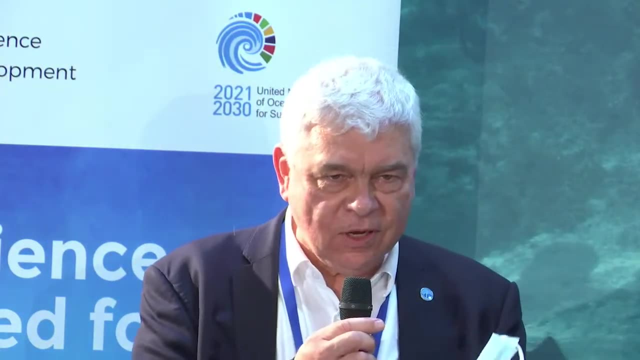 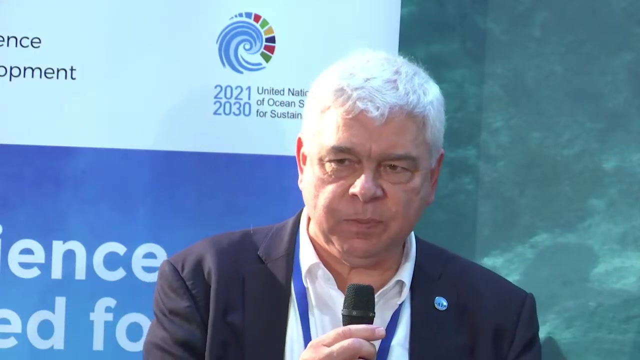 And this is exactly an illustration of that. people need to know to act, But sometimes you don't need, So the situation is that it's not only the quality and the quantity of the data that we need. The data makes all decisions much more transparent. 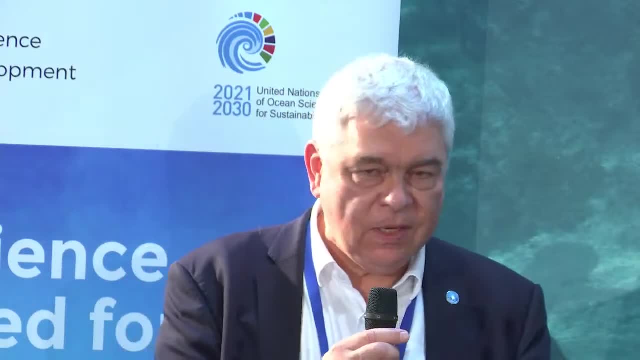 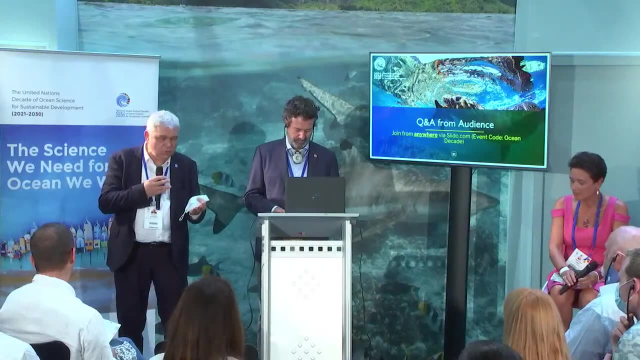 Excuse me, this world is corrupted And decisions are taken not because of the objective reasons, So we have to create a data system that brings to the decision makers not only the chance to take good decisions, but also to be verified on those decisions. 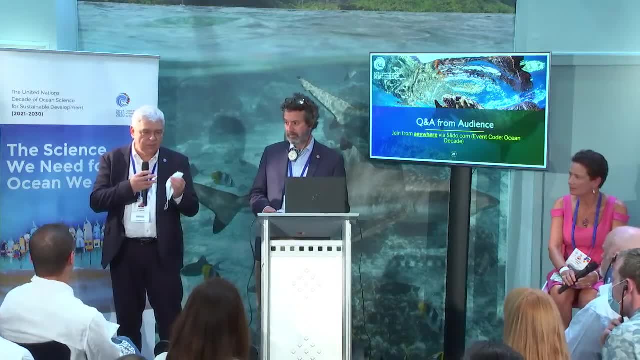 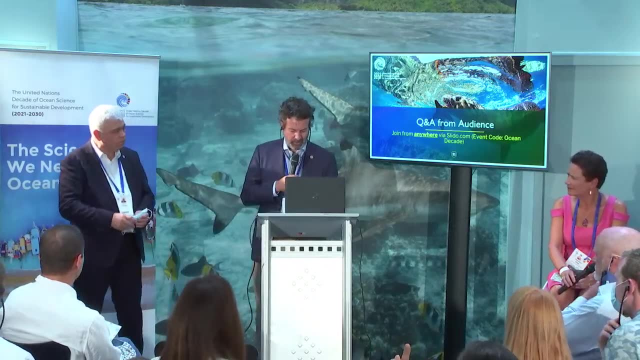 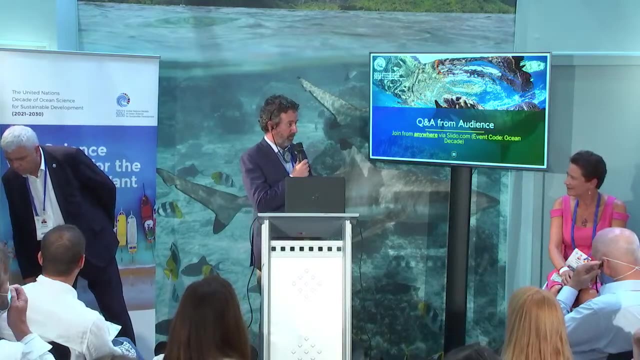 And the science can do this. That is the best answer to this question, I think. Thank you, Thank you very much. Another question I have here: How will Decade actively support co-design? That's something I'm not allowed to answer the questions. 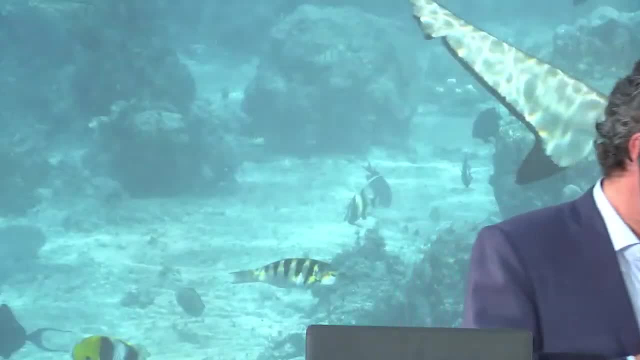 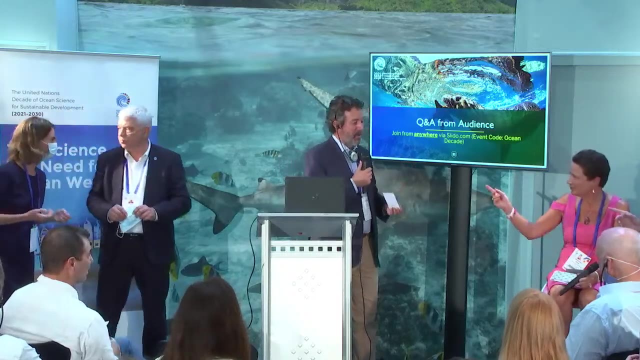 How can, How will Decade actually support co-design? Well, no, I know, but I'm the moderator so I can't do it. We have to play the role here. Alison, do you want to talk about co-design? 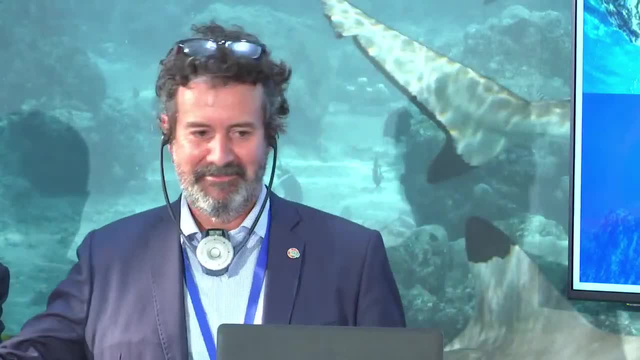 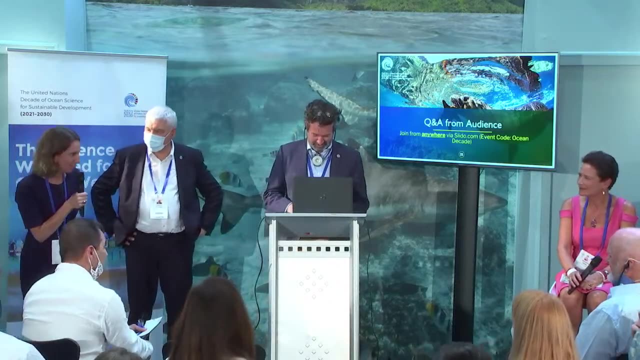 How will Decade support co-design? Thank you, I see I got thrown that question, Okay, So I think you know we have some fabulous partners. We have the Ocean Voices program. We have several other endorsed Decade programs that are really focusing on this issue of co-design. 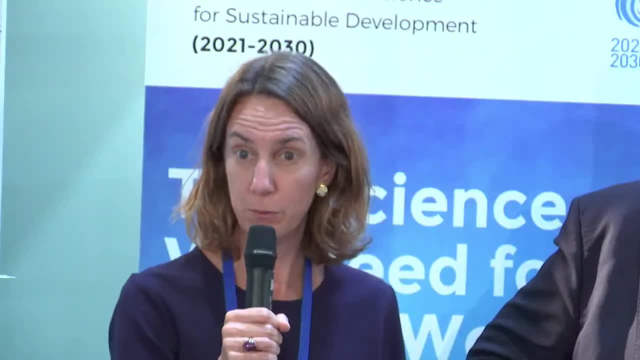 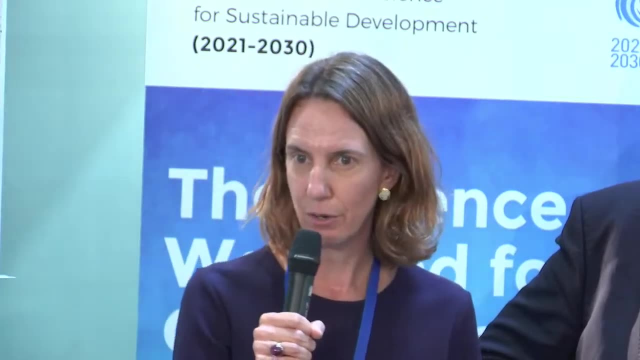 Last year we had a series of six or seven regional workshops, webinars and some global sessions that started to look within each region. what are the obstacles and the barriers to co-design? And a lot of it just comes down to understanding what co-design actually means. 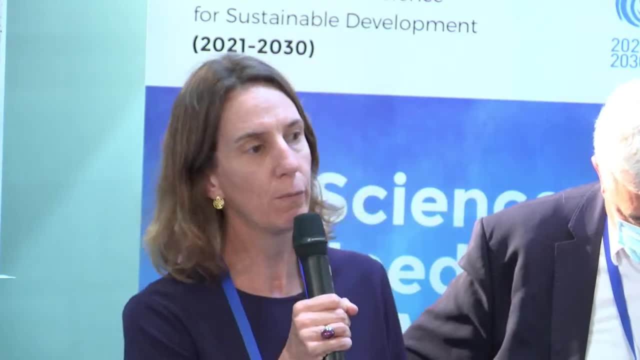 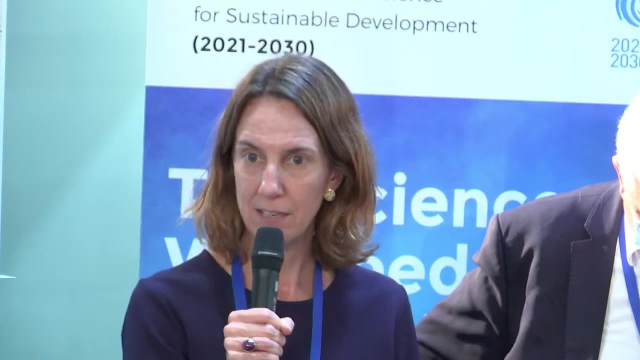 Because when you break it down it's not that complicated. So we're developing some training courses. There will be curriculum on an online platform, the Ocean Teacher Global Academy, towards the end of the year. that will gradually be adapted to different regions. 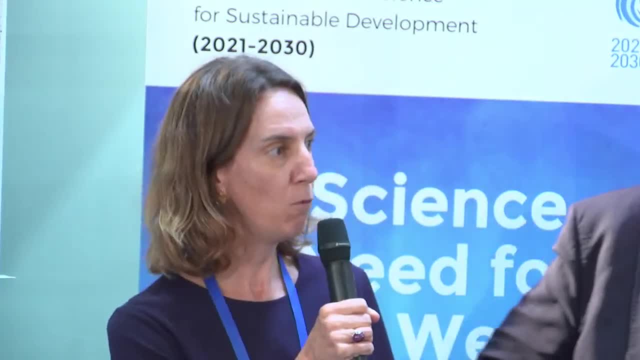 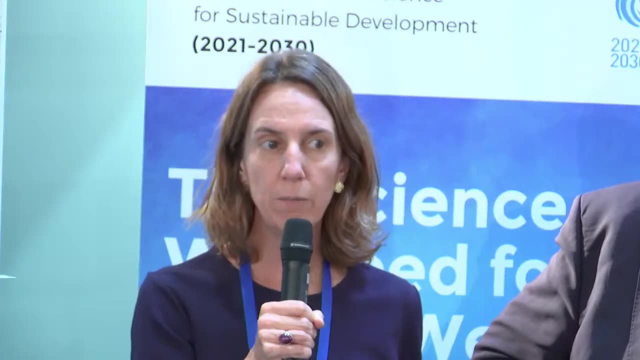 to different languages and so on, so people can start to learn. And then we'll be working with partners such as the Ocean Voices program to build on that training program, to do some publications where we're working with partners, to also mobilize resources for seed funding. 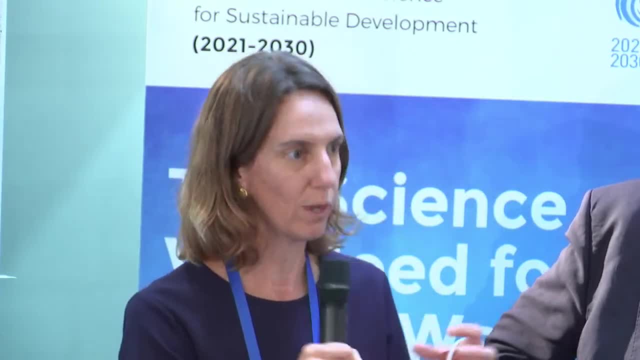 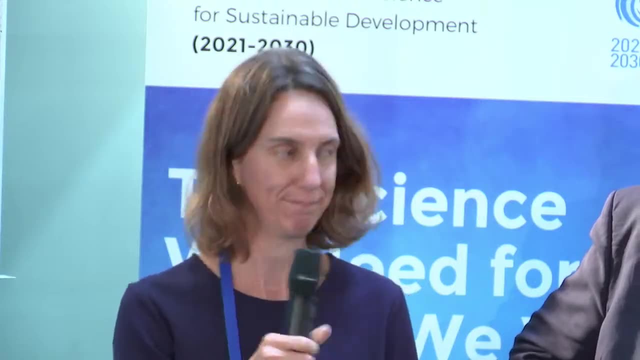 so that groups can come together, groups that wouldn't normally talk can come together and incubate different resources And incubate different actions through co-design processes. So about capacity and bringing people together. And while I have the mic- because I stole it- 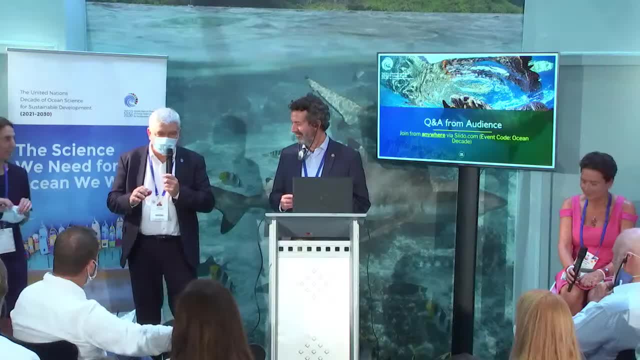 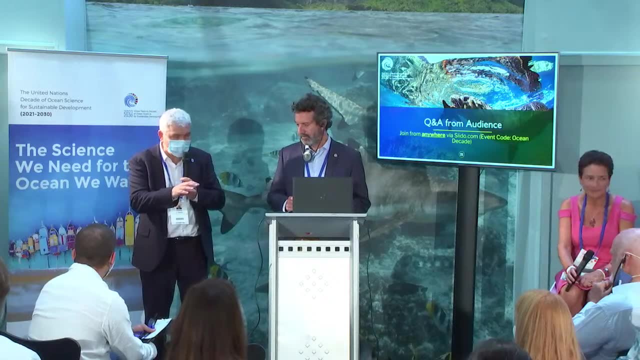 so I would like to say one important thing That you know: we are bringing together people, We are bringing together you with your understanding of the mother nature and what needs to be done. This co-design is enabled by the decade and there is a movement. 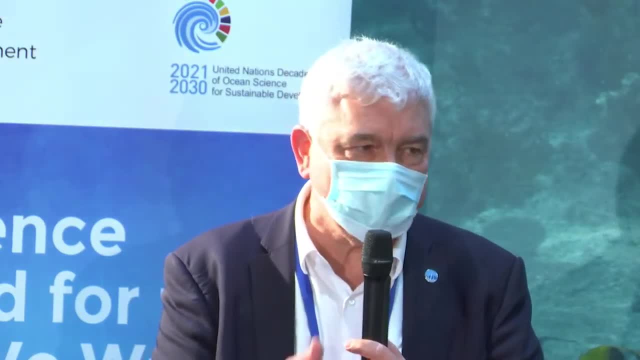 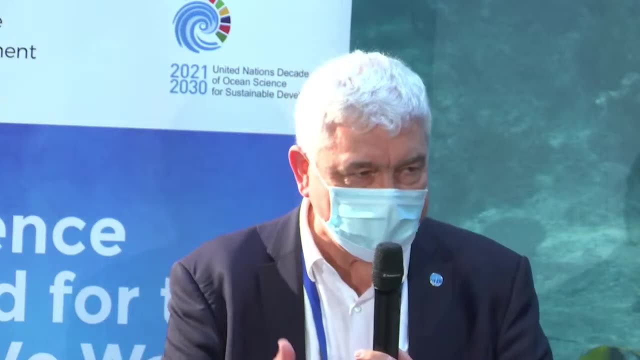 So everyone thinks about how to live better with the ocean, and for the ocean And for the future, And that is manifested also in science, And that is the co-design we would like to achieve. Bring everyone on board And, if I may add a piece of information, 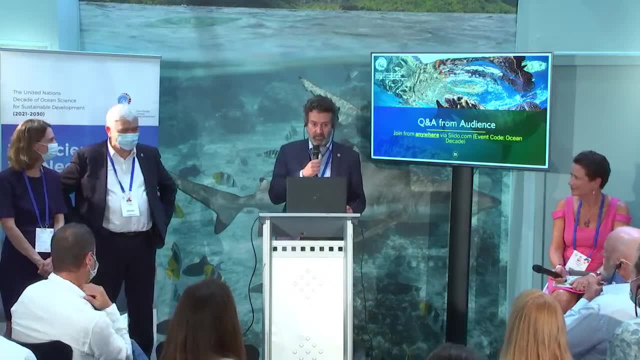 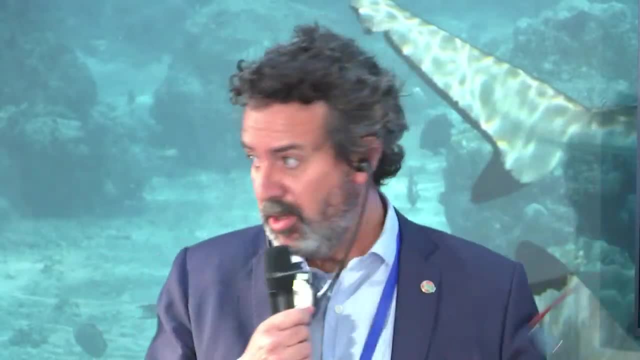 we do have regional and national mechanisms for co-designing. We have national decade committees that are being established around the world. We have 25 decade committees that have been established in the US, in Latin America, even in Africa and in the Pacific. 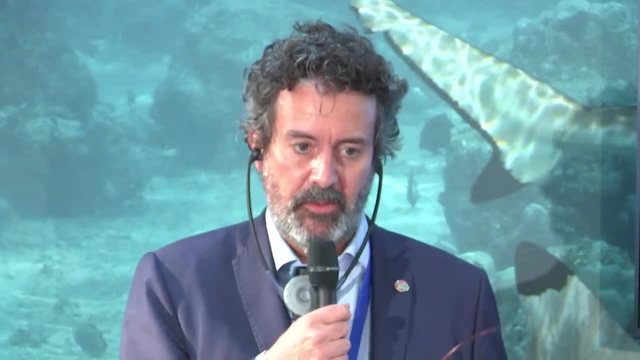 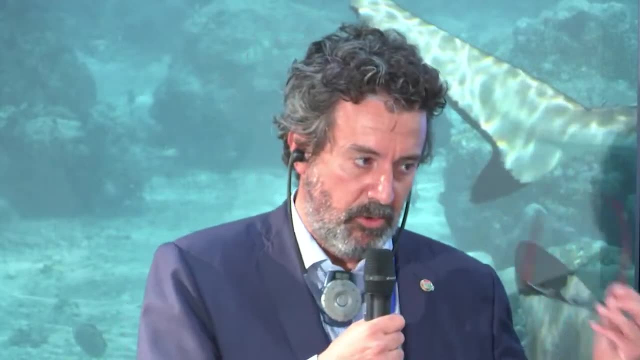 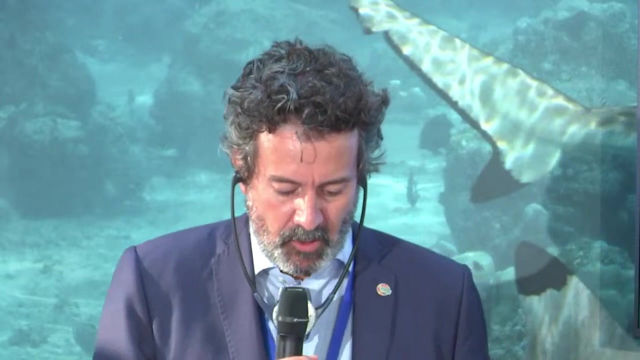 So those are also fora for discussing and identifying the scientific needs. We have regional task forces, Working groups Working in the Mediterranean region, Working in the tropical Atlantic region and the South Pacific, So you can join and be part of that discussion. We are coming close to our event. 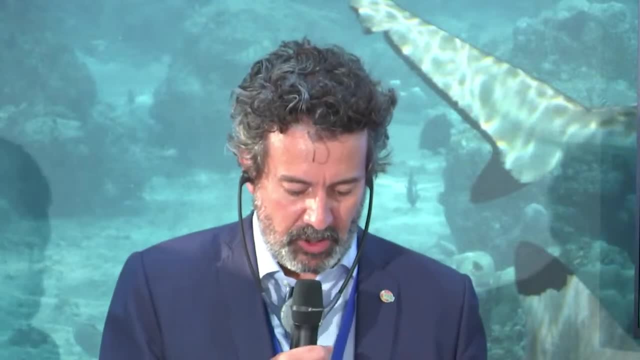 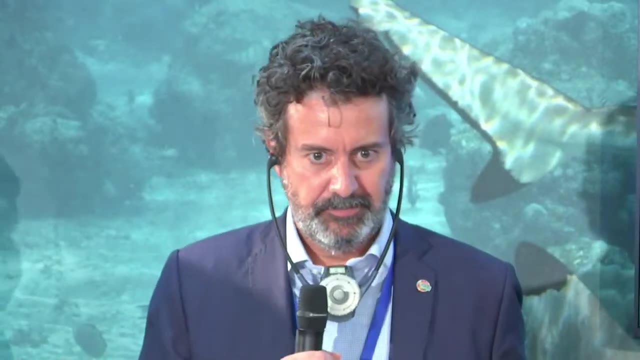 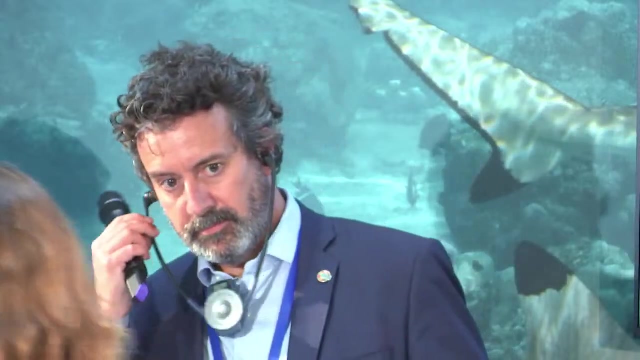 I see we have one live question and one last question related to ACOP, So let's go to the live question and then we'll wrap up and give a floor to Peter Thompson. Thank you, Good afternoon. I'm Dr Antares Ramos from Puerto Rico. 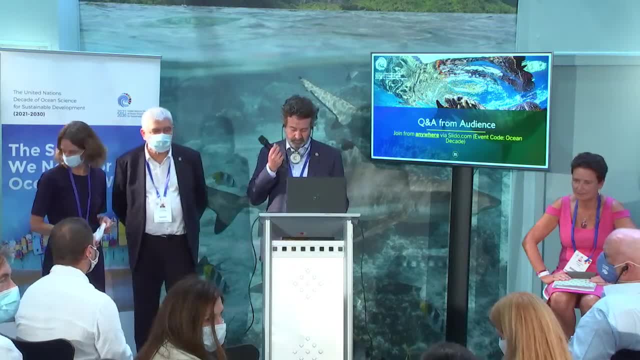 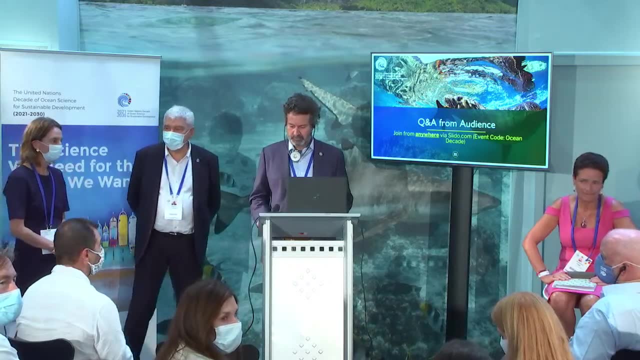 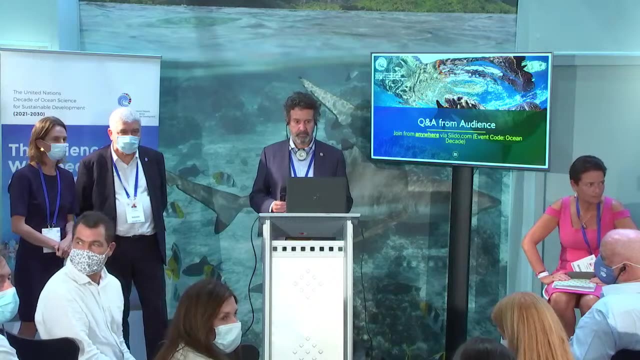 I'm a marine ecologist by trade, Also a social scientist For the last 20 years. we keep on hearing how we need to have more social science involved. We keep on hearing about we need more data. Our audience member here from Germany said we have enough data to actually start starting. 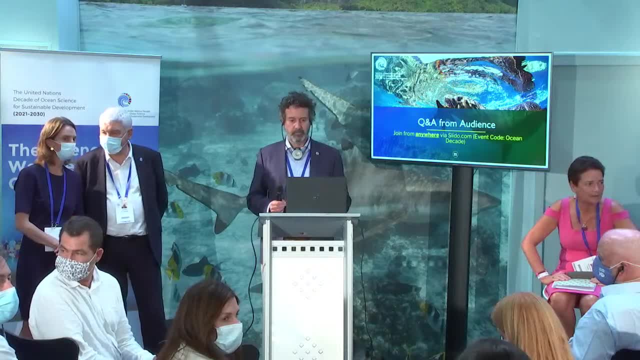 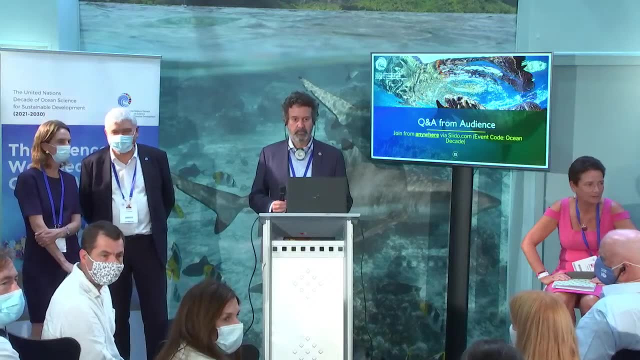 An issue we have in Puerto Rico is we have enough data, at least for coral reefs, for example, But the population It's really hard to keep up, It's really hard to get the message across, Being even an island, So it's a great example. 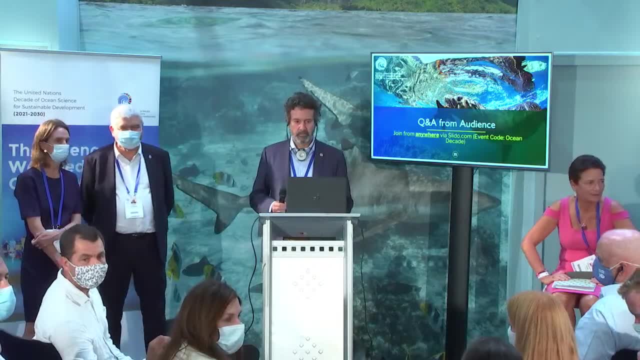 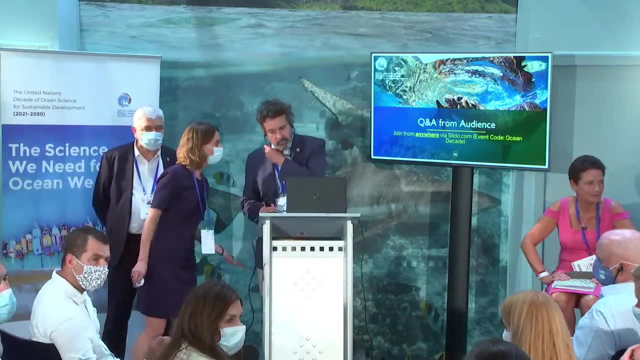 What? and I guess my question is: do we have any big picture groups or, you know, is it part of the conversation? You know, we have the policy level, We have all the regulations in place, at least in Puerto Rico. 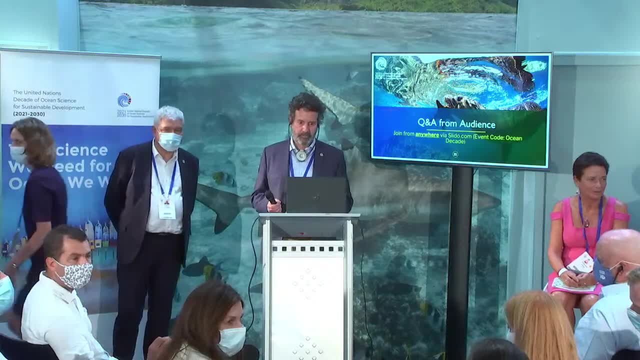 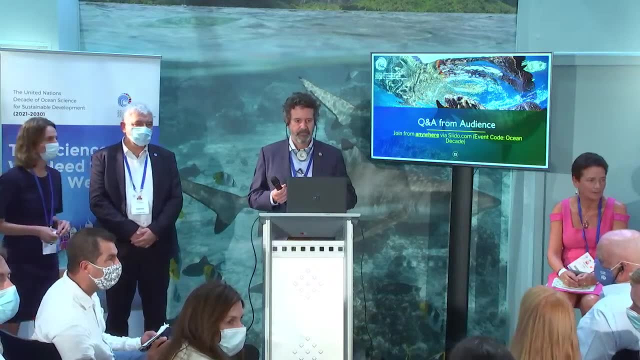 But then we can never get to the right audience, We can never get the message And we have that disparity between the scientists, the technical talk and then the day to day. So I guess I would love to hear a bit more about that. 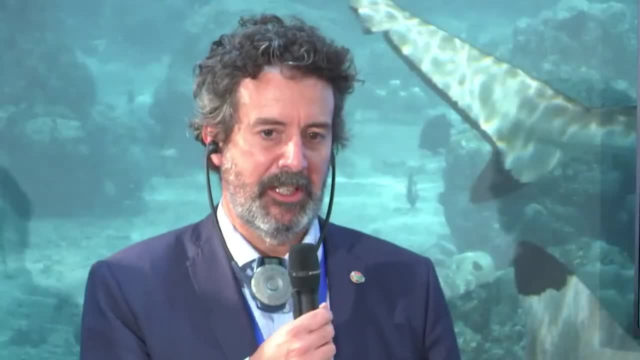 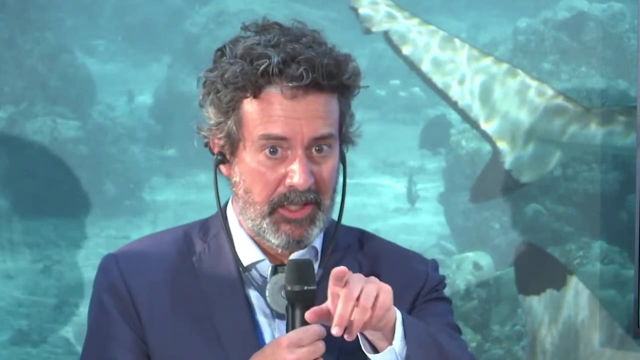 Thank you. Thank you very much for this question. Unfortunately, we need to wrap up and we need to give a floor to a special envoy, But please stick around. At the end of the event we can certainly, you know, interact and try to give you some answers. 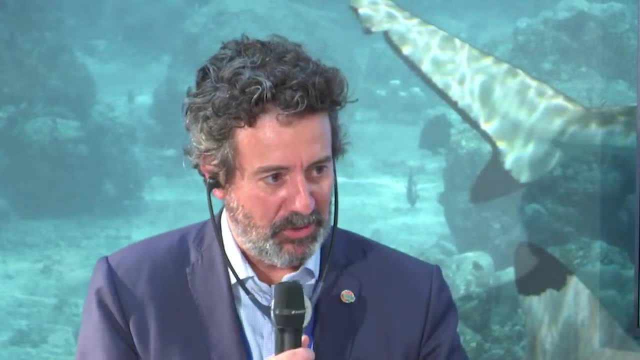 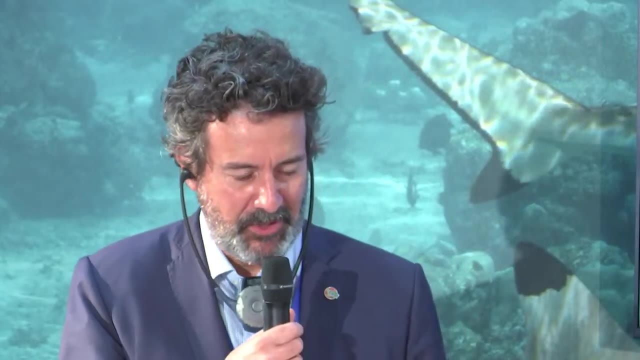 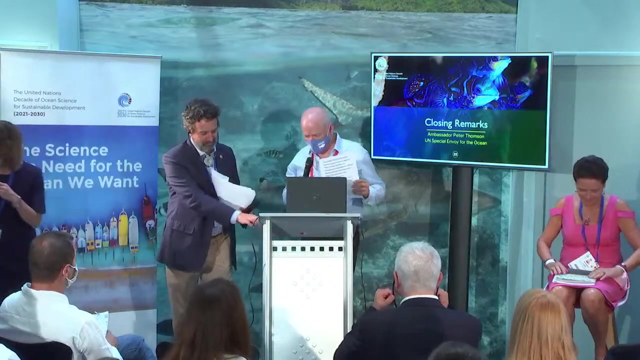 So with this, it's my pleasure to invite Ambassador Peter Thompson, UN Secretary General, Special Envoy for the Ocean, for a concluding remark on this event. Peter, over to you, Pleasure to see you again. Okay, I'll just do my advertisement first. 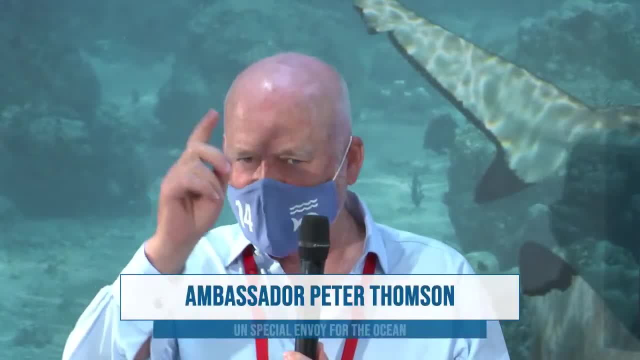 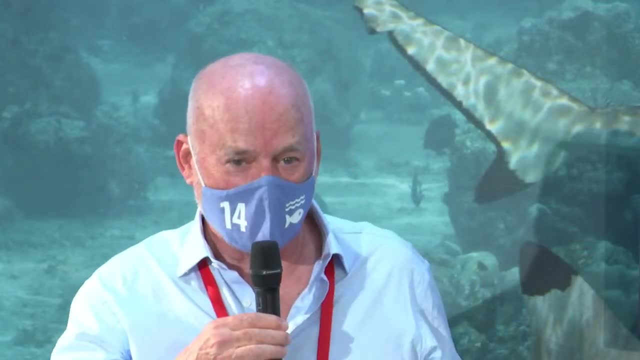 But the lady from Puerto Rico, where are you There? You know, I think the media, The media has to start getting responsible about ocean work. I had a meeting with BBC, last week actually, where the BBC was agreeing with me. 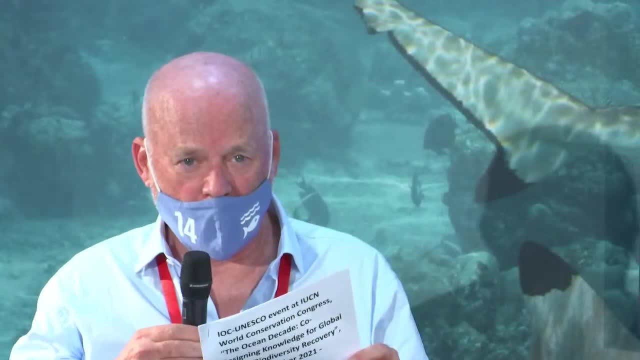 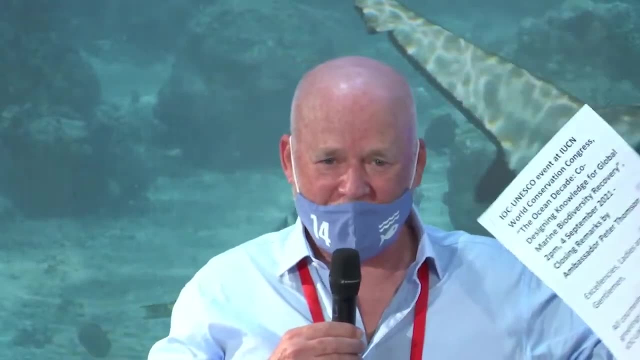 Being a blind spot for them. You have to engage your media and get some champions in the Puerto Rican media. So that's to answer that. Look, I made a very nice speech before I came down here for this event- down here for this event. it's a beautiful speech and i'll give it to these guys. 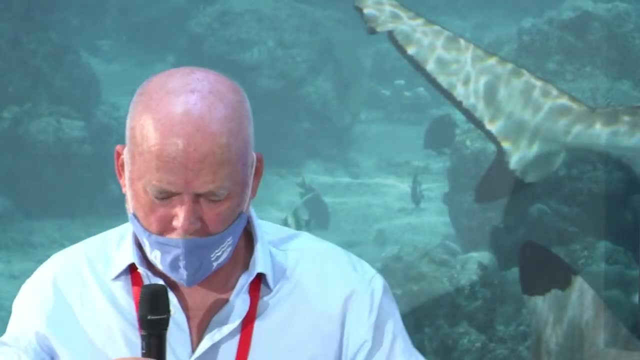 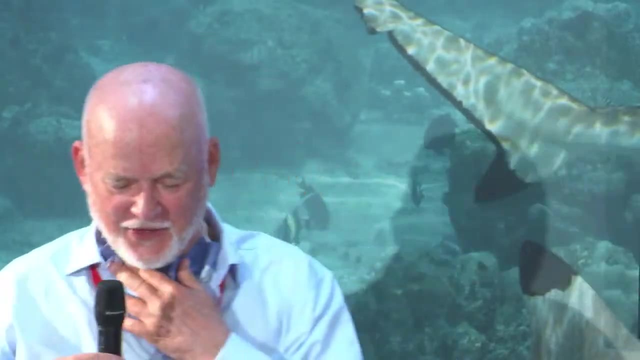 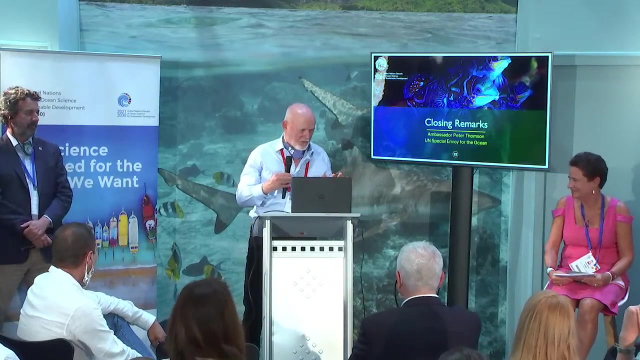 so i think this is more of an interactive stage, and you've probably heard enough, i think, now about the un ocean decade, and you've probably seen my branding enough, okay, so sdg14: conserve and sustainably use the ocean's resources. all of our countries have agreed to it in 2015. 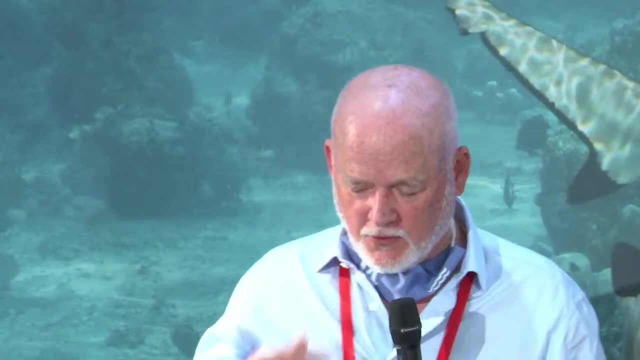 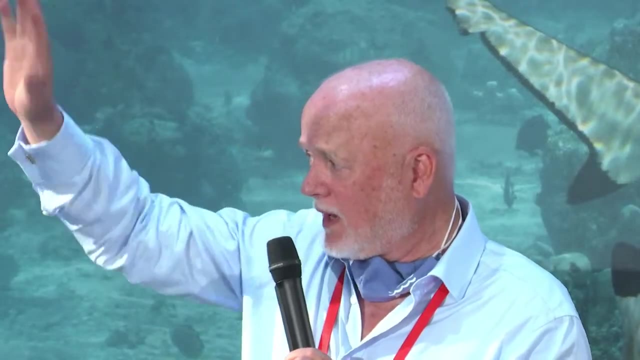 our job is to implement it, and so that's my job as well. so look, first of all. uh, allison, you better start jumping up and down when i've had my five minutes. okay, because i got no watch and no sense of time, and it's hard to turn an ambassador off once you turn him on. 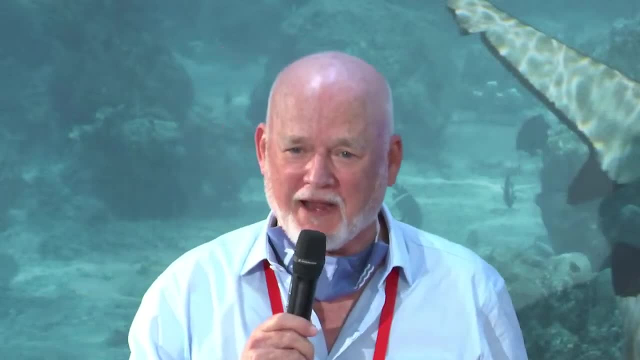 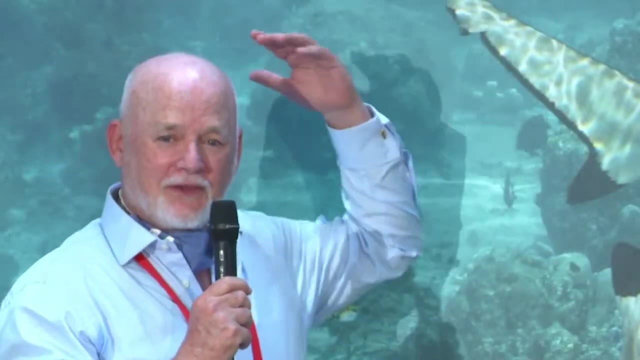 so maybe if you all leave the room when you've had enough, i'll know to stop speaking, but i want to just thank the organizers for putting this up. this is my home. this is where i'm born, this is where i'm brought up. i don't know what island this is, but i come from few. 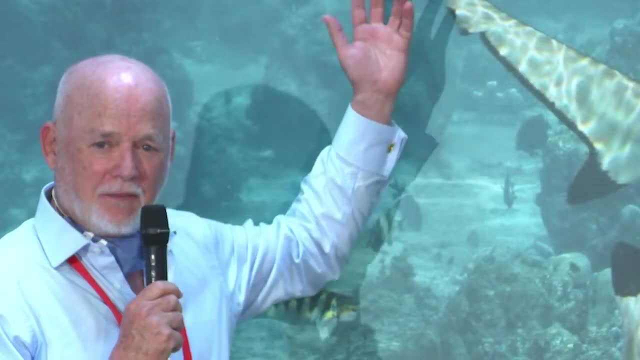 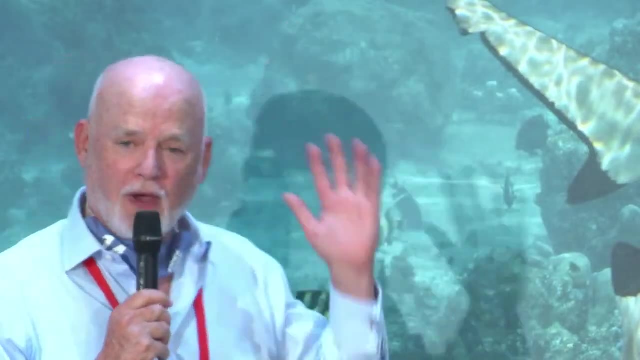 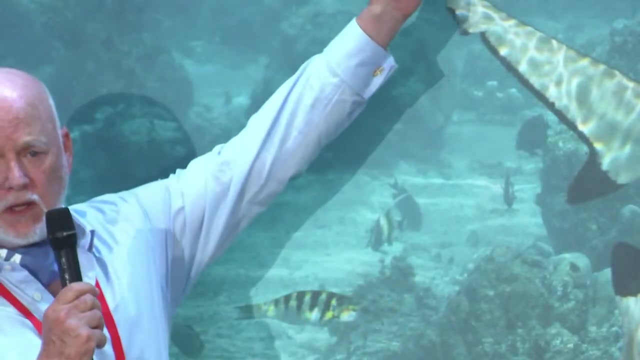 years ago. i'm from fiji. i'm a fourth, fifth generation fijian, my granddaughter, who is in my arms every morning. one of her ancestors is been living in these islands for four thousand years and this down here is our garden right. we played as kids in the mangroves in our tin boats. 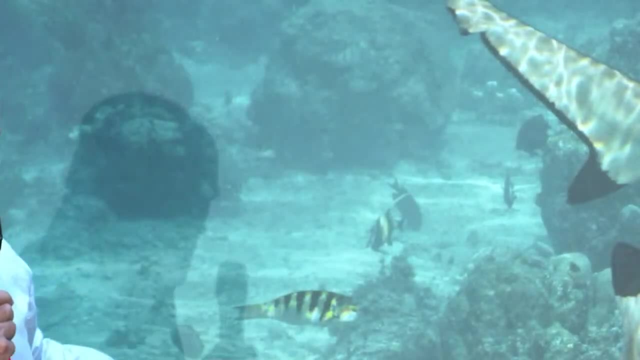 i spent a bit of time on the beach, not too much. this was our playground, what you're looking at here. as soon as you could swim- which is, you know, four years old- and get a mask on, you came and you get a mask on. you came out of the back yard and i can tell you that the healthy coral reef is. 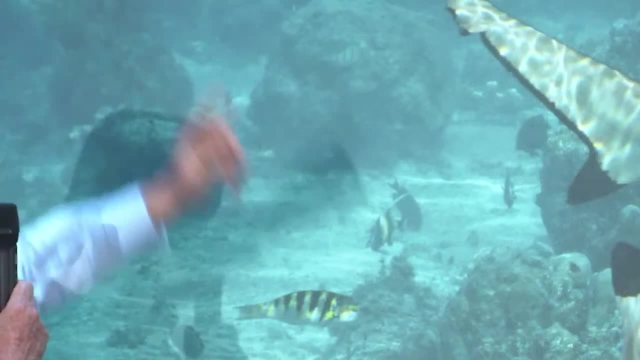 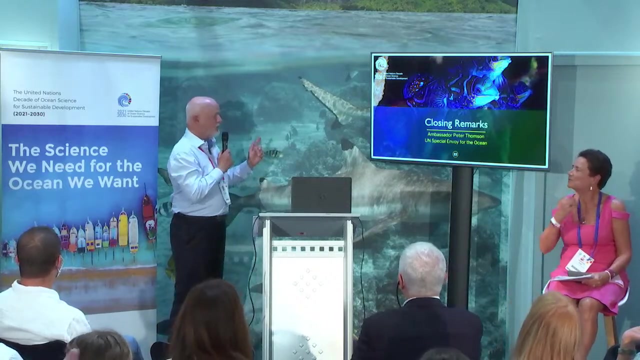 100 times more colorful than what you're seeing here. maybe it's a cloudy day, that's why the shark is in light, but it was probably put in artificially. but anyway, uh, what i want to say to you now is that so often when i go to these places now, i see a cemetery, i see the equivalent of a. 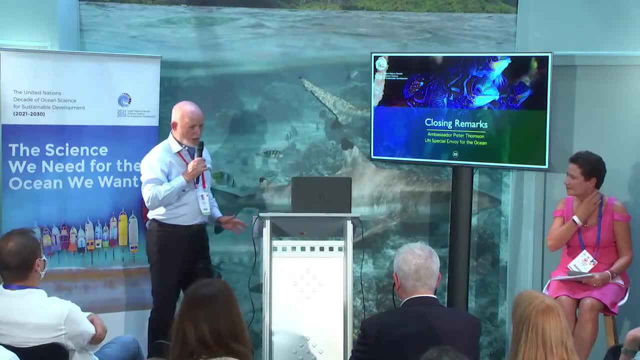 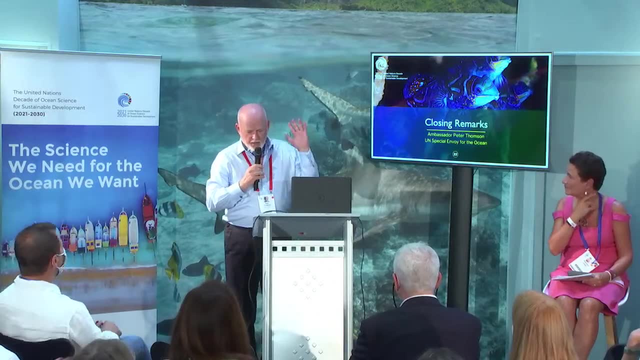 bombed out city after, uh, you know, carpet bombing or something. it's so tragic and you all know the story of coral so i won't go into that. but thanks for putting that up and giving me such a beautiful reminder of what it used to be like. and if we work hard enough will be like for our children. 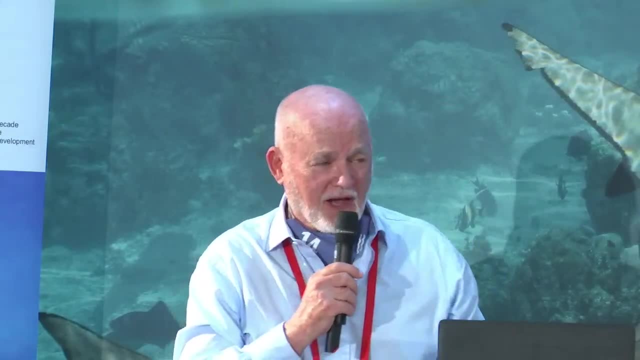 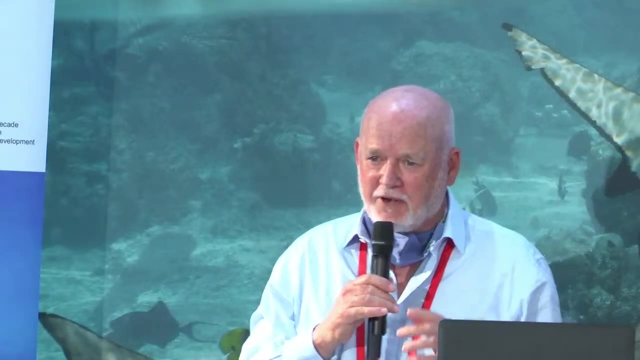 You know, one of the reasons I put my speech aside is it's pretty much what I said this morning at the opening of the Ocean Plenary, and I think most of you were there. So I did say there that I'm really here to spy on a hybrid conference. 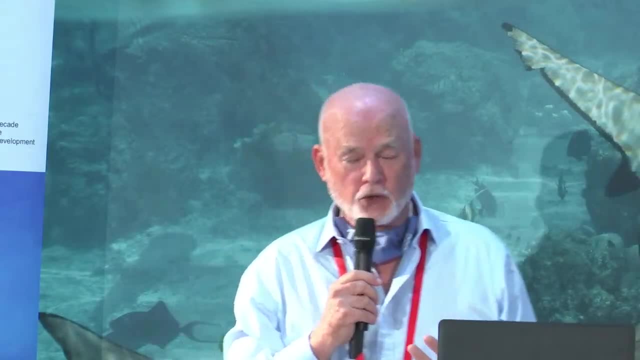 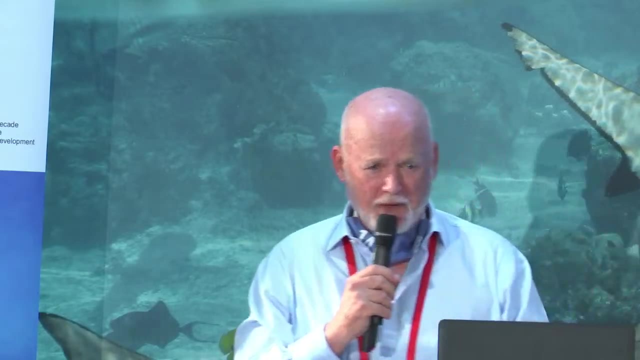 how to organize because- permit a little advertisement- the UN Ocean Conference is coming up in about nine months' time, 27th June to the 1st of July, don't quote me. it hasn't been mandated by the UN General Assembly yet. 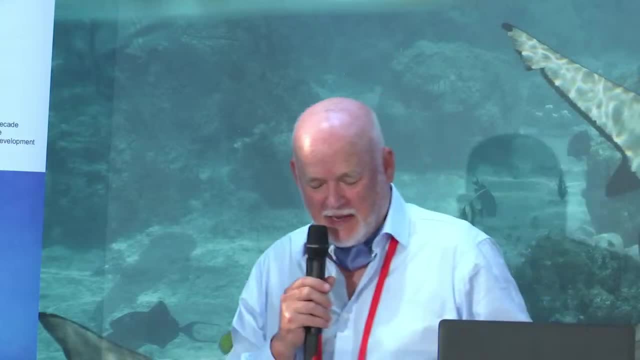 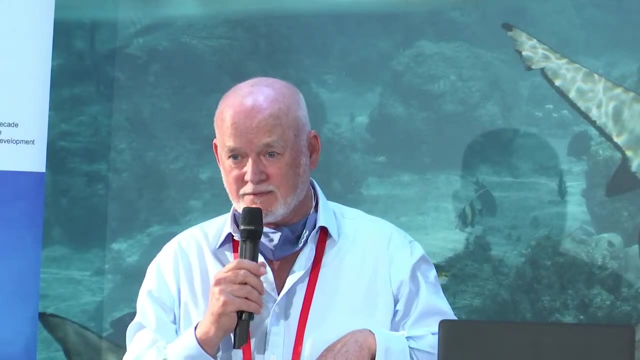 but if you work on that week you won't be wasting your time. So you know the UN Ocean Conference, one of the first things I learned, because I got lost for half an hour trying to get here and I saw this place yesterday to check very hard to find. 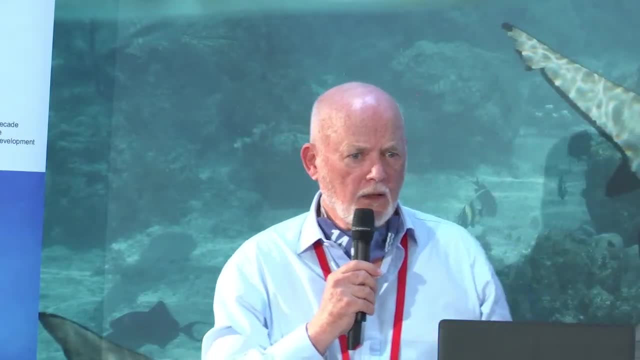 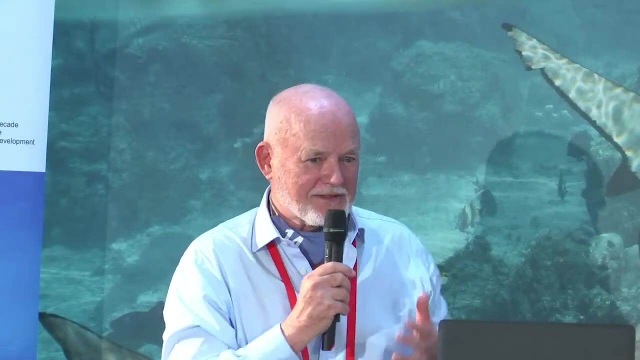 I didn't know. it's in the Phoenician Pavilion, you know. So this is, having been at hundreds of these conferences over. the first thing, get your directions. This is right for the users, us, and I apologize, Vladimir. 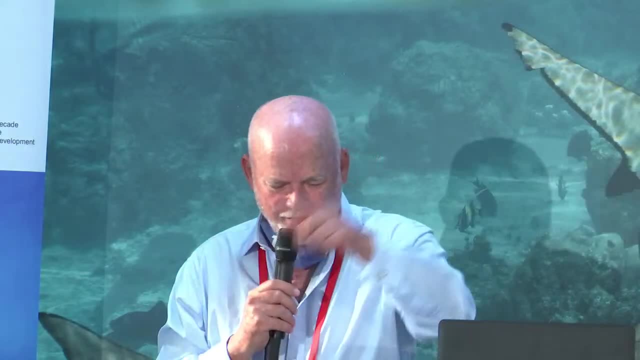 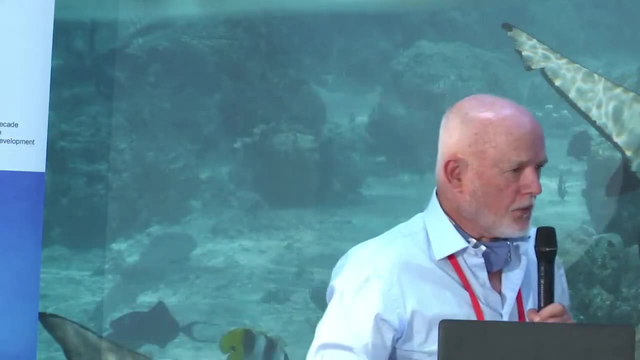 that's a funny way of apologizing to you for being so late for this event. I've been around the perimeter about five times before I found you. The other thing I'd like to say is that our host, the IUCN Bruno, said in his opening: we have two great challenges before us now. 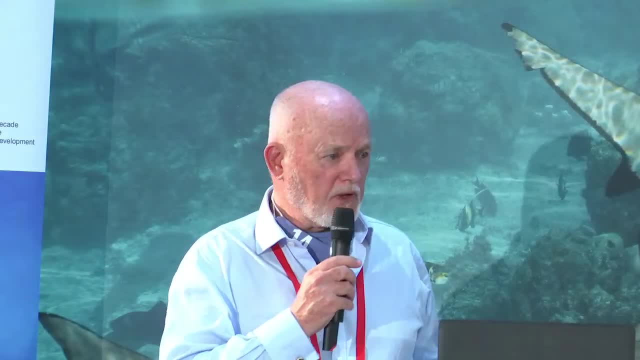 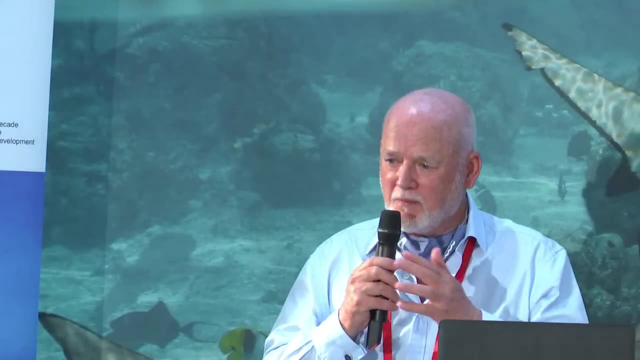 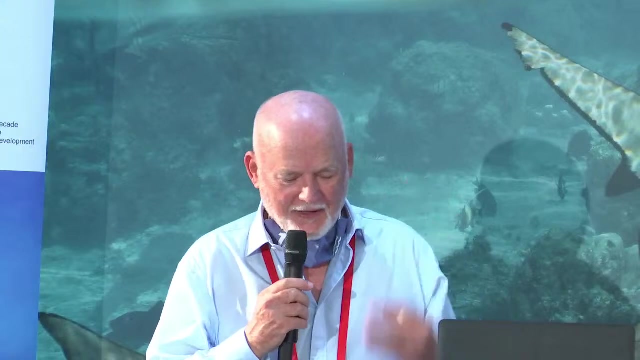 climate change and biodiversity loss. Where's the ocean in that? I didn't hear the ocean mentioned, And yet it's measurably, scientifically, measurably in decline. It's the ocean which supports us. Surely that is the third great challenge. 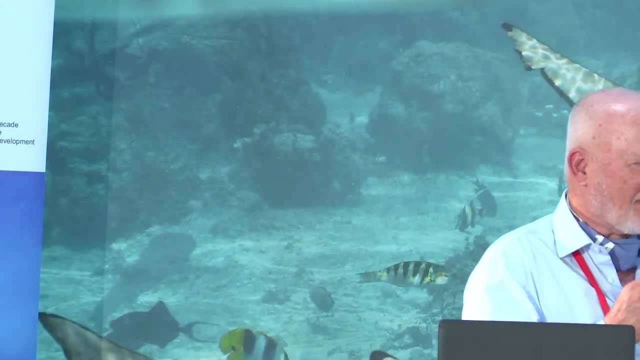 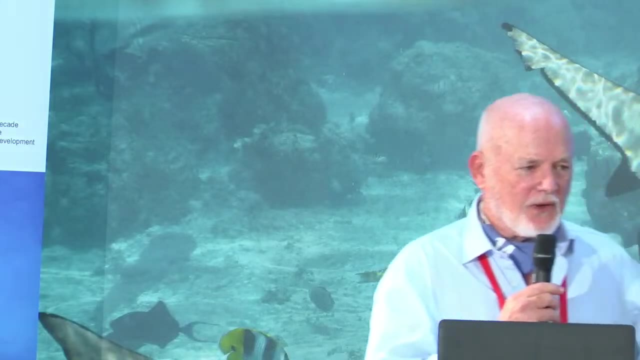 And if you look at climate change, what is climate? Climate is the interaction between the ocean and the atmosphere. Am I correct, Vladimir? That is what climate is. So how can you talk about climate change without talking about the ocean? You know, this is the driver of climate. 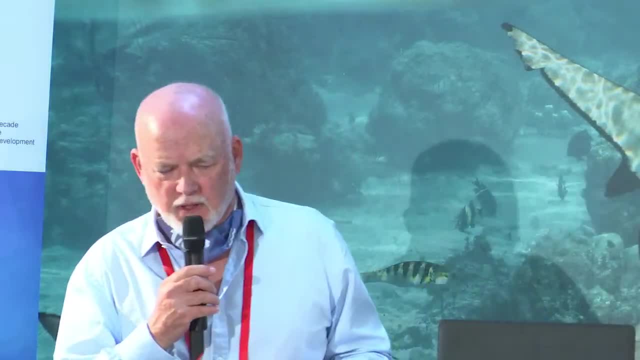 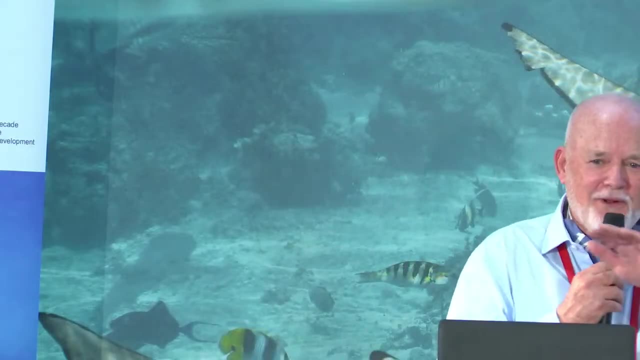 And, as I said, the ocean is in decline, Its health is in decline, measurably, scientifically measurable. And then you talk about biodiversity loss, where you know. look at all these terrestrial people you're surrounded by, you know terrestrials. 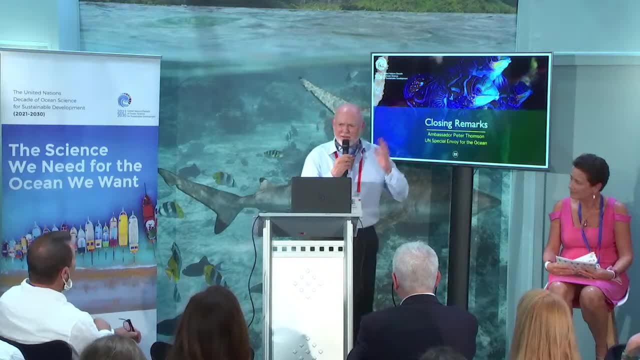 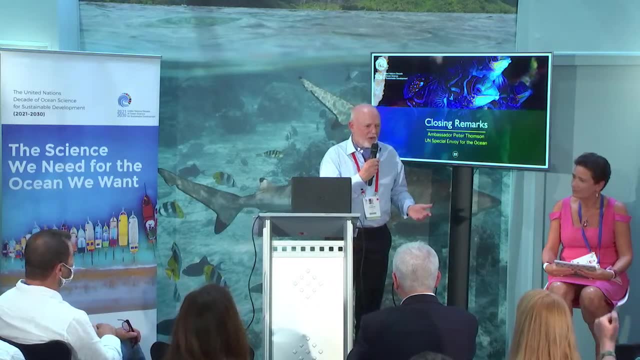 You know where is the great majority of life on this planet? 80 to 90%. I forget the figure, It's in the ocean. diversity, number of species: any way you want to measure it, it's all in the ocean. 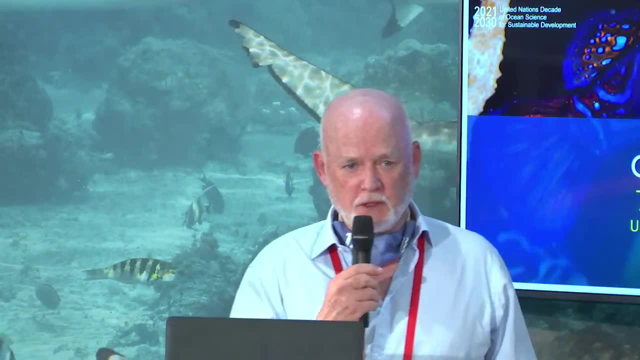 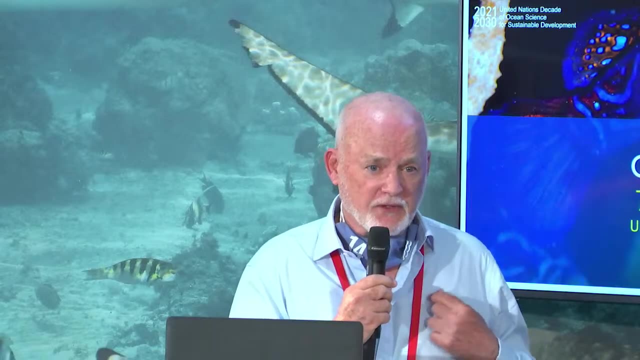 So that's why I never say the words our oceans. Firstly, you never say plural because the first principle of ocean is: there is one ocean and that matters to us in the South Pacific because the water coming off the Greenland ice sheet. 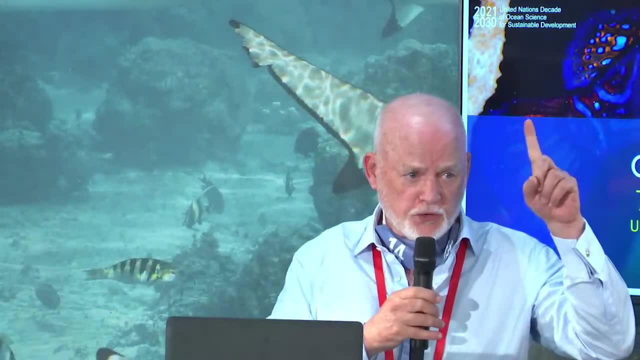 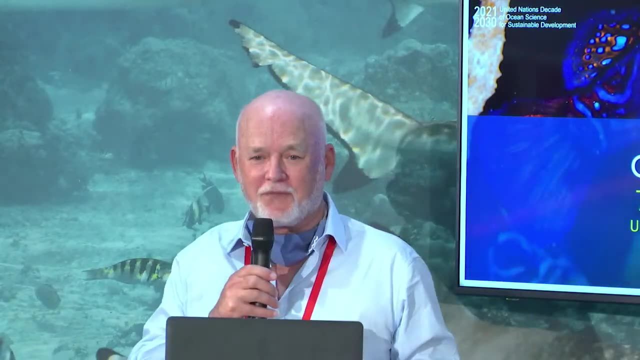 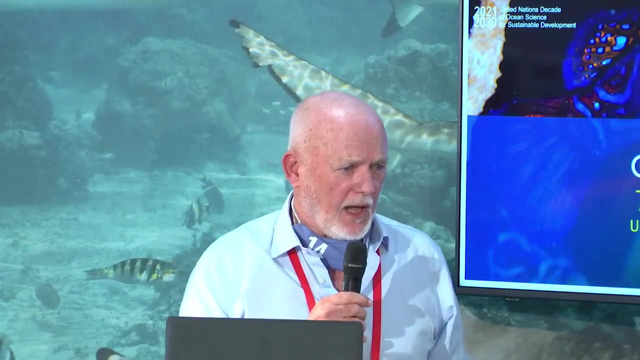 is sending up our sea levels here. it's one bathtub, So one ocean: the ocean. Thank you, President Macron, for the one ocean summit coming up very soon. fantastic leadership from the French president- And I never use the possessive our ocean, who says: 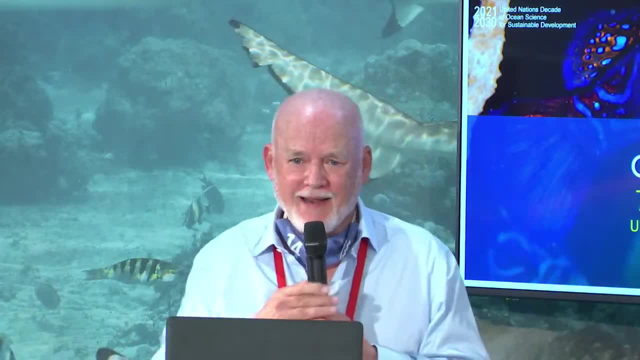 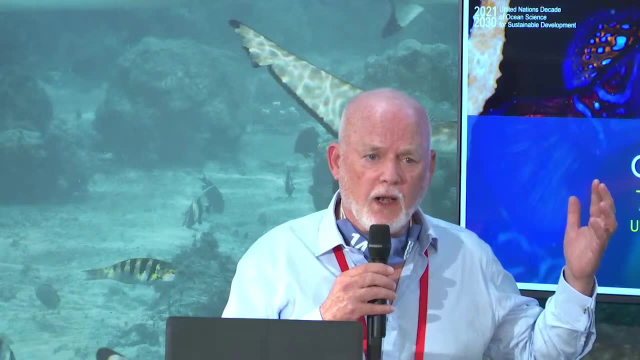 You know, when Homo sapiens has long gone from this planet, the ocean will still be there. It'll be a lot more acidic thanks to our efforts, but the ocean will still be there and there'll be a bunch of life creatures. 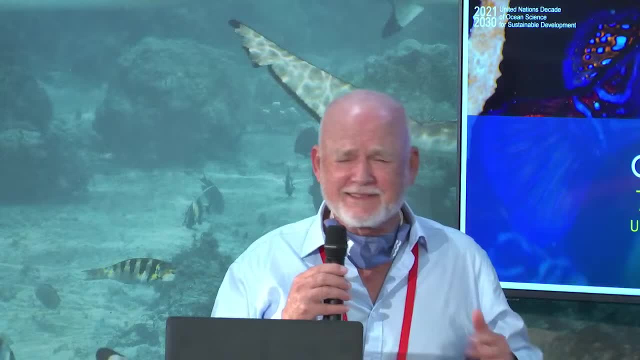 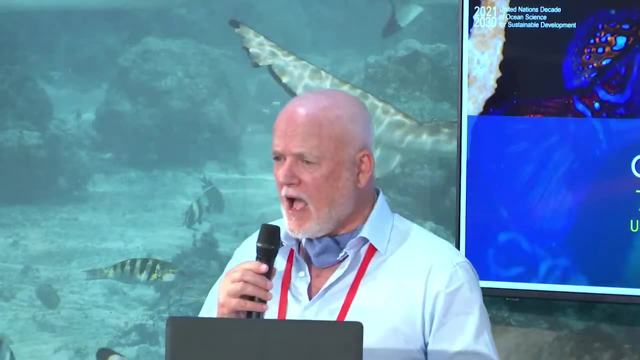 probably jellyfish or whatever. who'll be sitting on the beach with sunglasses and saying, hey, these guys used to call it their ocean. Yeah, the ocean is still here. So it's not our ocean, it's not our oceans, it's the ocean. 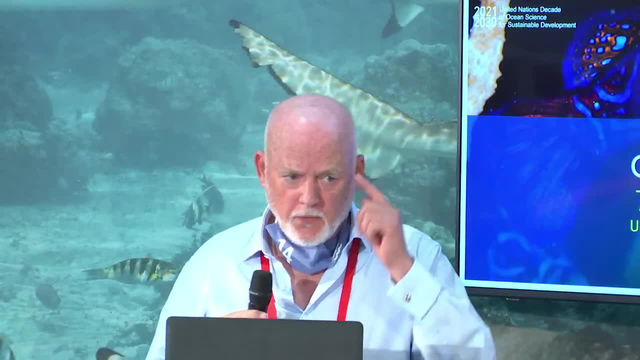 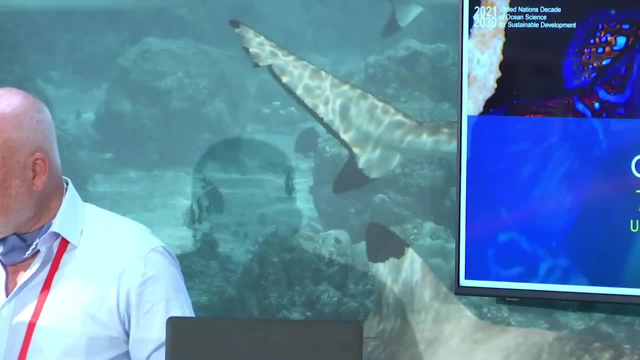 We belong to it. it doesn't belong to us. Very important, because when you get that in your head, a lot of things change in your thinking About life on this planet. So there's another thing we're cutting. now See, they're cutting me short and I've got a thousand things to tell you. 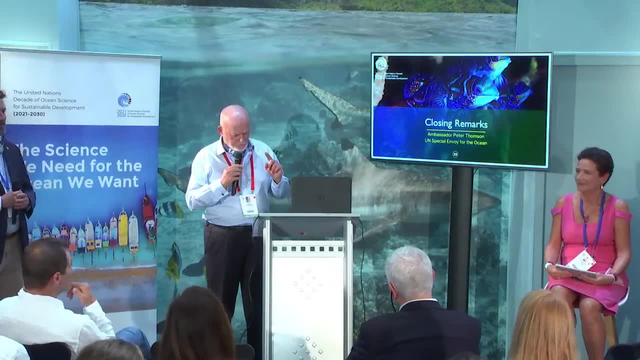 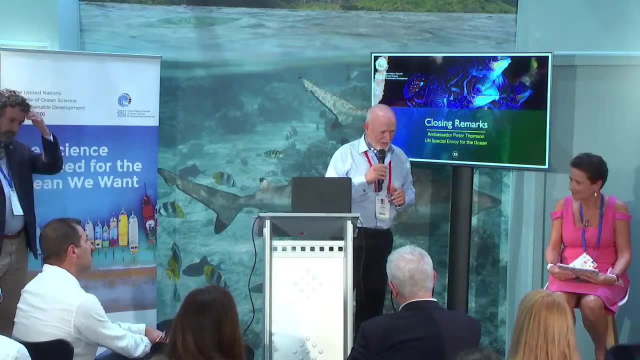 but I wanted to. okay, I'll give you one last thought then. Science planning, finance. This is what Peter Hogan, the former chairman of the IOC, and I and a couple of other people in Bergen. we sat down for a day brainstorming. 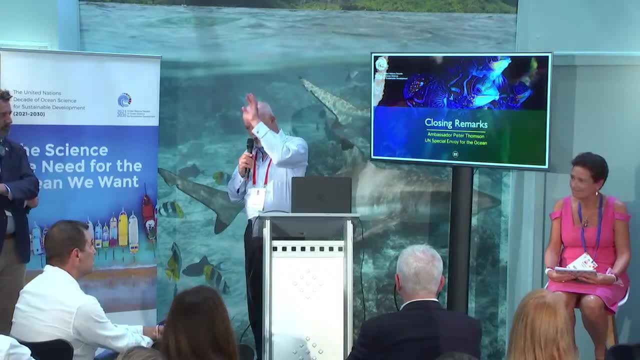 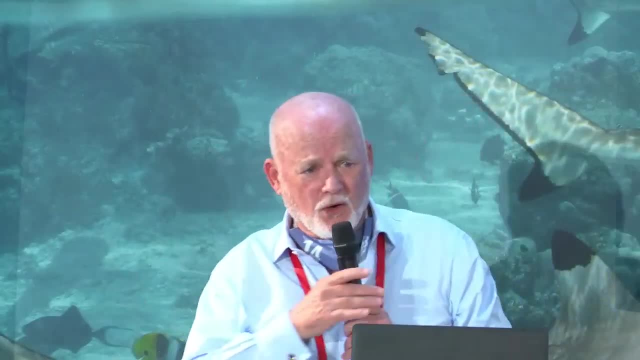 We came up with that mantra: science, planning and finance. What do you want? Everybody wants some money to put in their windmills in the sea to save their coral, to do their sustainable aquaculture, to make the shipping renewable energy, et cetera. right, 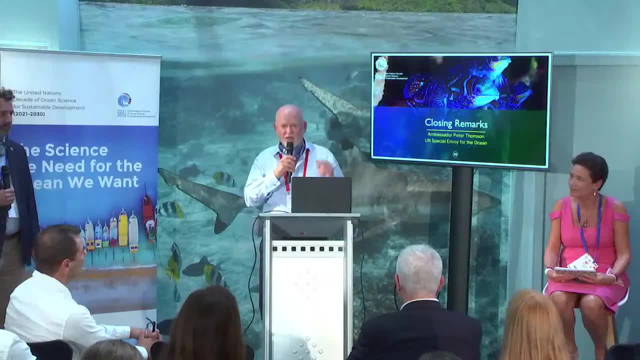 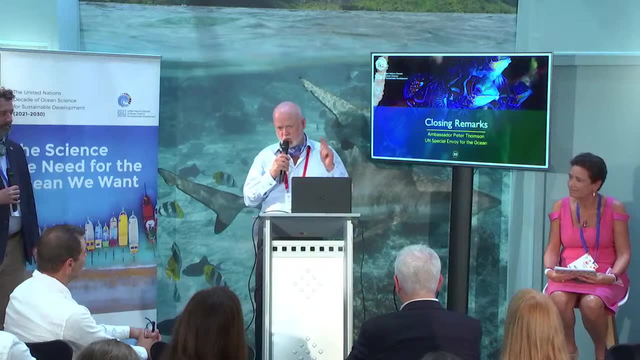 This all takes trillions, trillions of dollars. Great. that's where we need to spend our trillions. We know we can spend it- we've seen that in COVID- But before those funds will be freed up. to do that we have to have really good plans in place, really good plans. 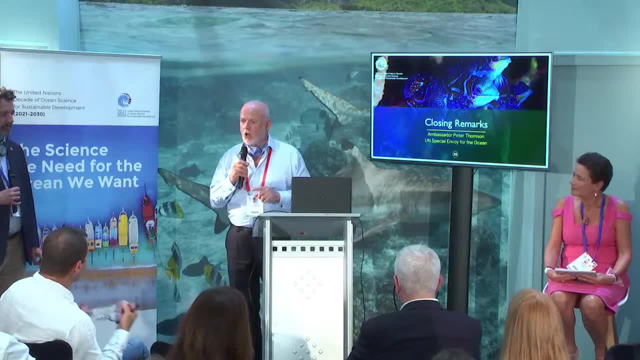 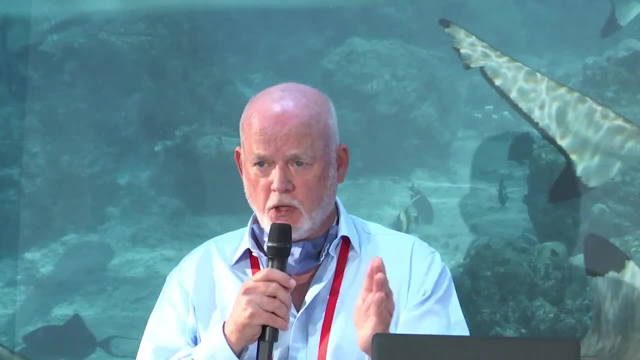 And that was the conclusion of a high-level panel for a sustainable ocean economy- that all of us, in all of our EEZs, have a responsibility to put in place sustainable ocean plans, And the 14 heads of government that are in the panel have agreed to do that by 2025,. 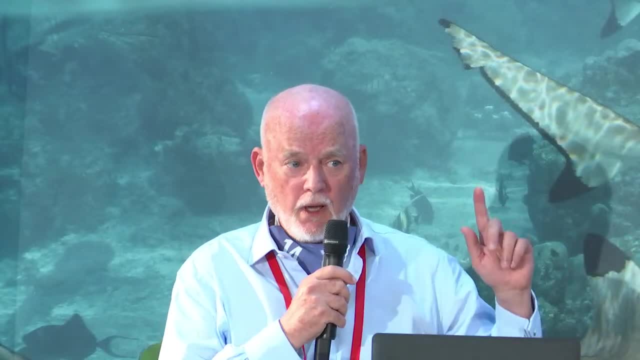 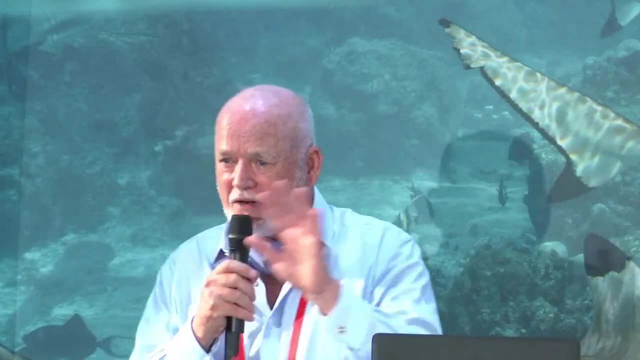 and they've asked all their peers, all the other heads of government, to do it by 2030. Why? Because without it, nobody's going to give you money if you haven't got a decent plan in place And you've got to do it all, obviously, environmentally correctly. 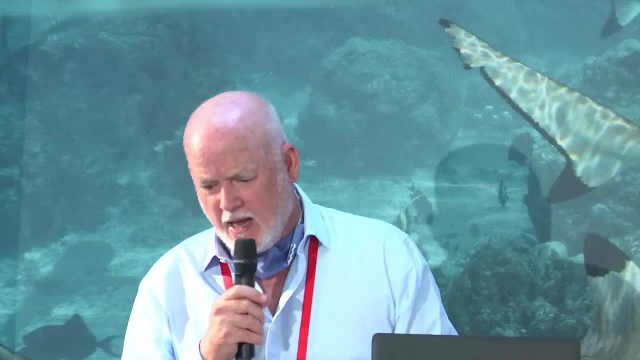 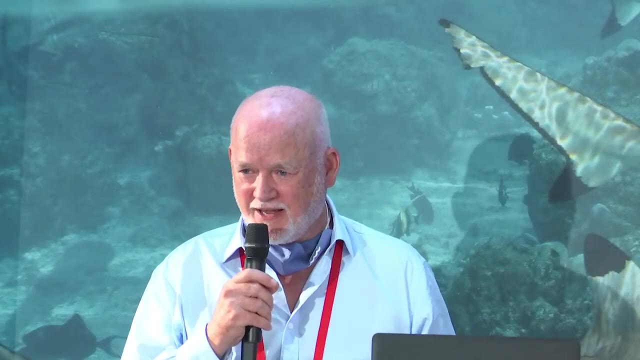 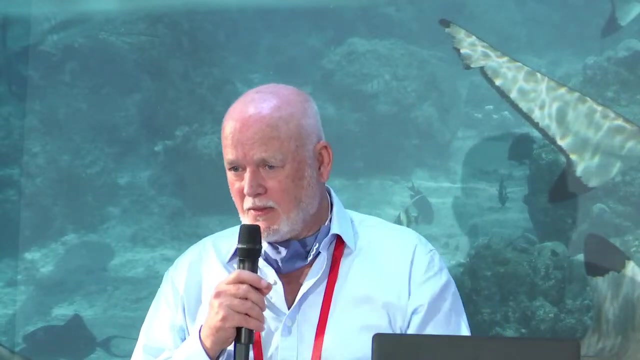 and where the MPAs go, where the wind farms go, et cetera. The first part of the mantra, though, is science. We have to invest in good ocean science in order to have the right plans in place, So science planning and the projects that come from that, 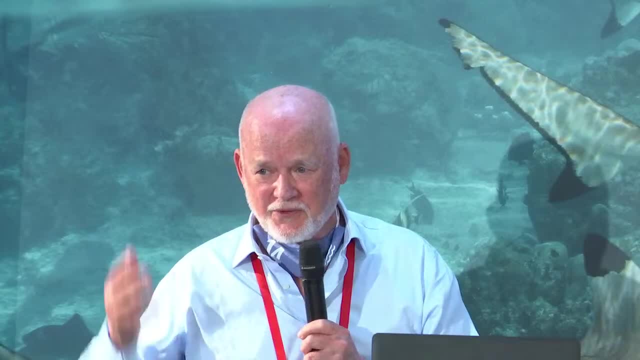 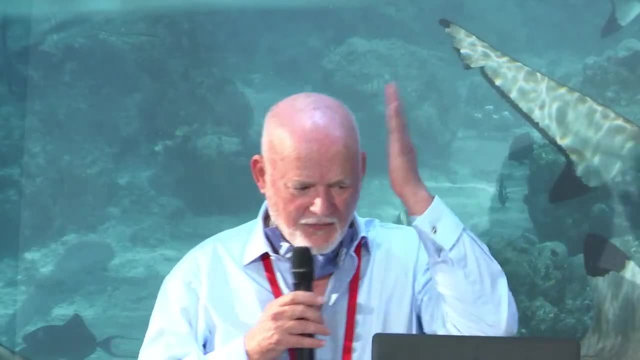 That's the mantra. that's where the money needs to go. I've got meetings with Green Climate Fund, with Jeff. I've just met with Nora- Anybody who's got the money to put in think of science, planning, finance.